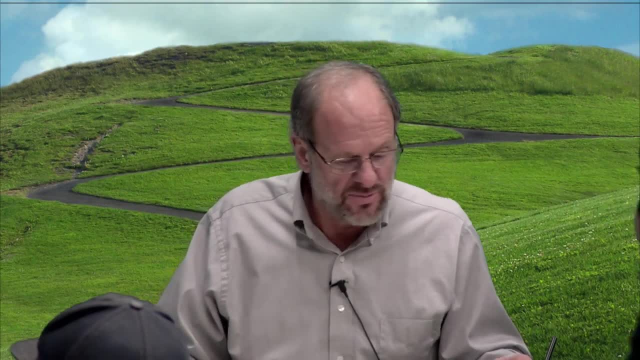 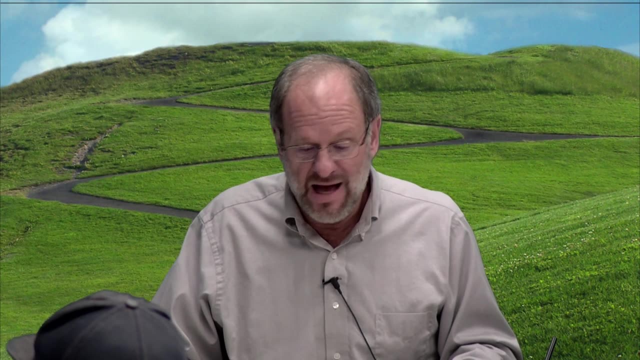 We can use graphs like the compressibility chart, But ultimately we have to have two properties, two independent intensive properties, in order to find all the others. A lot of what we've been talking about these first few weeks is just trying to figure out what all this data means. 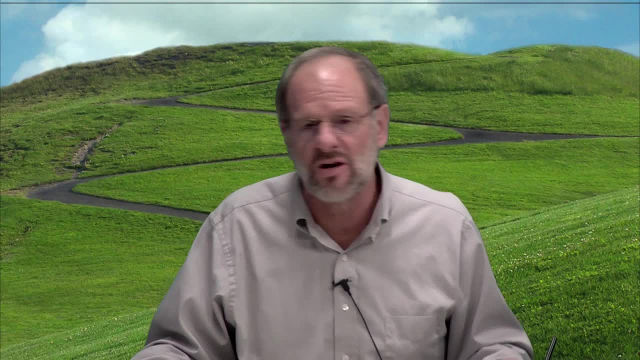 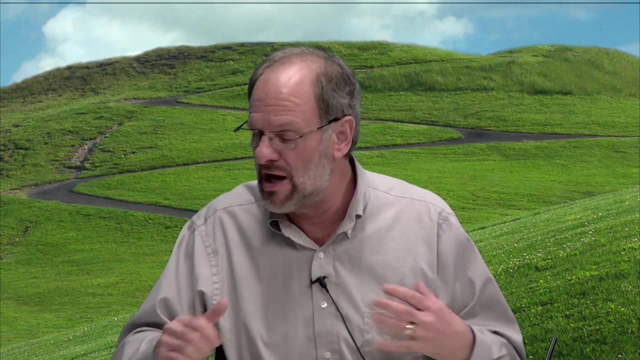 Where does it come from, How do we utilize it, How do we know which table to go to, et cetera, et cetera. We're behind that now. Now we started to look at the first law. The first law basically tells us that the energy difference. 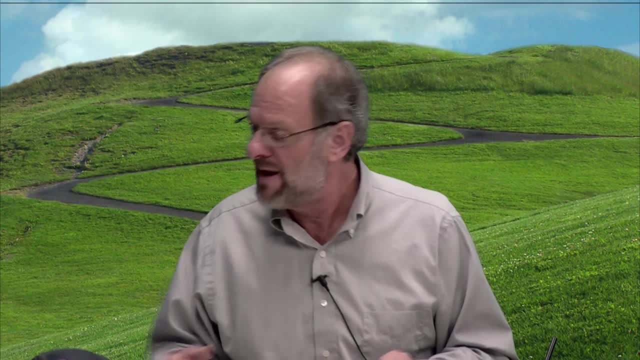 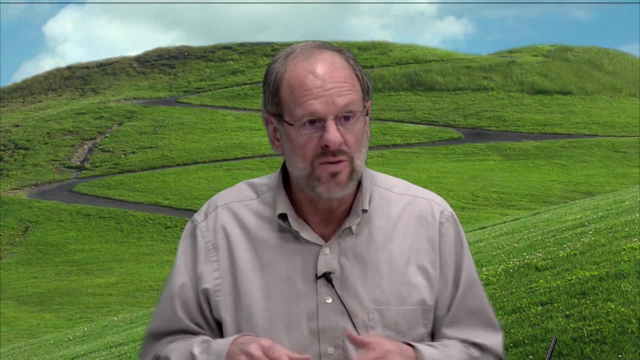 between what flows into and out of the system equals the energy change of the system And, as we saw this last time, basically this tells me that the heat transfer is equal to the change in the energy plus the work right. The change in the energy is the sum. 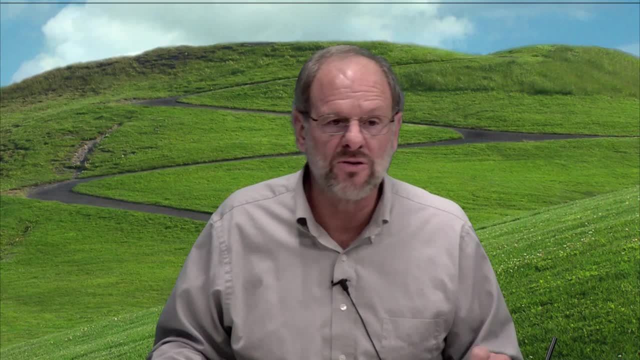 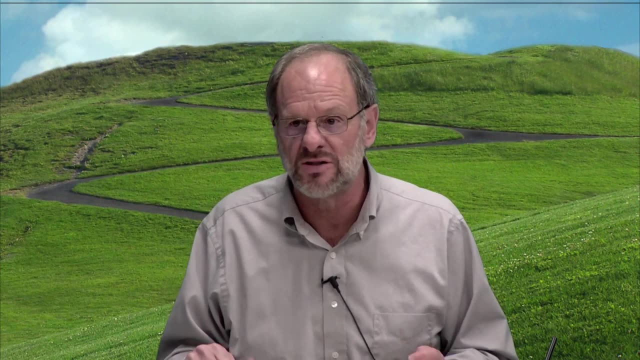 of the internal energy plus kinetic energy, plus potential energy. So we have a first law equation that we're going to solve And in fact we have several forms of the first law equation. Some are written in terms of total values, like the total amount of heat or the total amount of work. 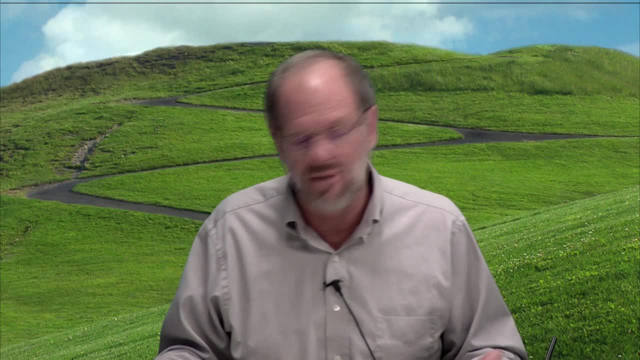 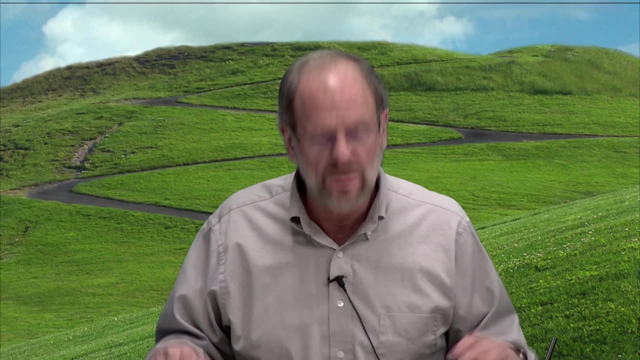 Others are written on a rate basis. Other equations can be written on a per unit mass basis, But all of this is written on a rate basis. All those equations we saw last time are just different forms of the first law. Now we're only dealing with closed systems. now 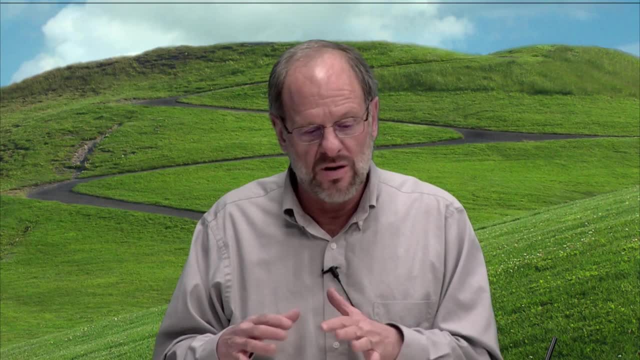 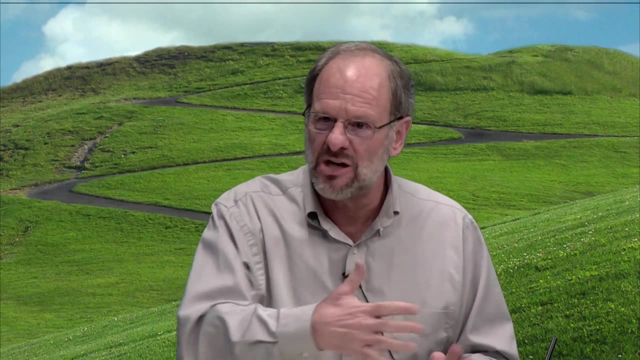 In other words, we have a fixed mass and we're now beginning to look at real problems involving such systems. So at the end last time we talked about problem-solving techniques And you know I'm going to try my best to use those techniques. 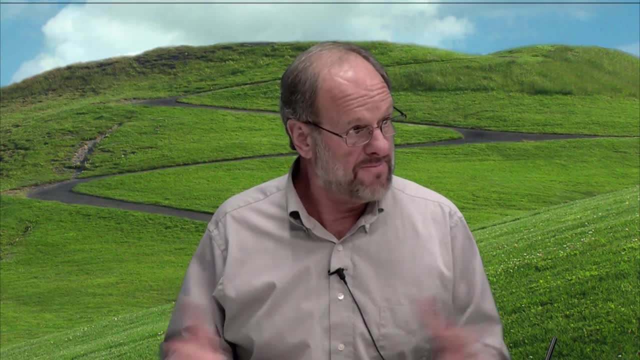 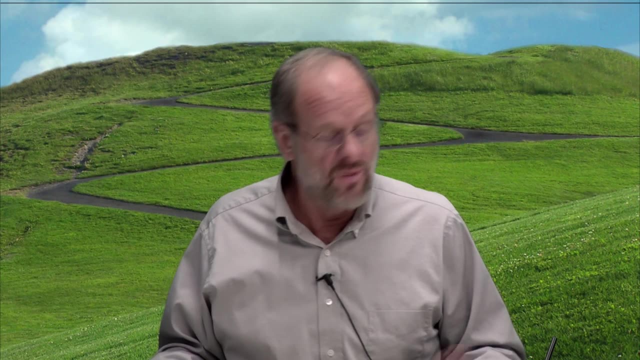 when solving problems. But now what we need to do is we need to bring it all together. Okay, We need to look at a written problem like the one I'm going to show you. I'm going to work on here- And we have to know what equations to use. 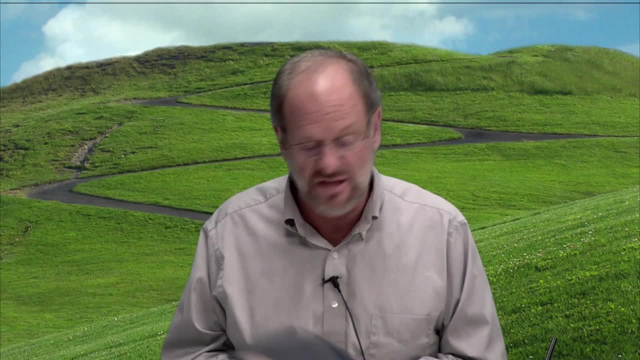 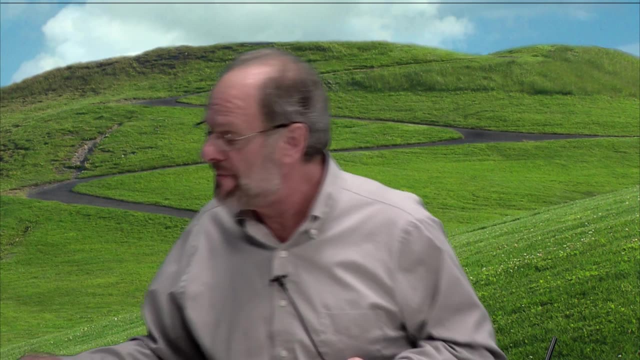 We have to know where the data comes from, We have to be mindful of units, et cetera, and eventually come to the solution. So, in this particular problem- and this is the first one we're going to do today out of many- 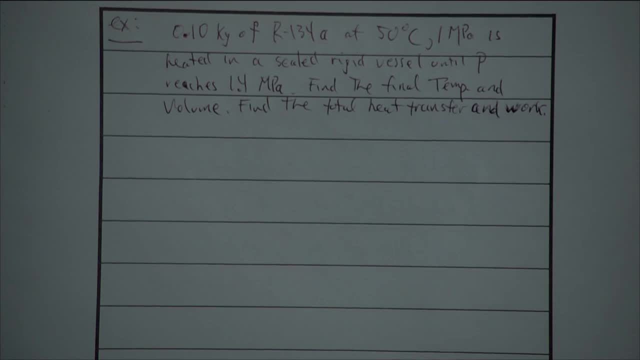 we have the following. So let's assume that we have a tenth of a kilogram of the refrigerant 134A and it exists at 50 Celsius, 1 megapascal, And we know that it's now being heated up inside a sealed, rigid vessel. 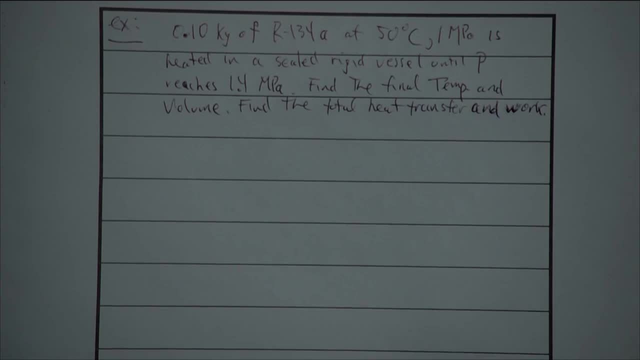 Okay, So we're going to do that. Now, when it says sealed rigid vessel, that means a tank. right, I could use the word container, I could use the word tank. I could use the word sealed, can I mean? there's a lot of things I could use. 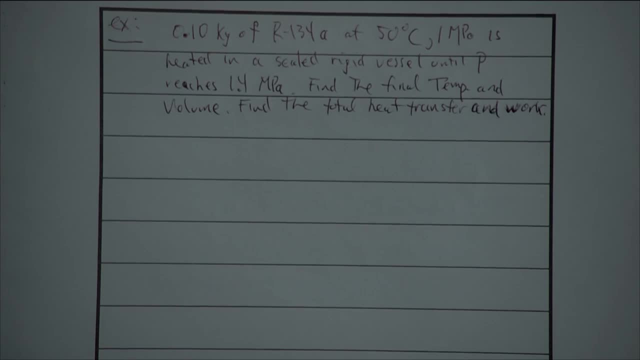 But we understand that we have a sealed container, So there's a fixed mass of material And we're adding heat until the pressure reaches 1.4 megapascal. All right, So that's the end. At the beginning we know the temperature of the pressure. 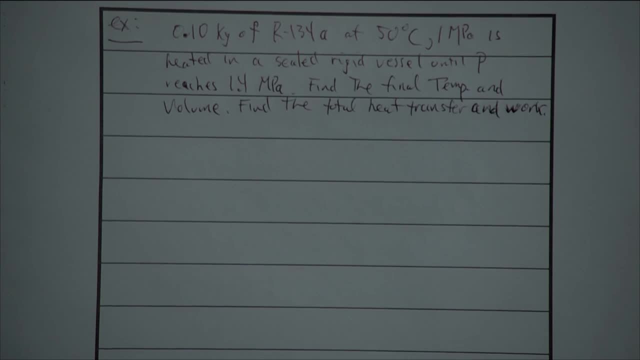 At the end, we only know the pressure, But what we're trying to do, then, is find some other conditions at the final state point. Right, We're trying to find the final temperature as well as the volume. We're also trying to find the total heat transfer and the work. 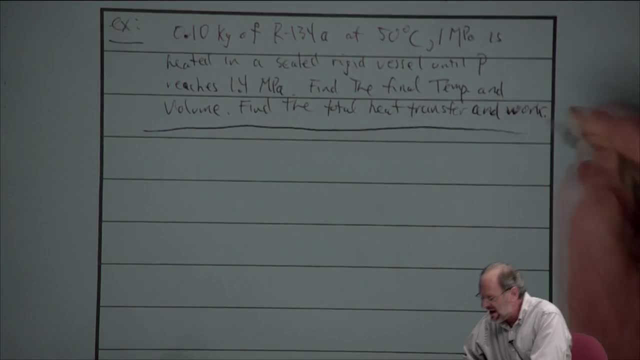 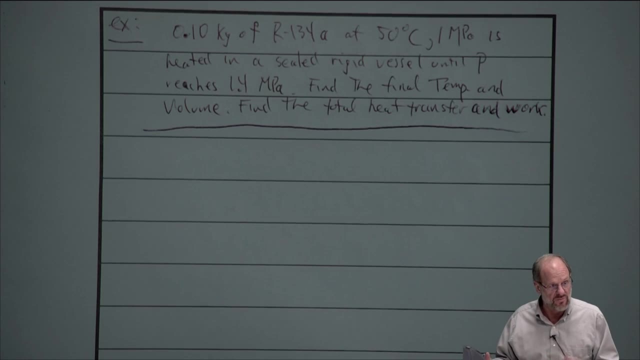 So this is where we're headed in this particular problem. Now, as I start a problem like this- and I would suggest you do something similar- the first thing you want to do is state the problem Now. I mentioned this last time. 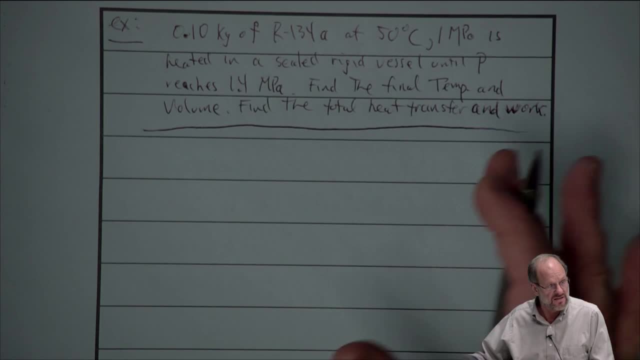 You can just cut and paste from the book, or you can rewrite it identically, or you can rewrite it kind of paraphrasing. But you need to write the problem in a way that makes sense to you. I'm not going to bother to rewrite it here. 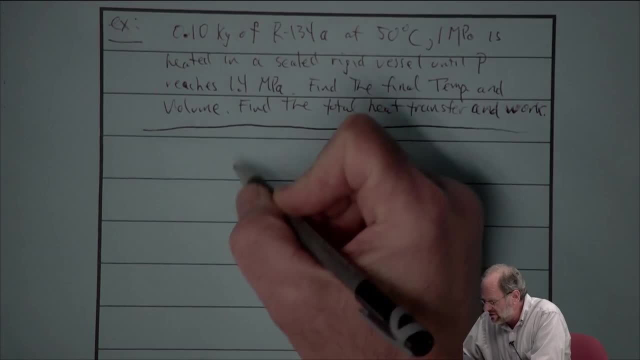 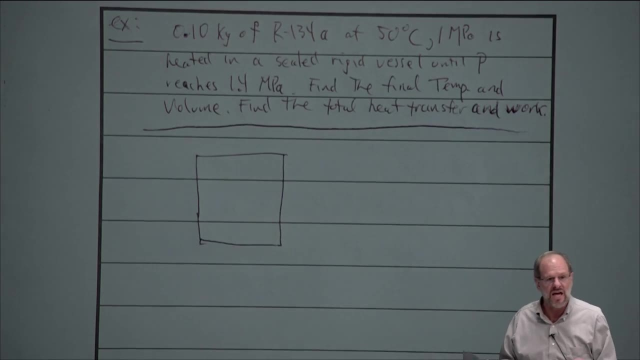 because I already have it written. But what I would do then is I would always start with some sort of a diagram and then identify as much as I can. So since it's a sealed rigid tank, I'll just show it as a big rectangle. 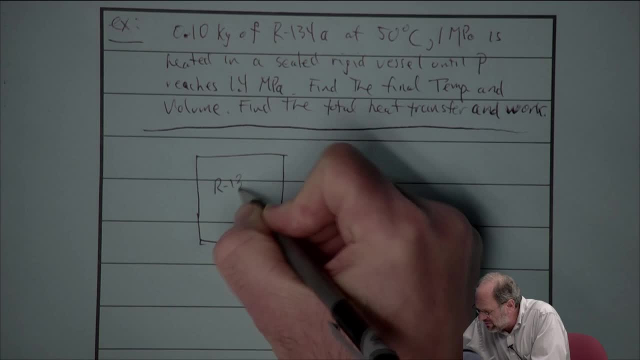 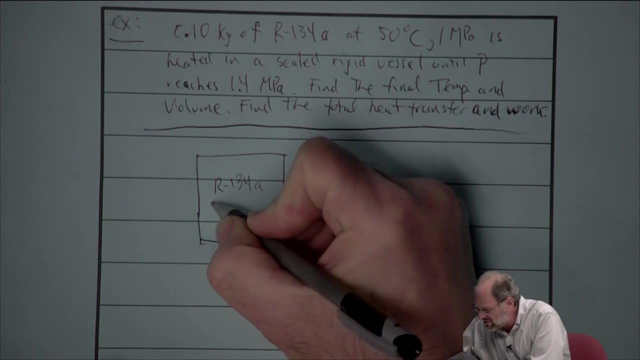 And we know that we've got the refrigerant 134A as the substance that we're analyzing. So I'm just going to write that on the inside. I'm also going to show the mass And even though this is all information that's given, 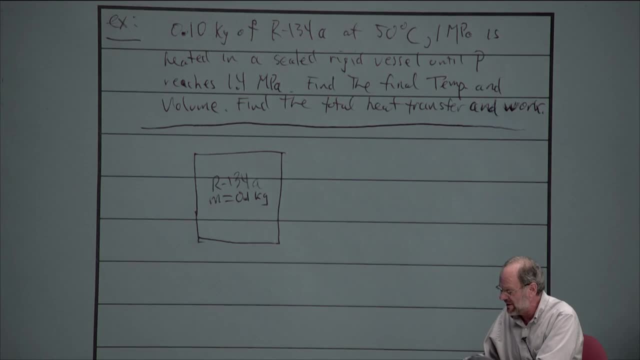 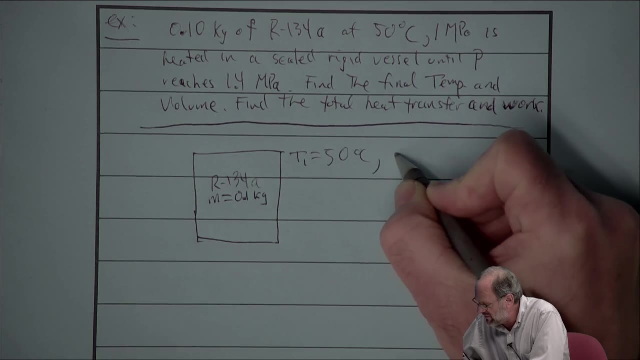 in the problem statement. I still like to rewrite this so that everything is right there in front of me. I also understand the initial as well as at least one final property, So I'll write: T1 is 50 Celsius, P1 is 1 megapascal. 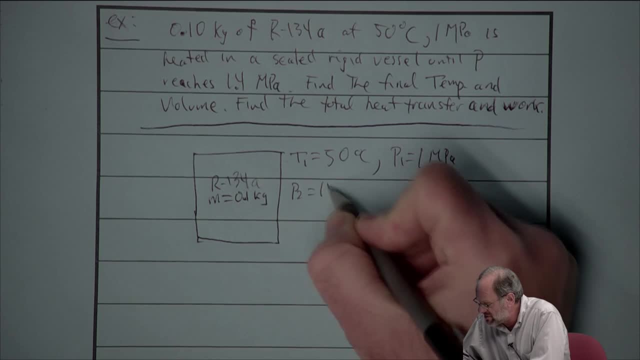 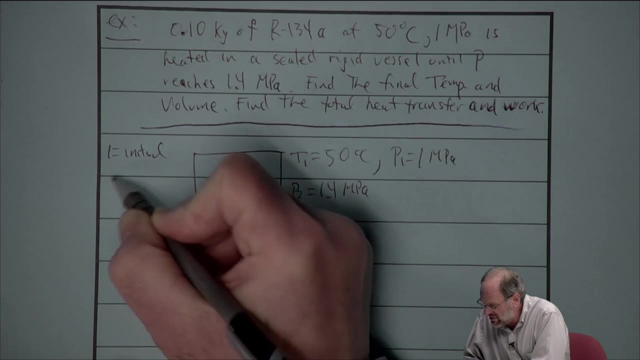 I'm also going to note that P2, which is the final pressure, is 1.4 megapascal. If it helps, you can just write: 1 equals initial, 2 equals final. just to remind you, we're talking about an initial. 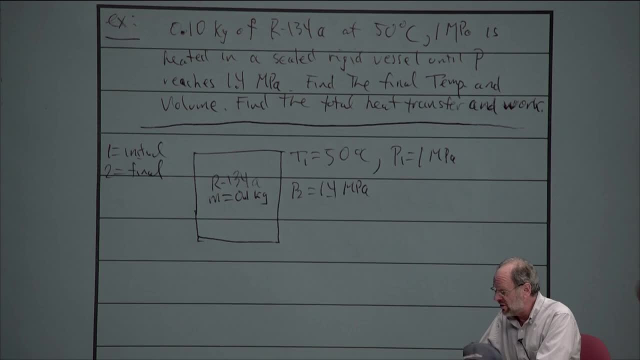 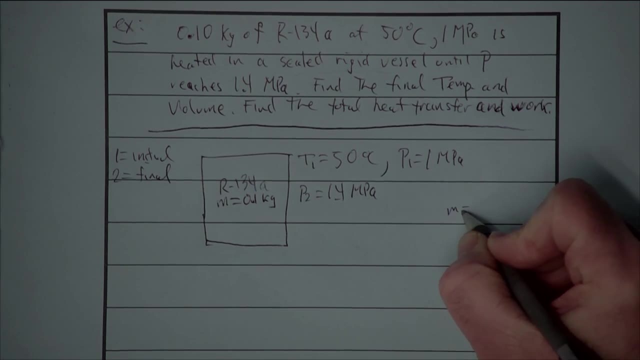 and a final state associated with this problem. Now you're also told it's a sealed, rigid vessel. So that actually tells you something too right. I mean first of all that the mass is constant. I mean that should be very obvious. 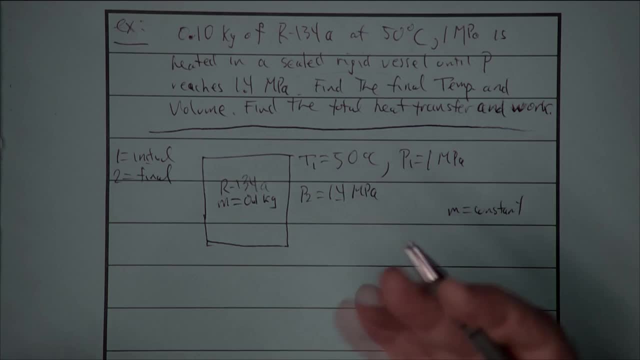 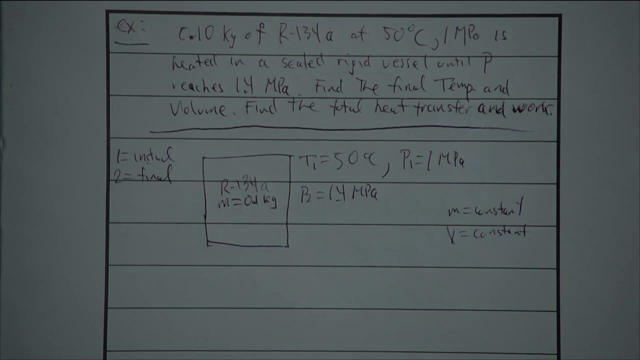 But also that the volume is constant. right, It's a rigid container. So if the volume is constant and the mass is constant, then we know that volume over mass is just a specific volume, right? So does that mean the specific volume is also constant? 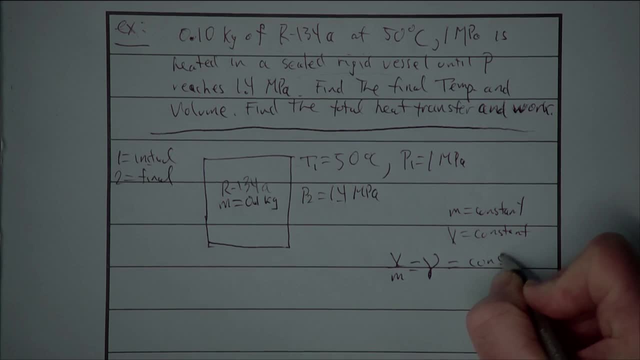 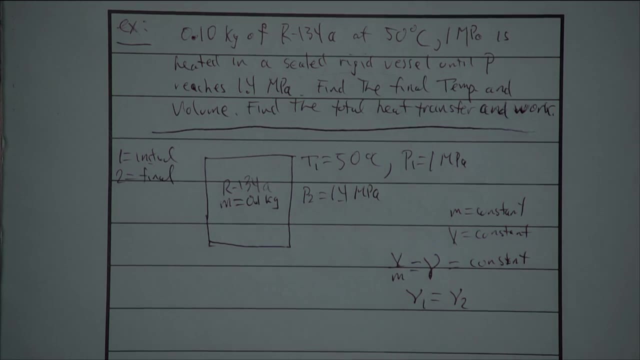 So you'll then say that the specific volume is constant, Or another way of writing, that is simply that V1 equals to V2.. So these are things that we know about the problem. Now, what about things we don't know about the problem? 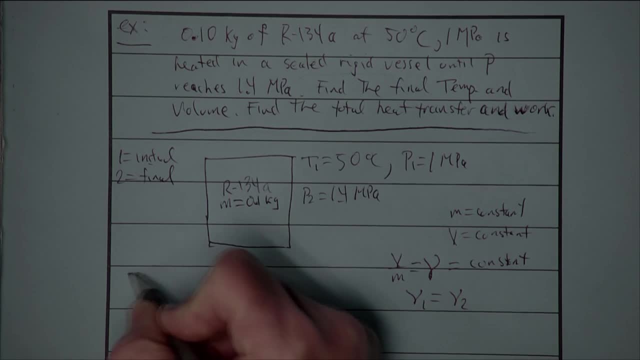 that we're interested in. Well, I certainly want to know what the final temperature is. I need T2.. I need to know V2.. So V2 is unknown, Although we've stated above that V2 is the same as V1.. 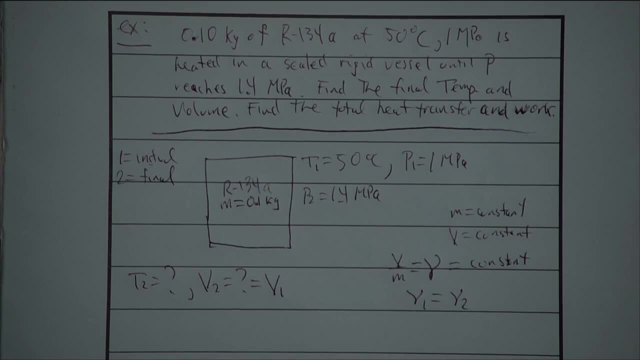 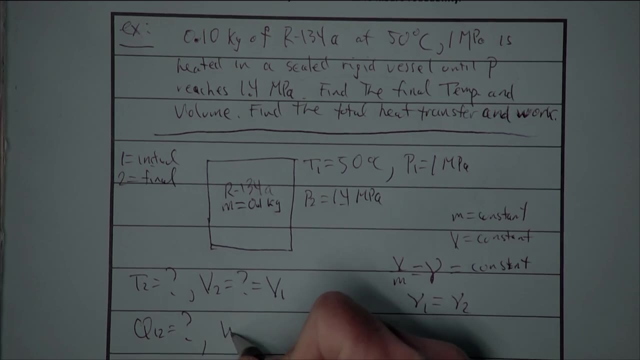 So you could also just show that V2 is unknown but it's equal to V1.. We're also trying to find the heat transfer for this process, So Q12 is unknown. We're trying to find the work, So work 12 is unknown. 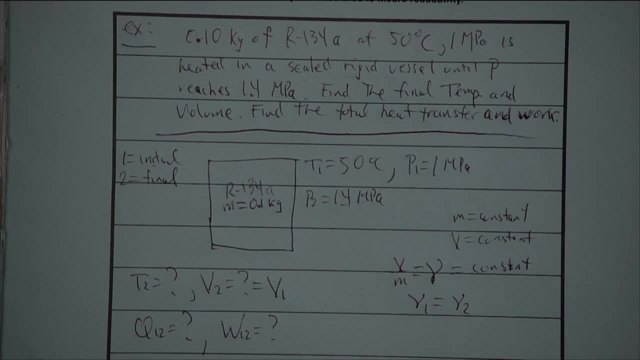 So these are all the things that are known and unknown to me. okay, So I've identified a lot of the information. I've also shown that this is a constant volume process. right, Specific volume is constant. Total volume is constant. It certainly is a constant volume process. 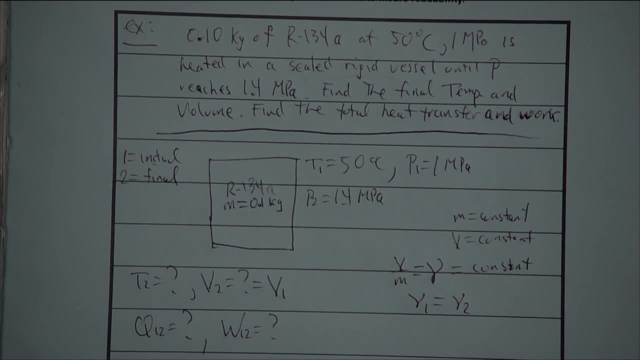 We know that about it. So I've really kind of completed the first two steps of this seven-step discussion from last time right. I've identified my knowns, I've identified my unknowns, I've created a sketch, I've identified the problem. 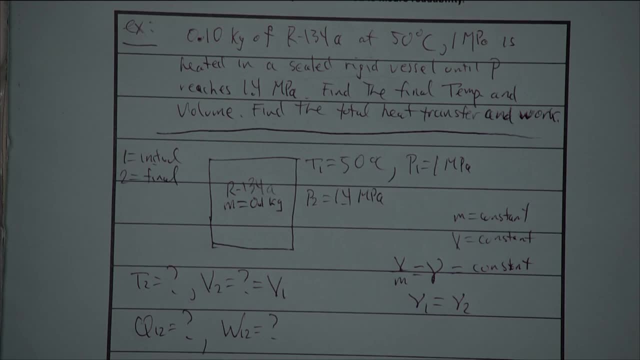 I've identified any process. I've identified all the processes that are involved, That is, it is a constant volume process. I've identified the substance. So there's not much more I can really do. I've shown a schematic diagram. What about some assumptions? 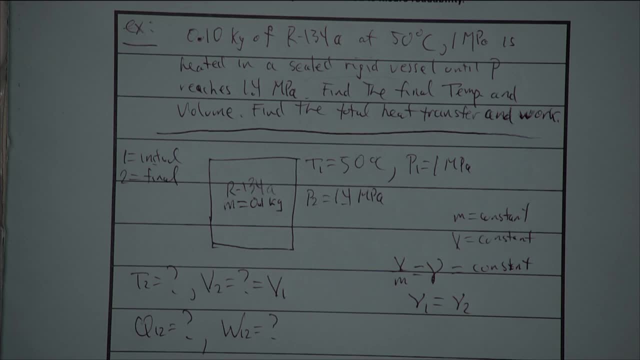 Is there anything we can assume that's going to be important in this problem? Well sure, It's a sealed, rigid tank. There's no motion associated with it, So there's no kinetic energy change, right? So we can assume that. 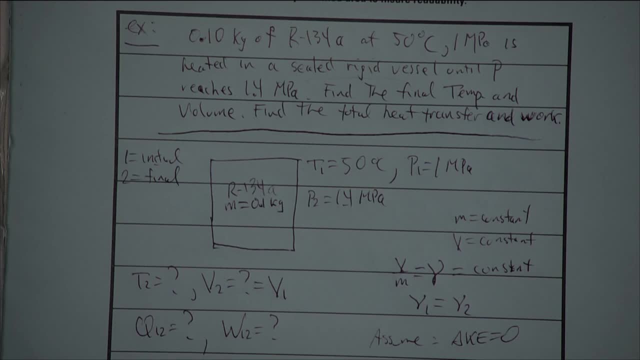 There's no change in kinetic energy, since there's no motion either at the beginning or at the end of the process, And we can also note that there's no change in potential energy right. There's no height change associated with this thing. 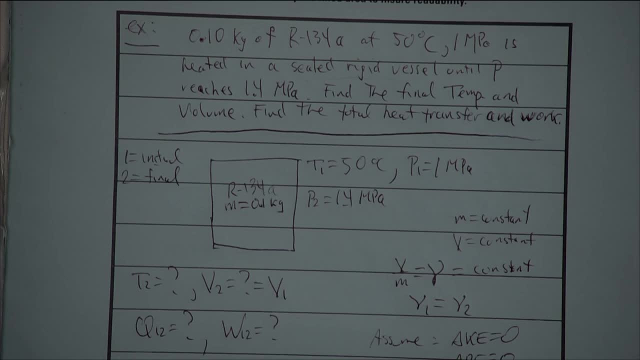 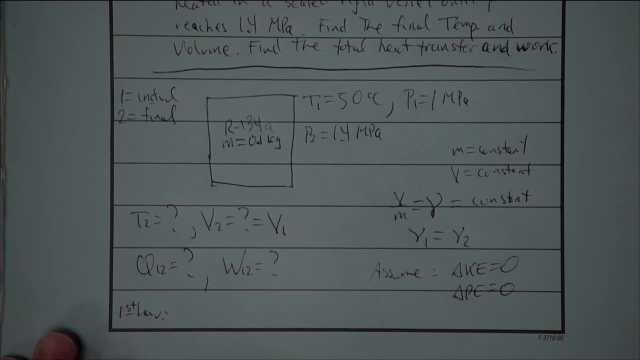 We start at one elevation, We end at the same elevation, So there's no change in potential energy. All right. So now, if we continue, we know this is going to be a first law problem because, frankly, they're all first law problems. 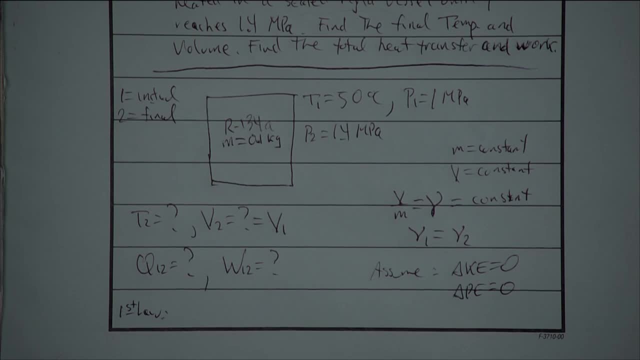 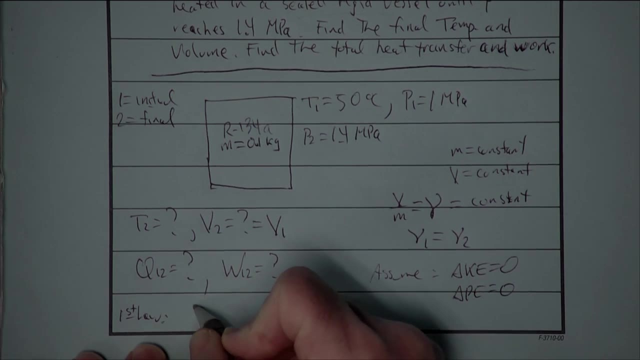 And the equation Which we want would be the one that includes the total work and total heat transfer. So I think I called it equation E in your notes from last time. So basically, the heat transfer is going to equal the change in internal energy plus the change in kinetic energy, plus a. 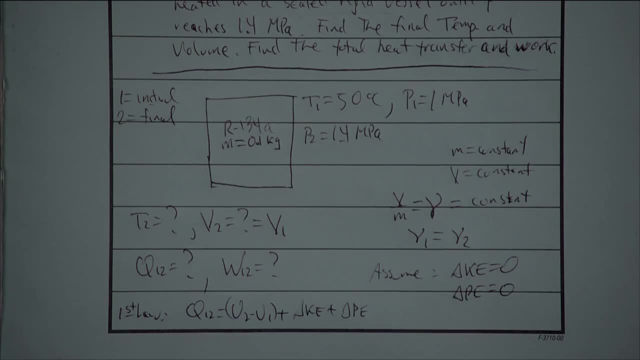 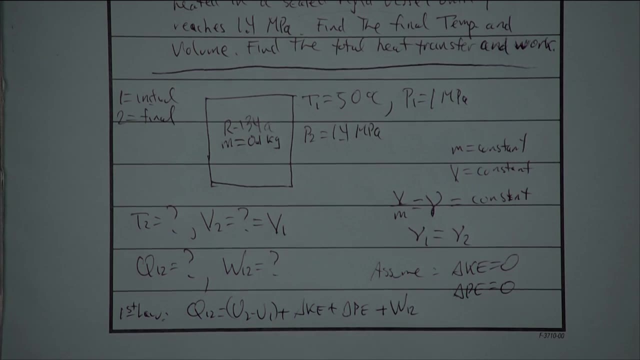 change in potential energy. I'm not going to write out the actual equations. I know they're zero And then plus the work that's done. Now, what about the work That should be zero too right, There's no other forms of work. 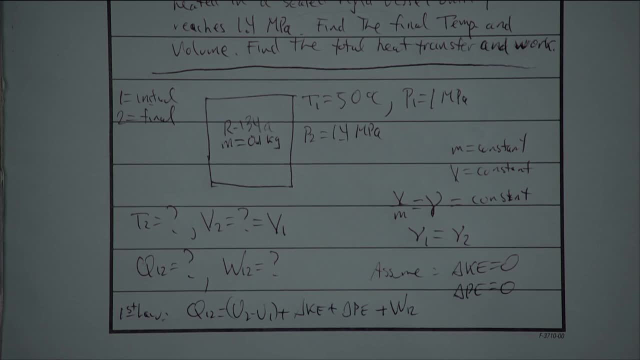 There's no bent wires, There's no springs, There's no electric resistance heaters, There's also no boundary work, right? So I could assume that there's no work, or I could just simply note that, since there's no volume change and no other forms of work, that there is no work. 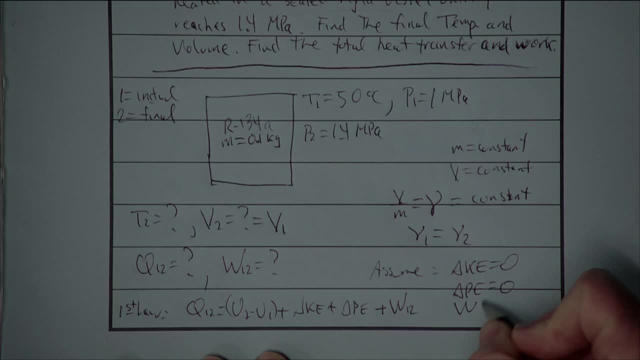 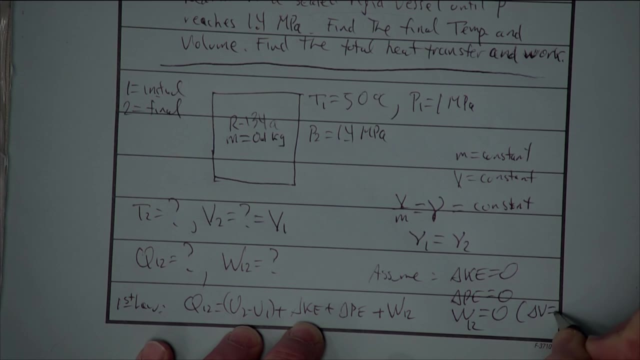 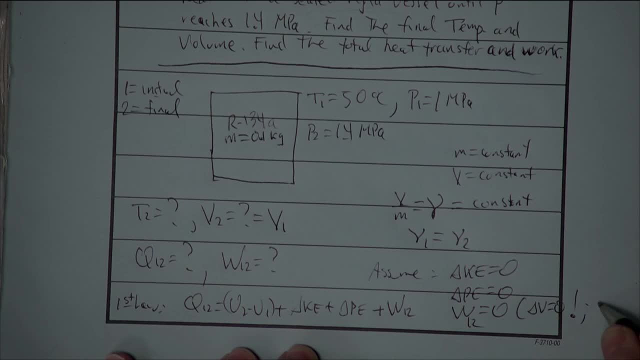 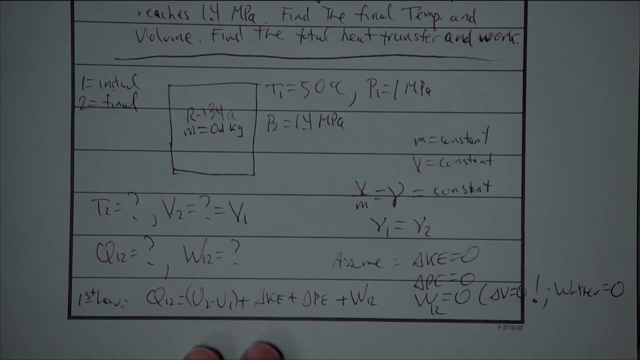 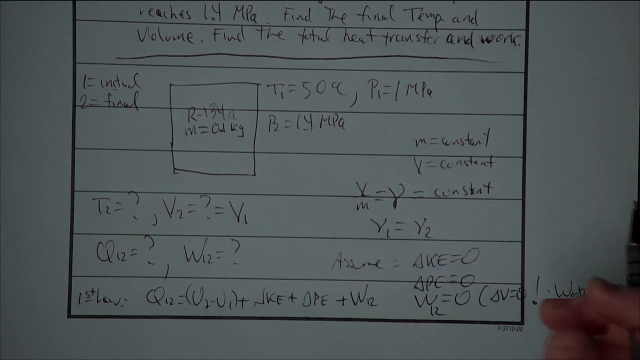 With no volume change, there can't be any work And there's also no other forms of work. Okay, So there's also no other forms of work. Well, so here's our first law. Let's get rid of what we have already said is zero. 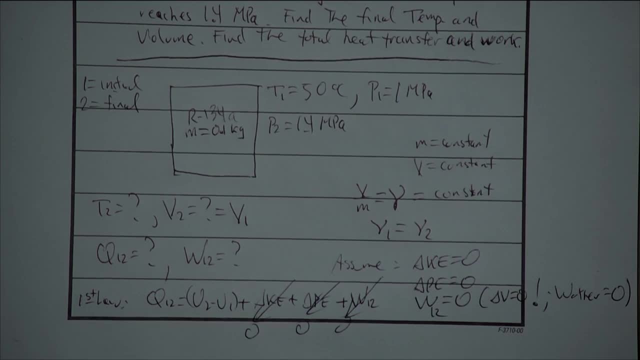 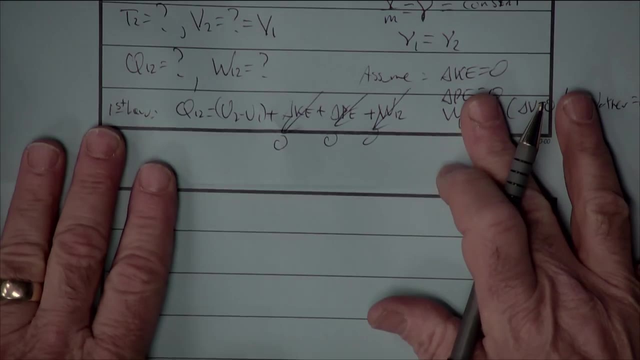 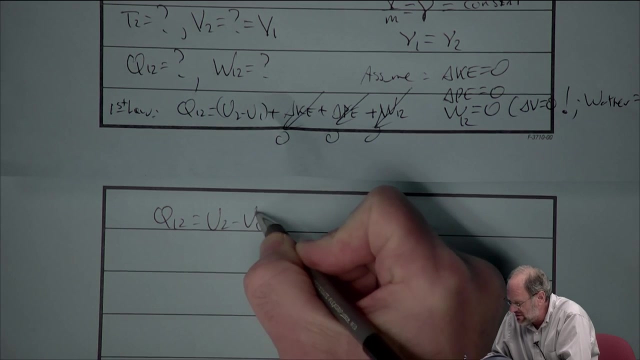 So there's no kinetic energy, There's no potential energy, There's no work. So in order for me to solve this problem, at least to find the heat transfer, I just have to solve the equation that says that the heat transfer is equal to the change in internal energy. 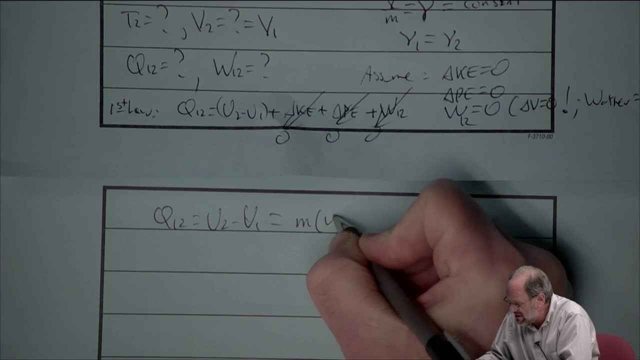 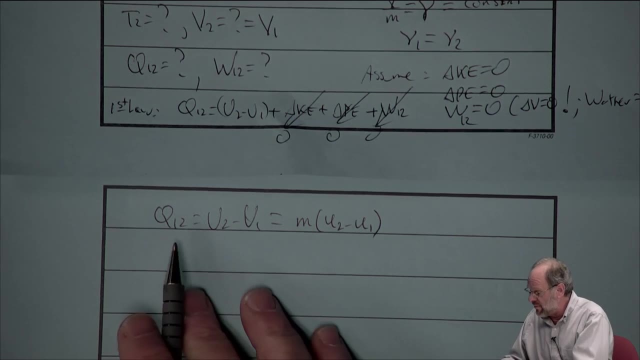 And let's also recall that the change in internal energy is just the mass times the change in the specific internal energy. All right, So we can solve this problem, And always. you know, all we need to do to solve this problem is figure. 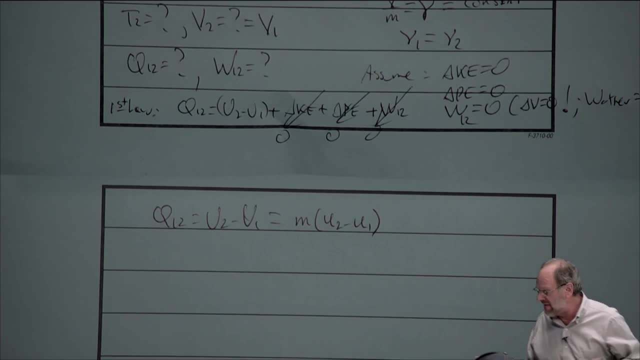 out what u1 is, figure out what u2 is and figure out what the mass is. So now we have to ask ourselves a little bit more: Do we have any other information that's going to help me solve the problem? Because, quite frankly, I don't know the mass. 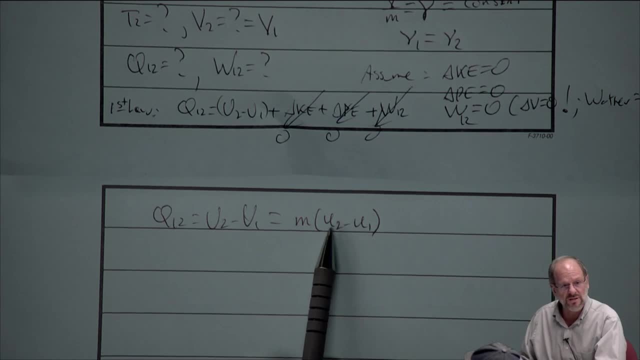 I'm sorry. I do know the mass but quite frankly, I don't know the final thermodynamic state. Can I find the final thermodynamic state? Do I have any information anywhere which allows me to find the second unknown, the second property at state 0.2?? 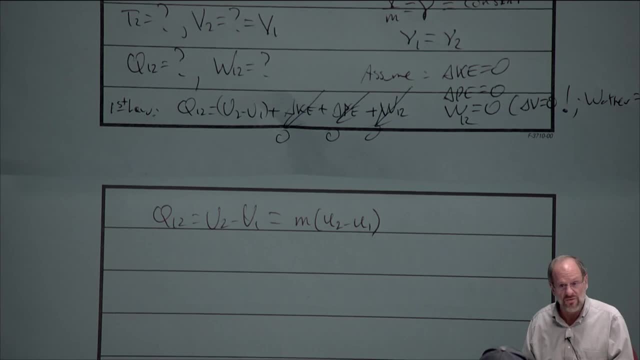 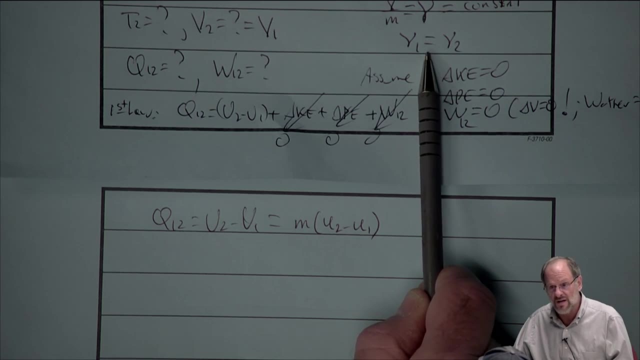 Again, it has to be an intensive property. Well, the answer is already there for you, right? V1 is equal to V2.. Whenever you have a sealed rigid vessel, the specific volumes are constant, And that's what's going to give you the second property. 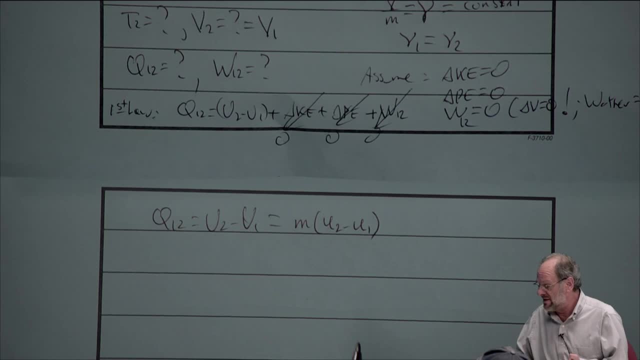 at state 0.2, so that we can then find every other property, including the internal energy. So, if you think about it, I know two properties at state 0.1, so I can go into the tables and very easily find u1.. 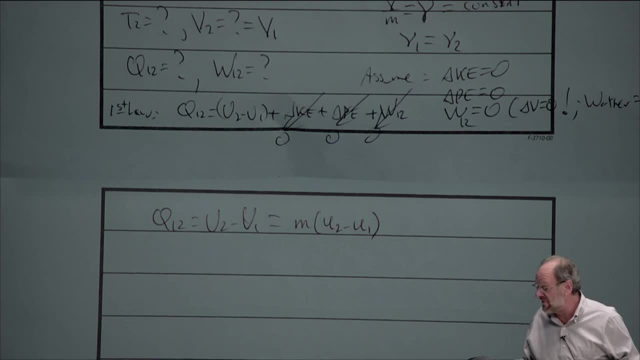 I can find anything else I want. I can find the specific volume at 1.. I can multiply that by the mass to get the total volume at 1, which is one of those things I need, right, So I can get everything I need at 0.1. 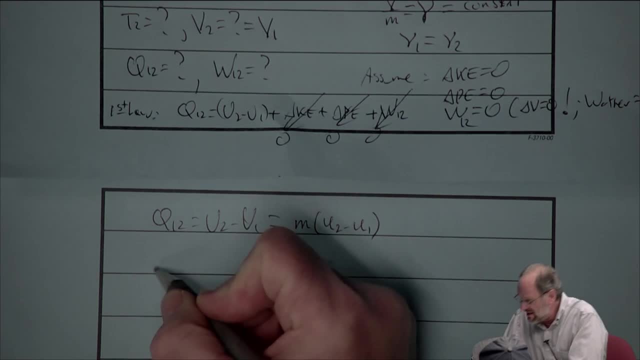 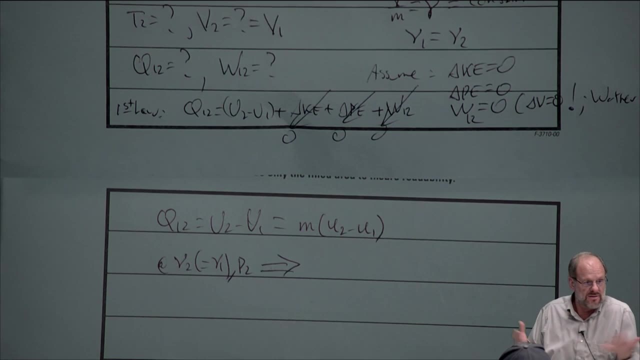 And then the same thing at state 0.2.. Since I know the specific volume at 2,, which equals V1, and I know the pressure at 2,, well, I can, you know, recognize that those are both intensive properties. 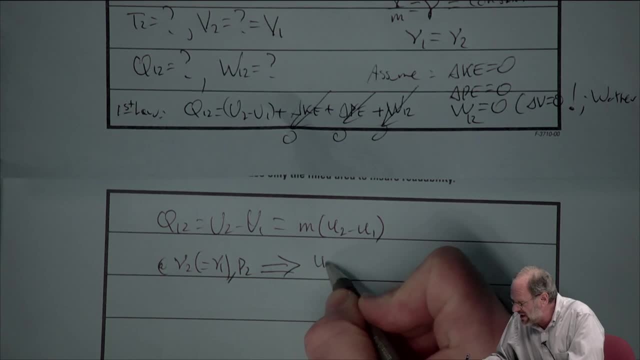 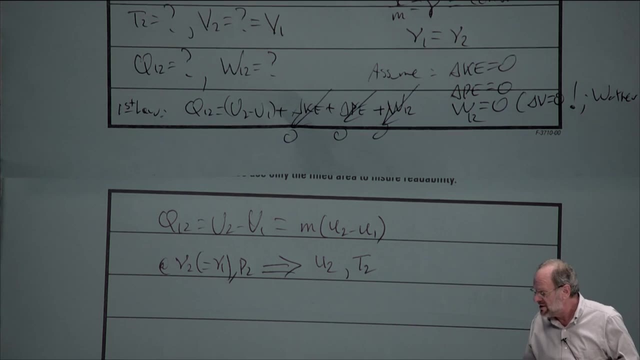 so I can go back into my tables and I can look up anything else I want. Now, certainly I'm going to need u2, but the book also asked me. well, the problem statement also asked me- to find t2.. So it turns out we really have everything we need, right. 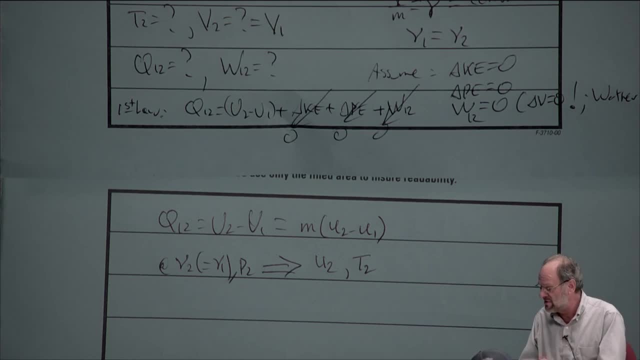 We have enough information to know state 0.1.. We have enough information to find state 0.2.. It's really just a matter of throwing everything back into the equations and then solving right. So now we want to ask ourselves: well, okay, we've gone. 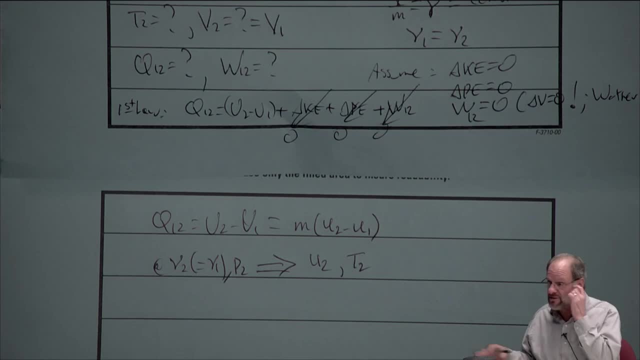 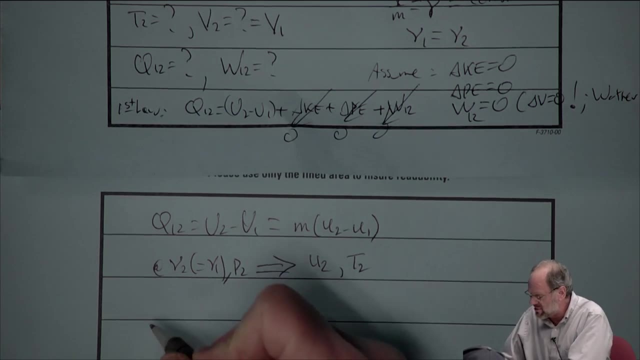 through the problem in our minds. We know that we can do the problem. Now it's just a matter of doing it, Knowing where to get all the data and all of that. So what about some data? We know that it's refrigerant. 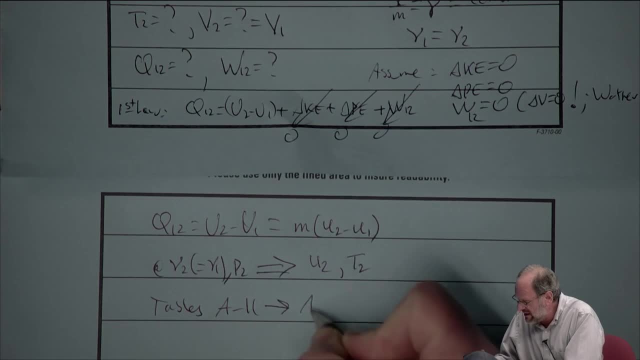 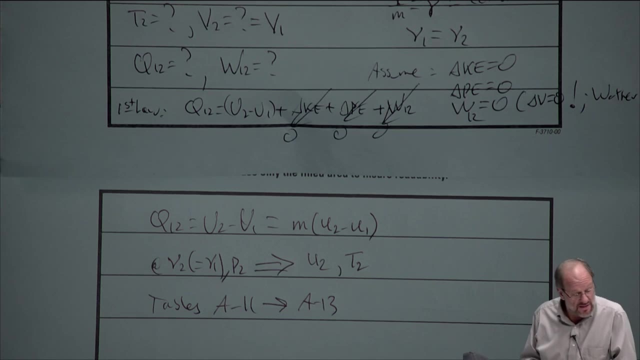 We know that all our refrigerant data is in table A11 through A13. So those are the data tables that we're going to use And now we're really set. One more thing that's always useful is to show this kind of a process on the thermodynamic property diagram. 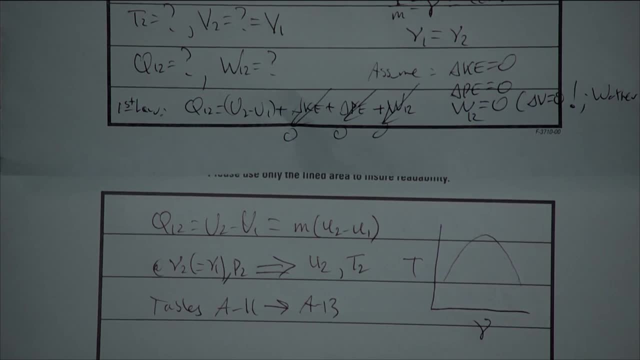 The TV diagram is very common, So I'm just going to show this on this page here as well. Where is state 0.1, and where is state 0.2? I don't really know quite yet, do I? I do know that the pressure at 2 is greater than the pressure. 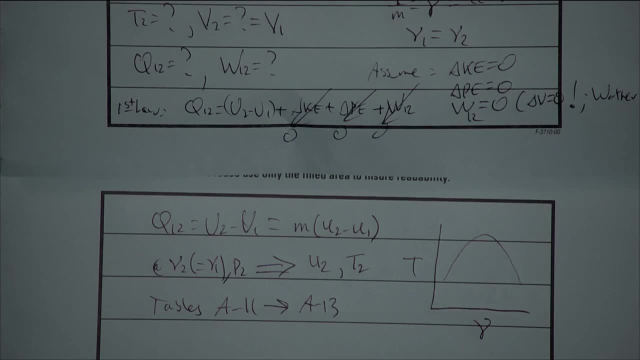 at 1, but given the initial temperature and pressure, I really don't know whether we're superheated compressed two-phase. So let's start the problem this way, by going into table A12,. okay, So at P1.. 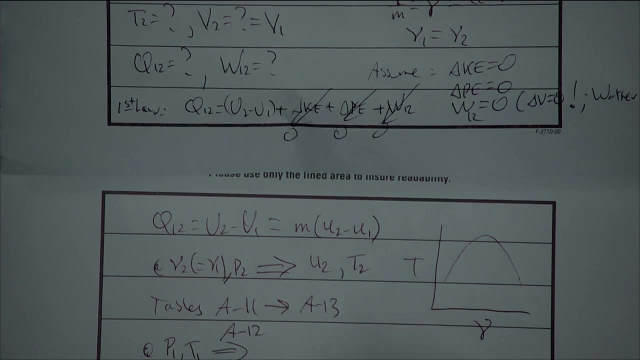 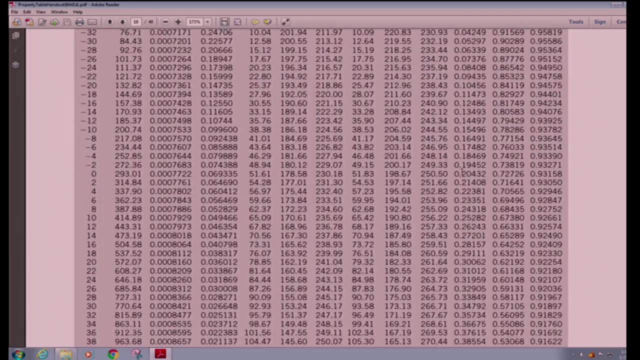 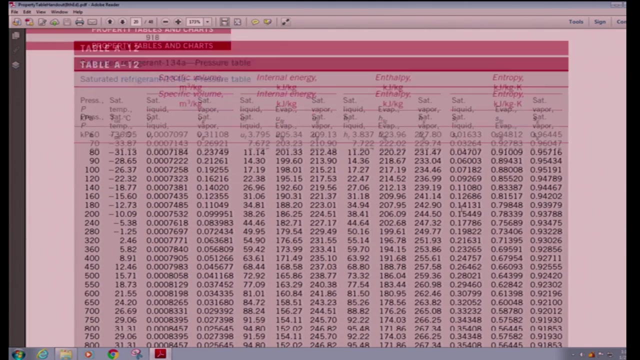 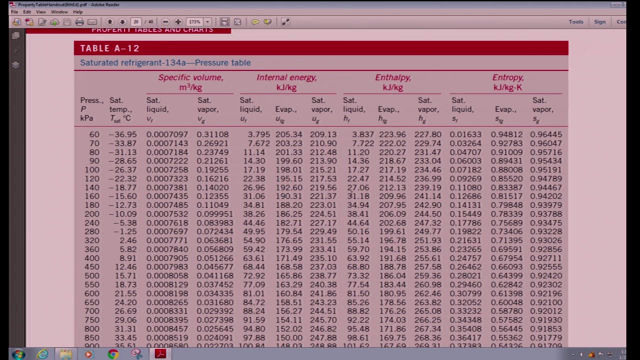 And T1.. We'll go into A12, which is our pressure table. Okay at this point, if you could put the computer up one way or the other. So this is basically table A12 now, And this is the refrigerant table in the SI units. 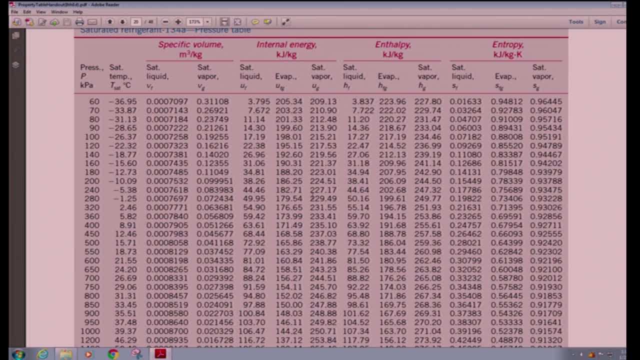 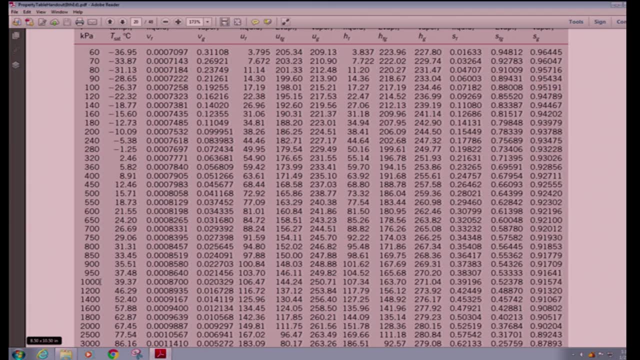 All I'm trying to do initially is see what my phase is right. So if I go into this table at the given pressure, which is 1 megapascal, that's right here, which is 1,000 kilopascals, and you can see. 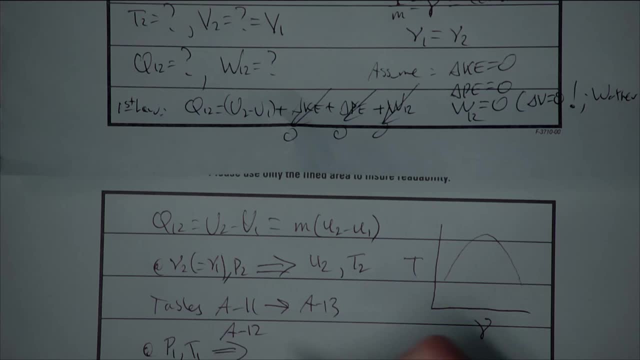 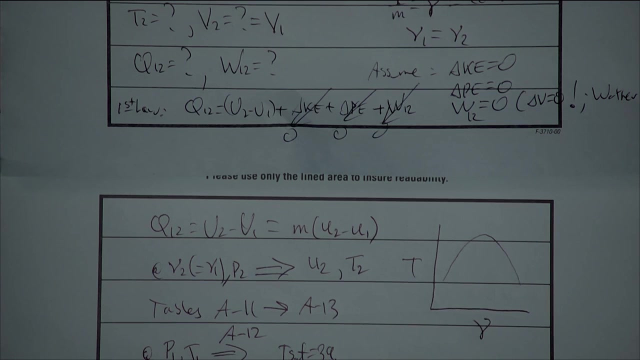 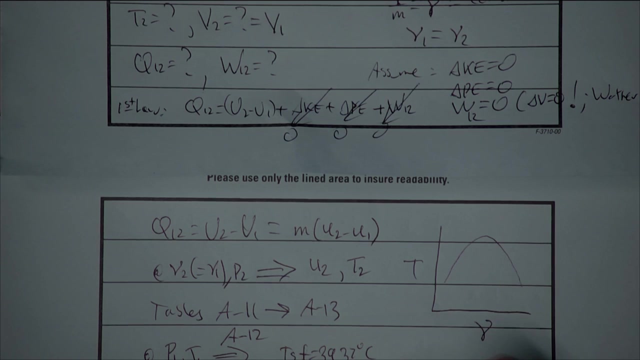 that the saturation pressure is 39.37.. So I'm sorry, I said pressure temperature is 39.37.. So at this particular pressure we find that TSAT is again 39.37 degrees Celsius And therefore T1 is greater than TSAT. 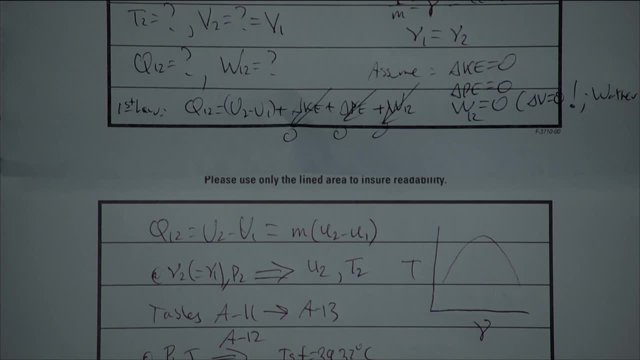 And therefore it's a superheated vapor, right. So we take this test. We know it's superheated And we don't know exactly what the value is, but we definitely know that it's superheated. So my state 0.1 has to be over here somewhere. 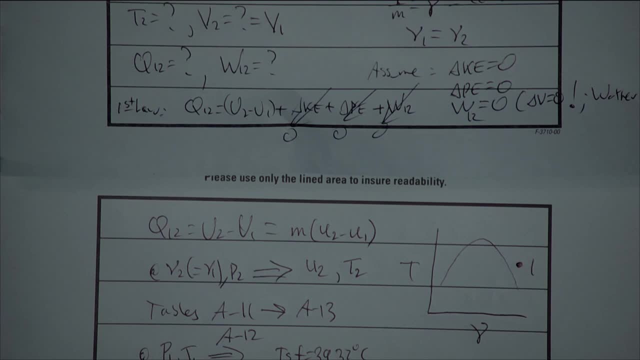 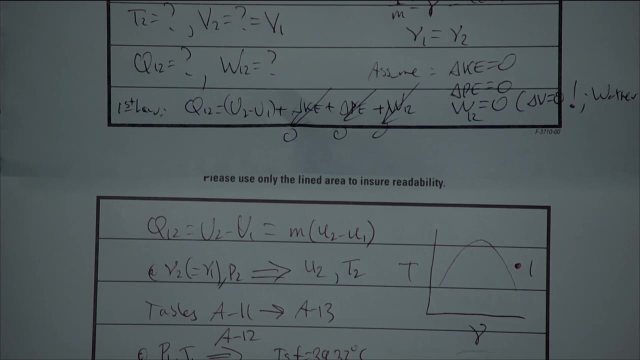 We also know that it's a constant volume process And that the pressure is increasing from 1 to 1.4 megapascals. So note that The horizontal axis is the specific volume axis. So if it's a constant volume process, 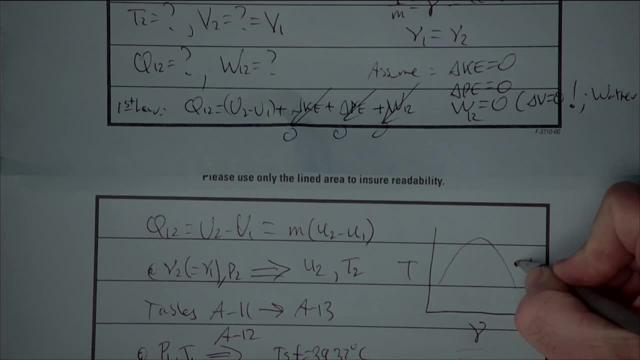 it has to be a vertical line And we have to move upwards, because we know that the constant pressure lines move upwards as we go to higher pressures. So this is the basic process. Now, at some point I'm going to get to state 0.2,. 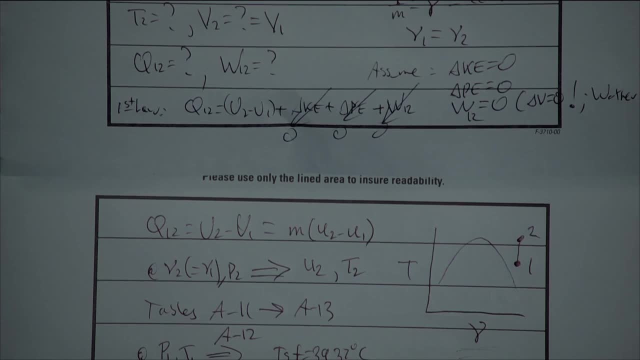 and I could do a check to see what the phase is at state 0.2,, but we don't need to really right, It should be entirely obvious. We'll start at a lower pressure, We'll move through a constant volume pressure process. 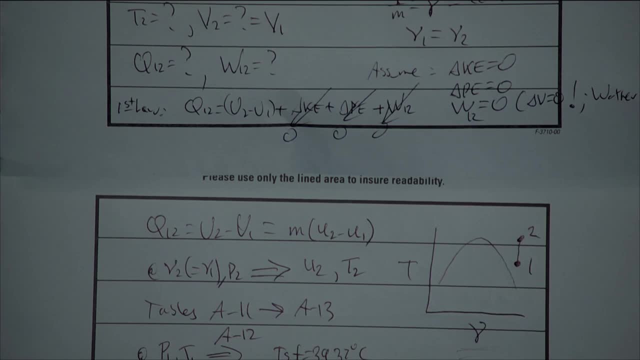 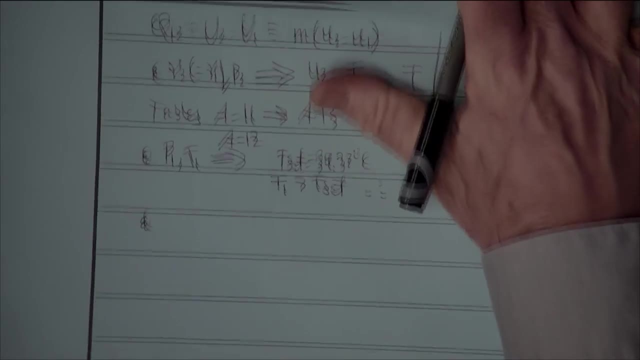 to a higher pressure. So 0.2 has to be above 0.1.. It's definitely going to be superheated. Okay, So we see that it's superheated, So now let's just get our data. So at P1 and T1 being superheated. 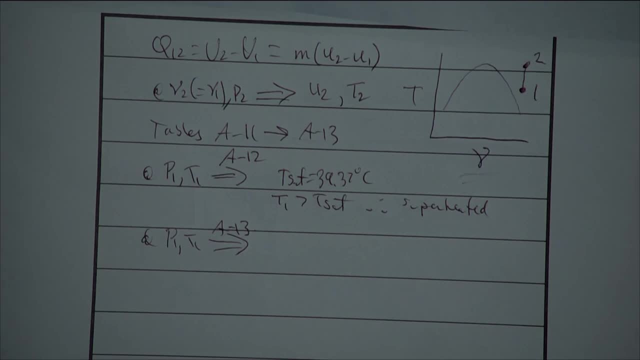 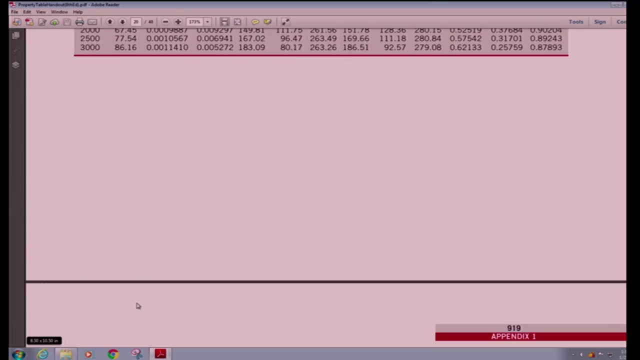 we know that our data is really in table A13.. So we're going to have to go to our subtable And we're going to have to go to our sub table. Make sure I did that, right, Right. So now we go to table A13. 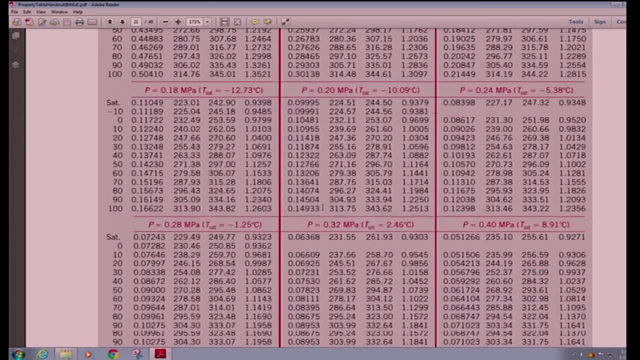 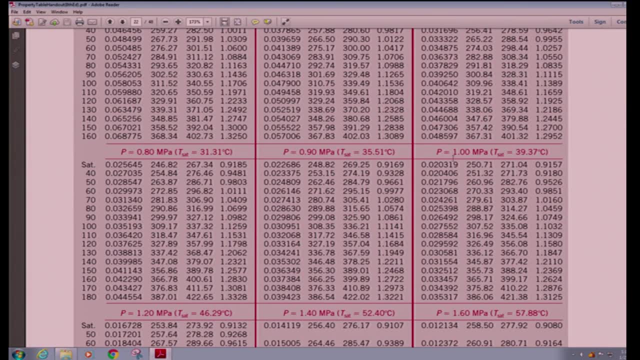 And we find the subtable that corresponds to our pressure at 0.1, which is 1 megapascal. So here it is, over here And we come down to the 50 degree Celsius line, And that's basically right here where my cursor is. 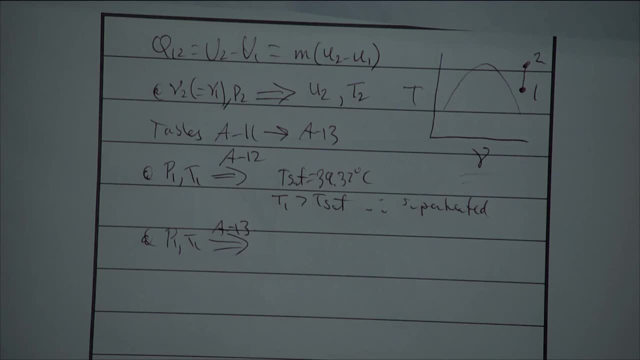 So we now write down the information just directly off of the data table. So there's a couple of things we're going to need. We're definitely going to need V1 because we need to find the volume as well as the well. we need the specific volume because at 0.2 it's the same. 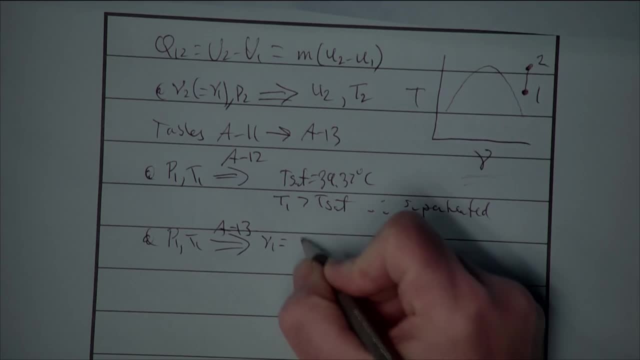 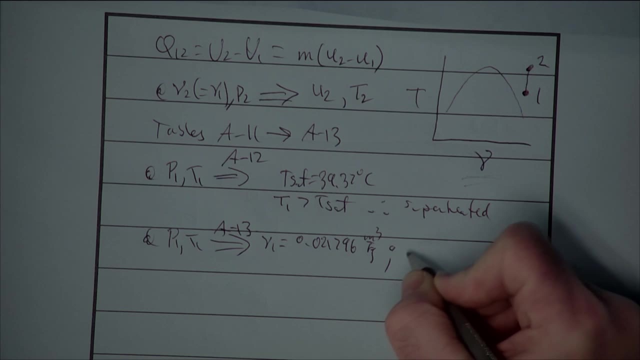 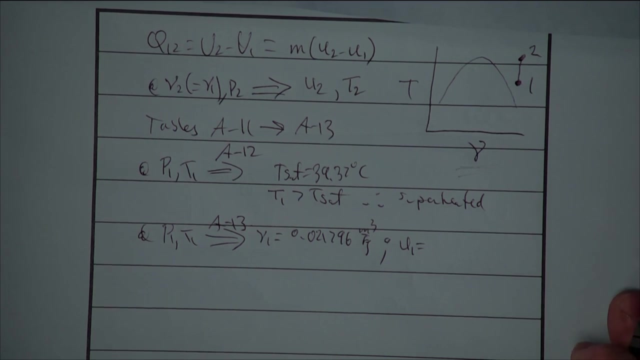 as 0.1, so we definitely need the specific volume data, And that is 0.021796 cubic meters per kilogram. We're certainly also going to need the specific internal energy at 0.1.. That's the, That's the. 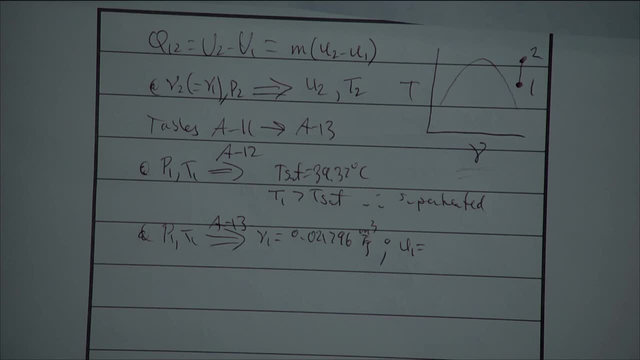 I'm sorry I couldn't hear you. You wrote this for 60 degrees Celsius instead of 50.. No, no, no, that's right. That's right. So this is what I hear: .021796.. No, I think I got it right. 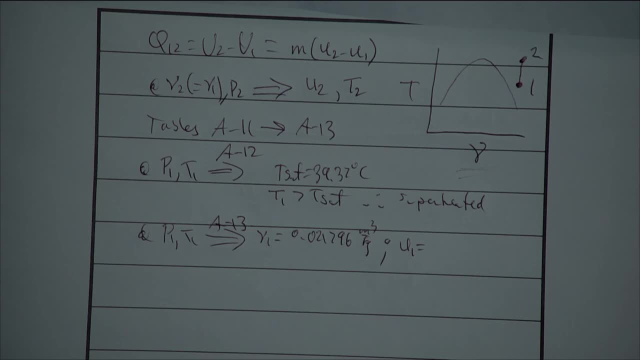 Is that from 60, though the third line down? No, no, because saturated is its own. No, no, this is the given temperature and pressure. So I mean the 1 megapascal subtable that I read. 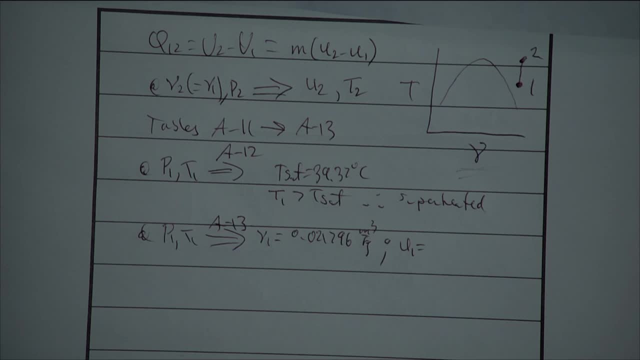 down to the 50 degree line, which is the third line. Oh, I see. Yeah, so I think you just missed by one line. Yeah, so, by the way, the top line is always going to be saturation. You would have to go into the previous table to find. 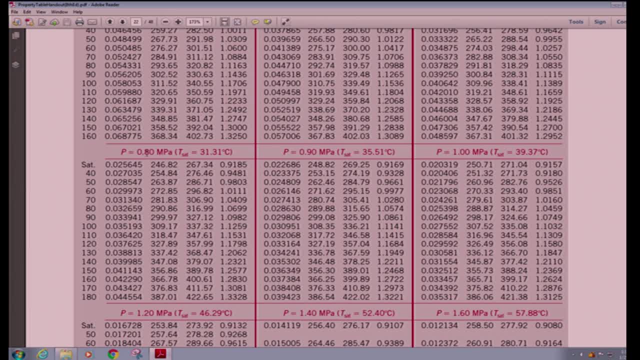 out what the saturation temperature is that corresponds to the given pressure. We don't have to worry about that right here. We're superheated, not saturated, But nonetheless it's nice to note that the first entry in every one of these subtables is the saturated vapor. 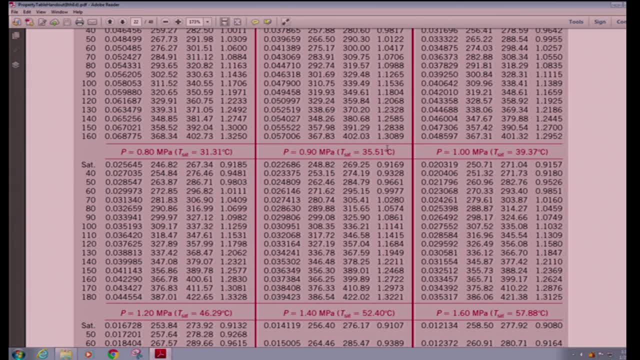 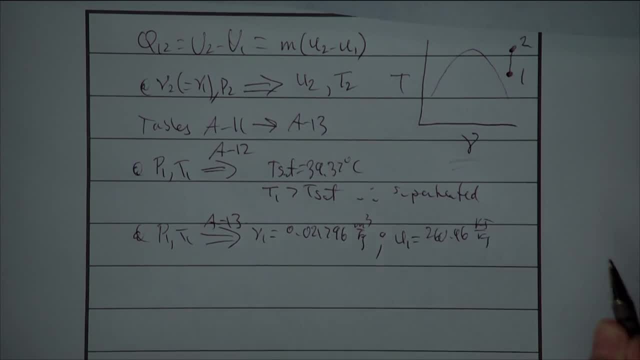 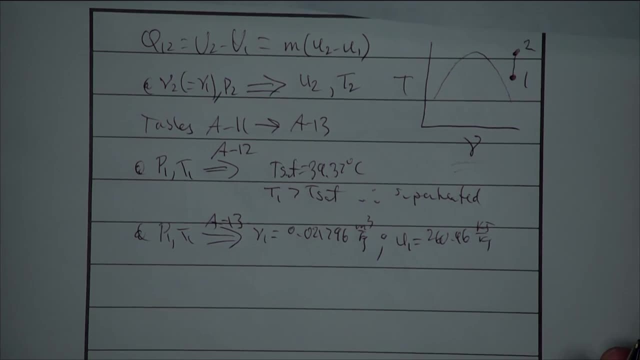 conditions at that pressure. Anyway, so we have the internal energy. now It's what? 260.96 kilojoules per kilogram. So that's all the data we need at 0.1, okay, Why don't we now find the volume since it was asked? 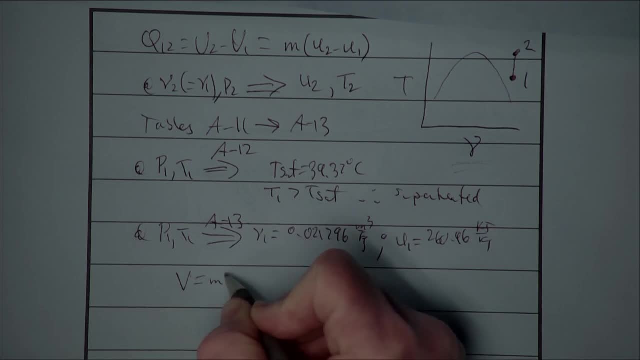 for in the problem statement. So we know that volume is mass times specific volume. The initial volume is mass times initial specific volume, which, by the way, equals the final volume. So this is just 0.1 kilograms times 0.0.. 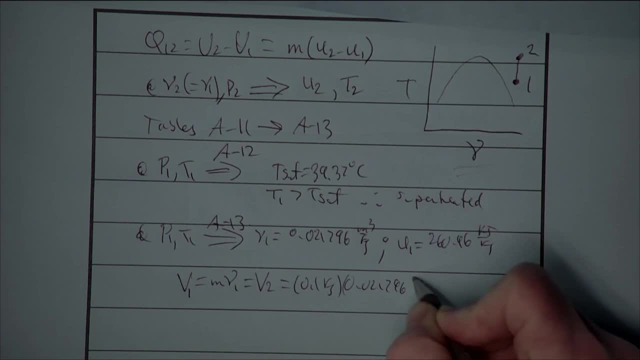 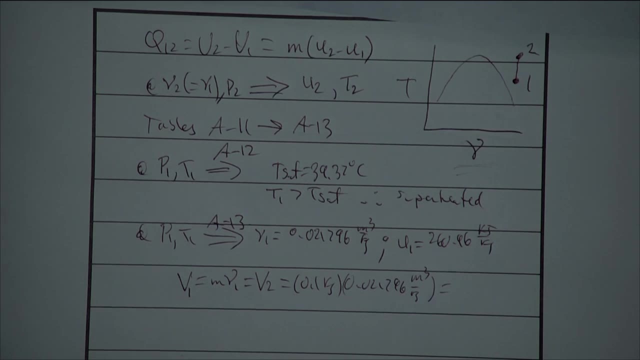 Okay, So that's all the data we need. at point one, The final volume is 0.021796 meters cubed per kilogram, And that's a pretty easy one. So we're just going to get the total volume here. 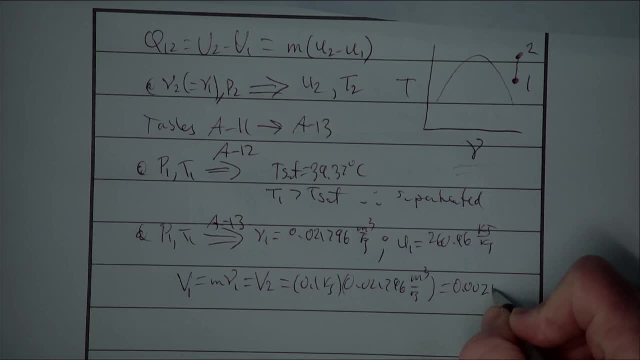 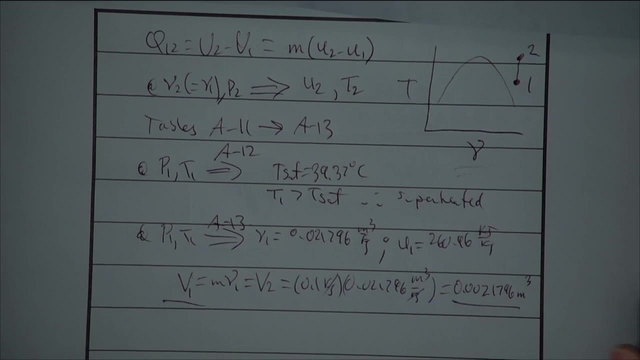 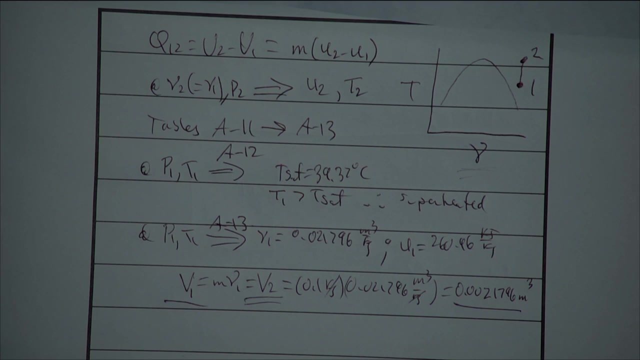 of 0.0021796 cubic meters. Note the kilogram units. cancel right. There's the first thing we're looking for. So we have the final volume. Now let's continue to our final thermodynamic state. We don't need it. 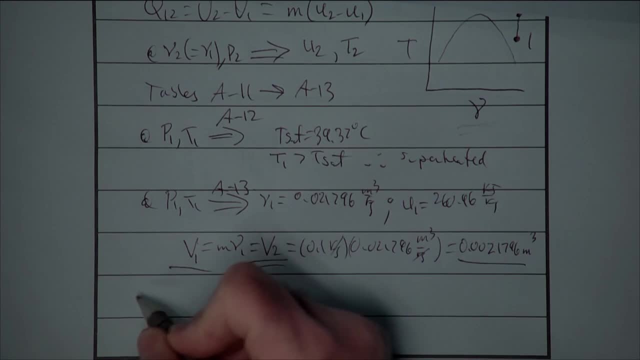 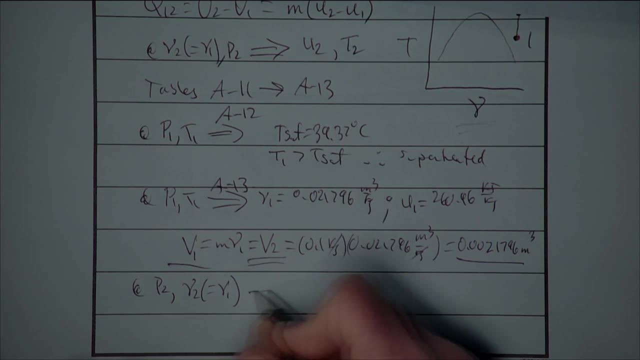 We don't need anything else here at 0.1.. We're only interested now in 0.2.. So we have two properties again, right At P2 and at the specific volume V2, which equals V1, well, 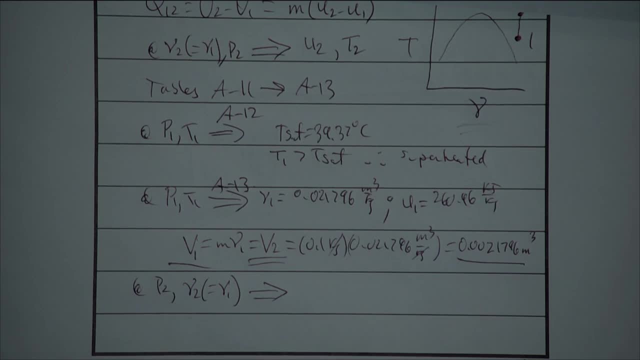 two independent intensive properties, So we should be able to find whatever other property we need. We're looking for the temperature as well as the internal energy, right? So here we're going to have to do our usual test once again, although because we've already talked about it- 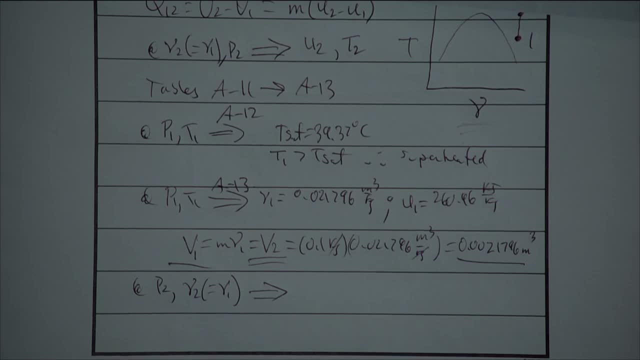 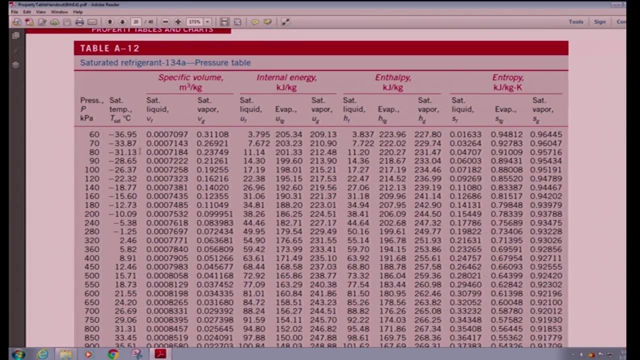 we know that it's a superheated vapor. It should be very obvious. I mean, we could just compare in Table A12. if we wanted to. We can go to the 1.4 megapascal, which is 1400,. 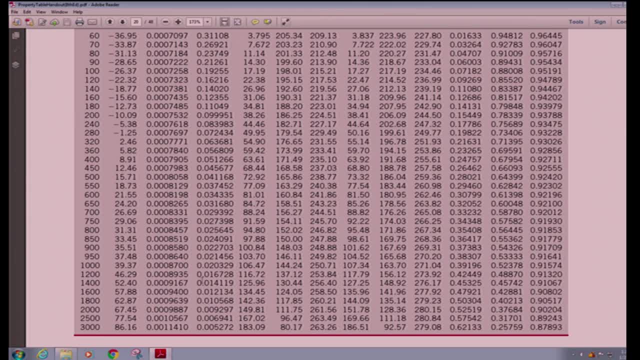 and we can come over here and this is going to be VG, and VG is 0.014119, but my specific volume is higher than that right, It's 0.021796, so we know that since VG again, if we were. 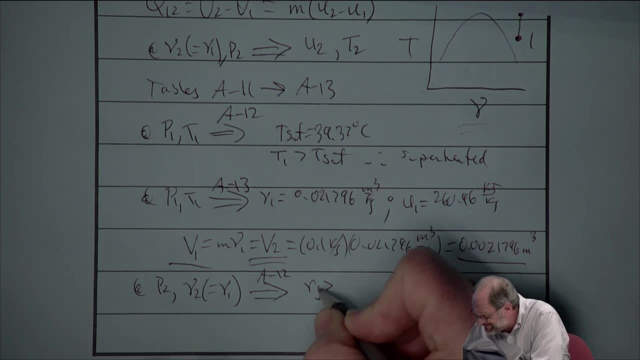 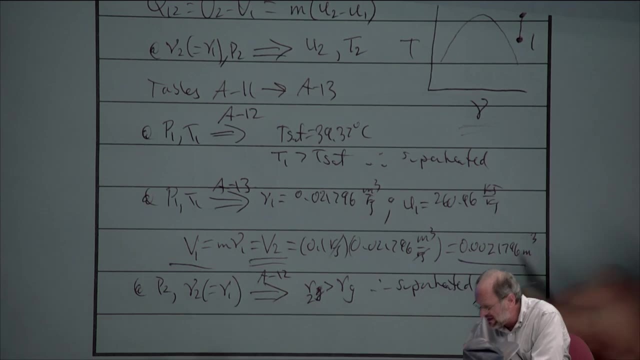 in Table A12, we know that VG is. I'm sorry. we know that my specific volume, V2, is greater than VG. Therefore it's superheated. Now again, I didn't have to do that, I'm simply doing it for illustration. 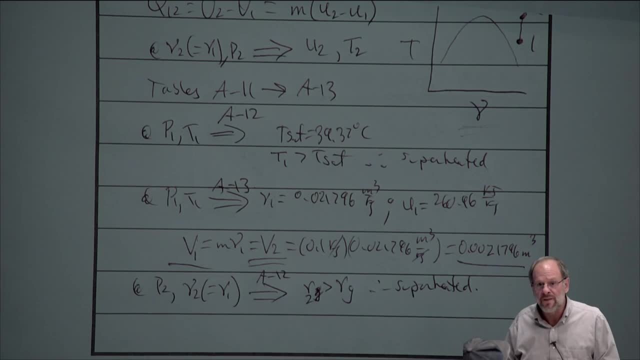 In this problem again. it should be obvious because of the diagram that we saw before. Was there a question? Yeah, Why would you not be able to find the second volume for the PV equation? I'm not sure if you mean by the PV equation. 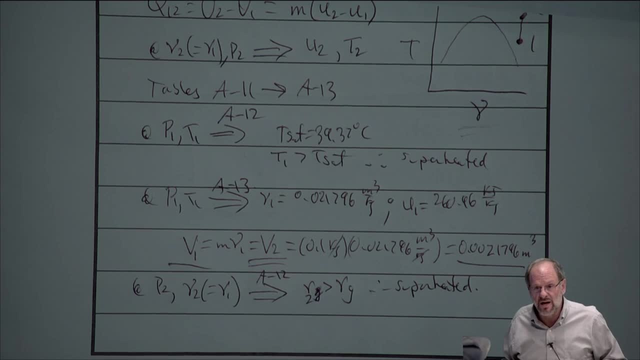 Or PV equals like MRC. Oh, it's not an ideal gas. It's not an ideal gas, I mean no. no, I mean, if we have refrigerant, we always want to assume that the most accurate data that's available. 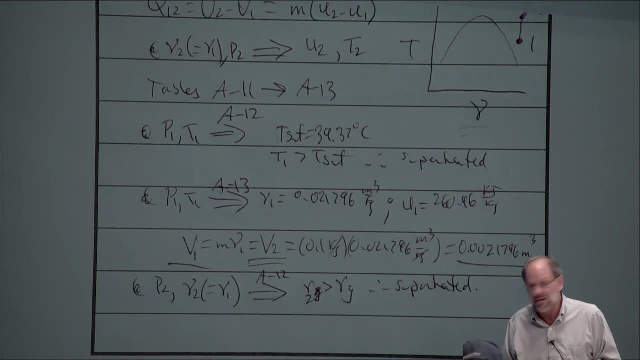 to us is the data from the tables. I mean, frankly, it might be an ideal gas. We'd have to make some tests to see so- but you know- that's really an approximation- that the best results will be from using the best data. 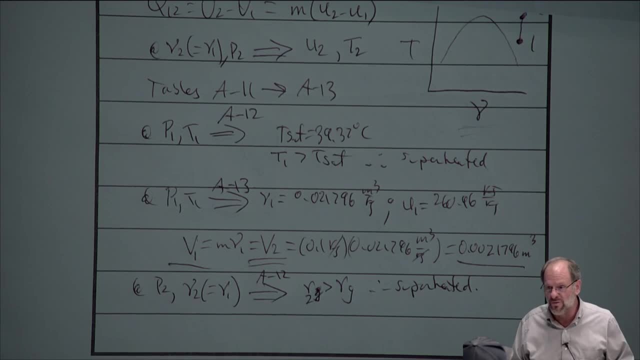 So, whenever you have a problem involving water, use tables A456.. Whenever you have a problem involving the refrigerant, use A1212.. And I wouldn't go so far as to say that it's incorrect to assume that this is an ideal gas, but there's just no point. 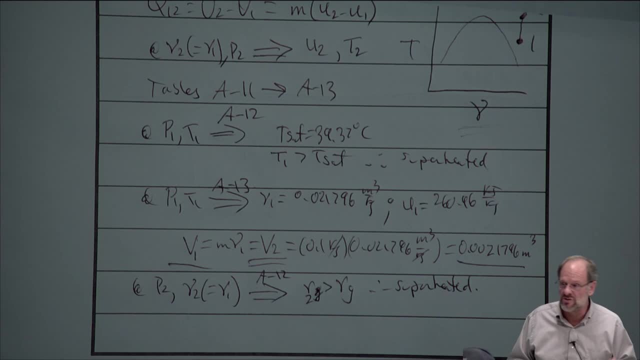 in doing so when we have such good water tables- I'm sorry- good refrigerant tables available to us. Okay, You know you might be interested. you know, when you go home, try it using the ideal gas equation of state and see if you get similar results. 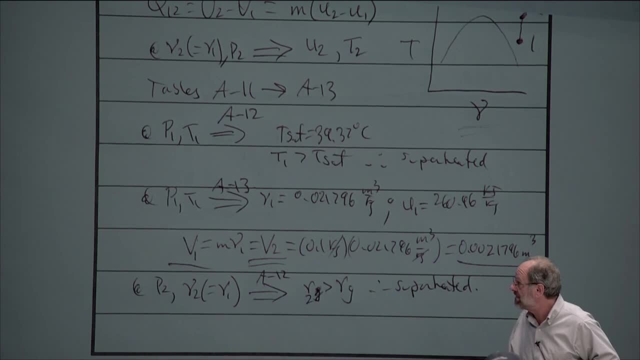 Maybe we do, maybe we don't, I'm not really clear. I didn't know about the ideal gas, but Equals one or less than or greater than one. Does it stick to this? If it's an ideal gas, then you have to use the ideal gas equation. 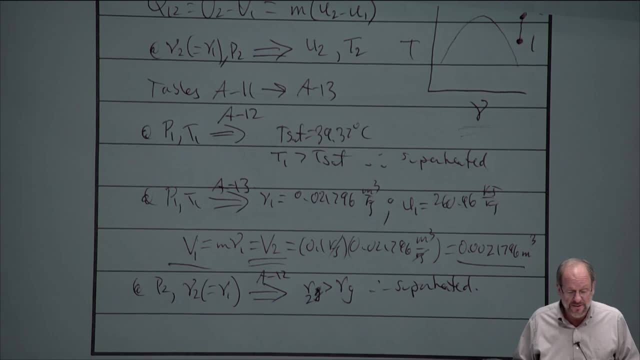 of state and or compressibility chart. If it's not an ideal gas, then you would use the data for the tables. Maybe I'm not clear what your question is, But I can't just even if it's an ideal gas like: can you still use the chart? 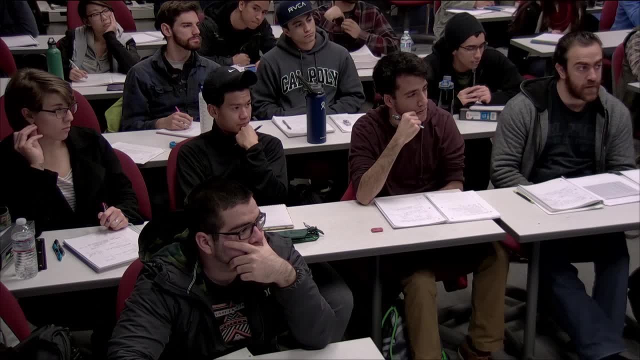 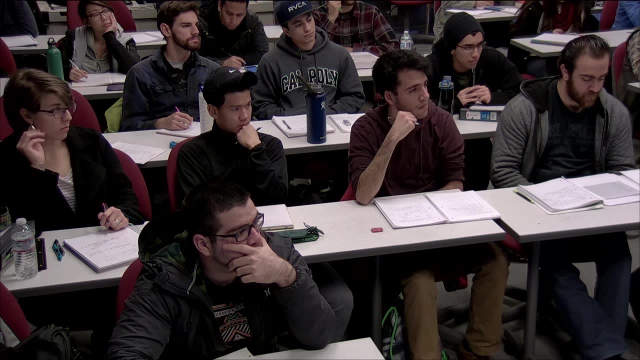 Well, yeah, sure, sure, If you conclude that it's an ideal gas, you can still certainly use these tables, All right, But in general, I wouldn't assume that problems involving water or the refrigerants are ideal gases. I mean, this problem is rather unique because it's always 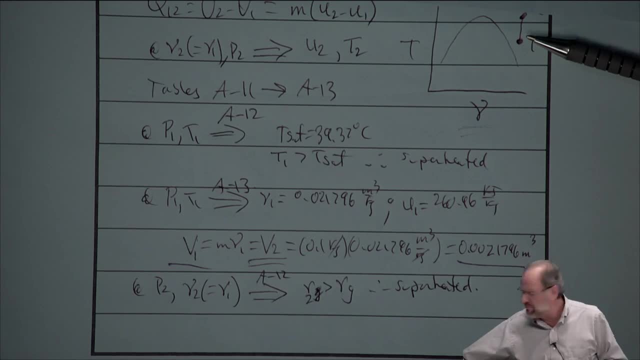 in the superheated vapor region. so it's a gas, But many problems you'll have. maybe one state point in the saturation region and the other in the superheated region, or maybe one compressed liquid and the other is superheated, or maybe another one is saturated. 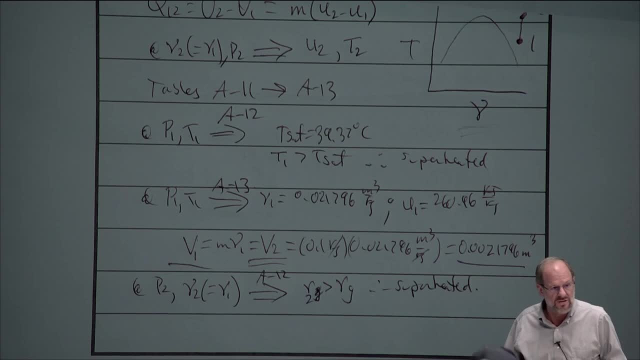 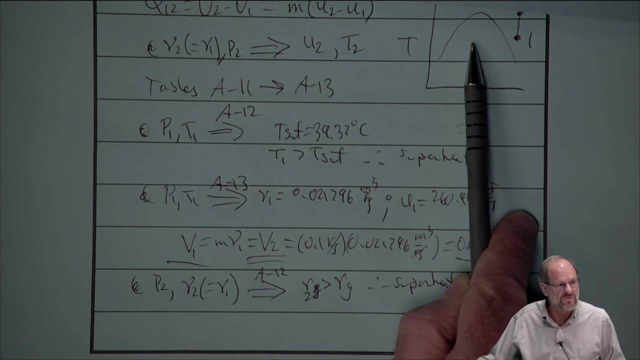 If the entire problem is not an ideal gas, you can't use an ideal gas relationship. I mean, you might have a problem like this one, but maybe then there's a process where state point two is not an ideal gas. State point two is somewhere in the two-phase region. 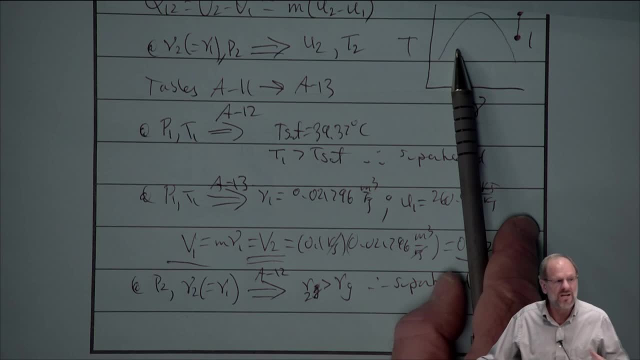 Two-phase mixtures are not gases. They're mixtures of liquids and gases. so immediately you tell yourself: nope, you can't use an ideal gas equation. But realistically, whenever you have water or the refrigerant, don't use ideal gas equations. 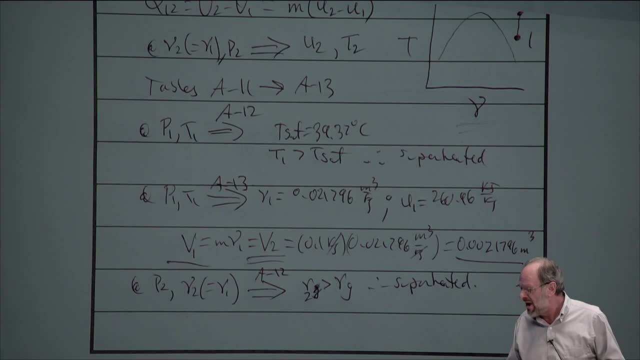 Use the actual data from these tables. That's better for accuracy, All right. So now we know that point two is a superheated vapor. We've seen it by this test. We've also seen it on the diagram. So now that we know that it's superheat, well again. 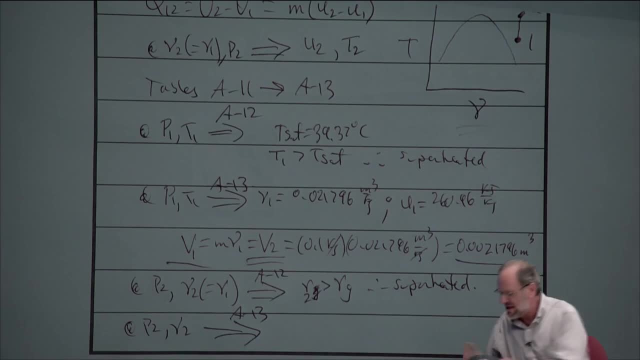 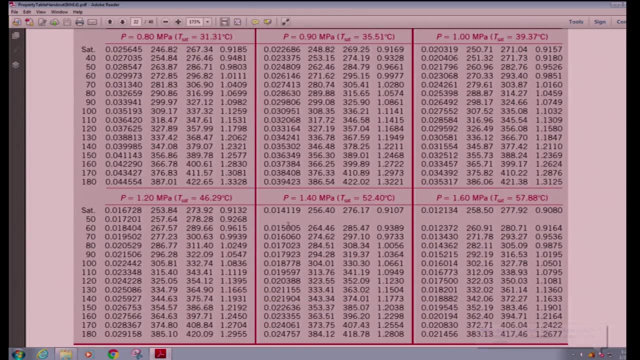 back to the appropriate table, which is table A13.. We have to go to the right subtable. So now we're at the 1.4 megapascal subtable which is down here and we're trying to find the pressure. 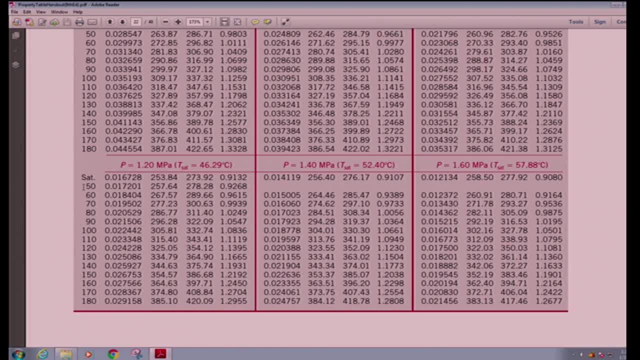 and specific volume where the two of them come together, Can't really do that, can we? We know that V1 is equal to V2.. We know that V2 is 0.021796.. But I don't think we're going to be able to do that. 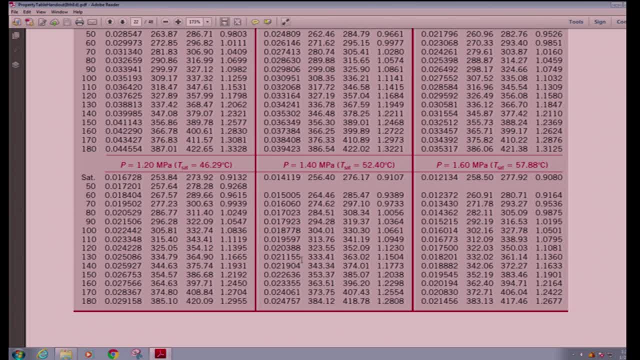 I don't think we're going to be able to do that. I don't think we're going to be able to do that. I don't see a 0.021796.. I see an entry here at 130 degrees, which is a little bit lower. 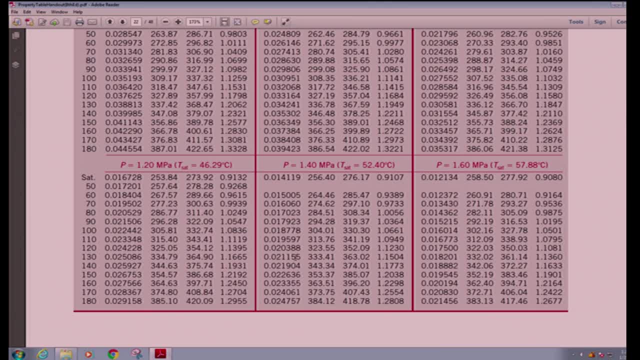 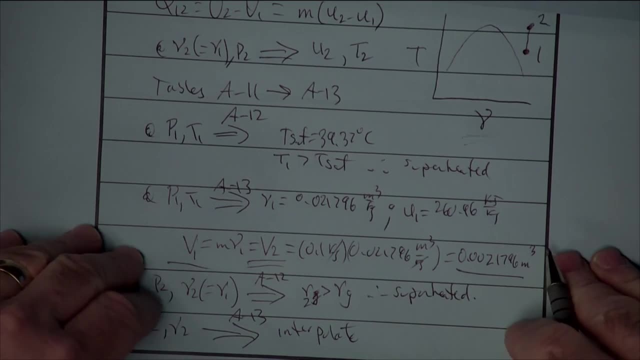 in specific volume, right, I get 0.021155, and then I have another specific volume corresponding to 140 degrees, which is higher than my specific volume. So I'm somewhere in between. So unfortunately I have to interpolate. This is very common. So, as we interpolate, Let me just create the little table here. So we have this 1.4 megapascal subtable And I am going to be interested in temperature, And I know that my temperature is somewhere in between 130 and 140. 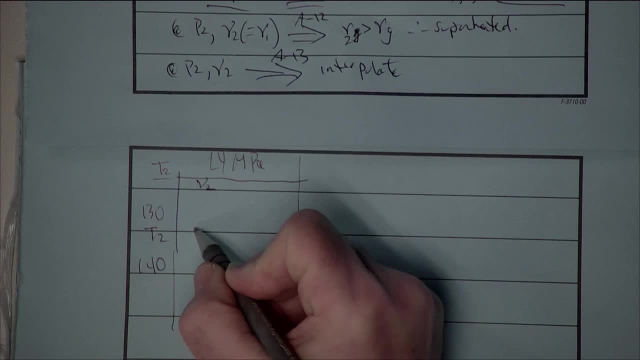 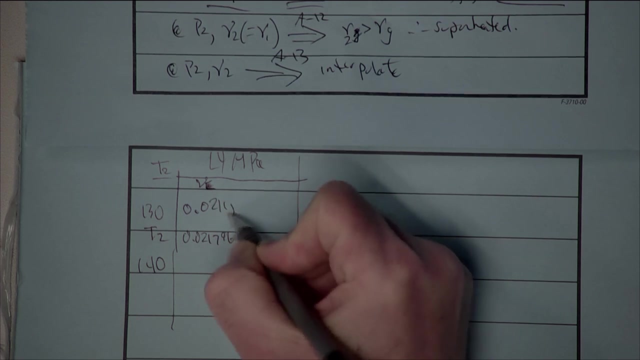 I'm also going to be interested in specific volume. So I know whoops, so that I know that my specific volume is 0.021796.. And I know, at 130 degrees the specific volume is a little bit different: It's 0.021155.. 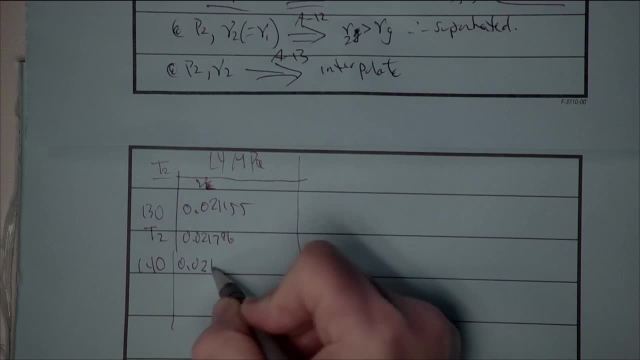 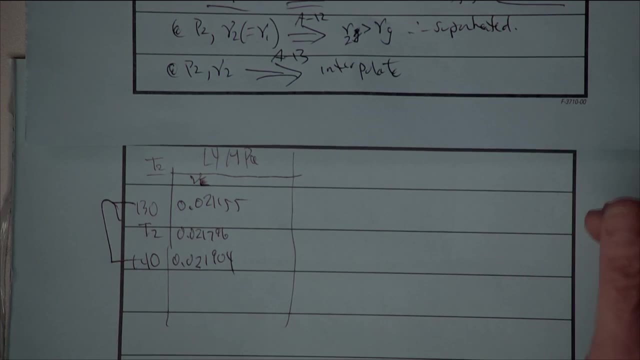 And at 140, it's 0.021904.. So I'm going to have to do my interpolation in between right And I'm going to do the same thing on internal energy. I need internal energy at state 0.2.. 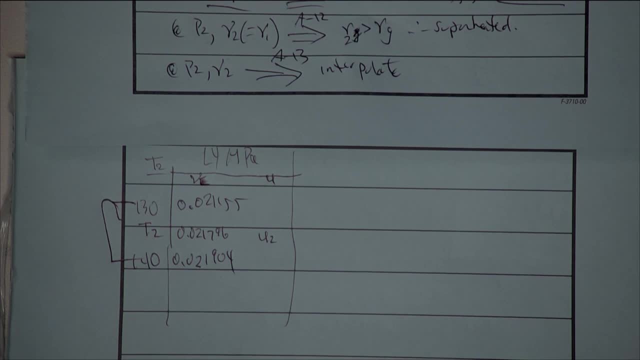 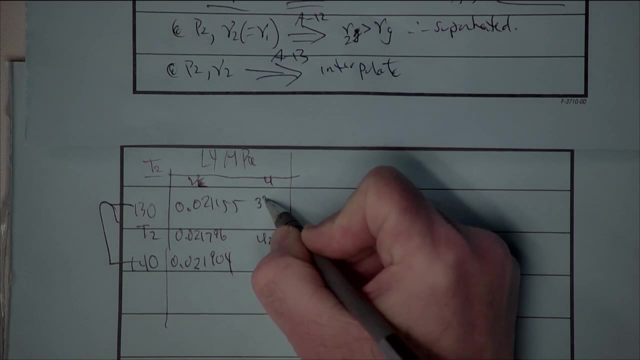 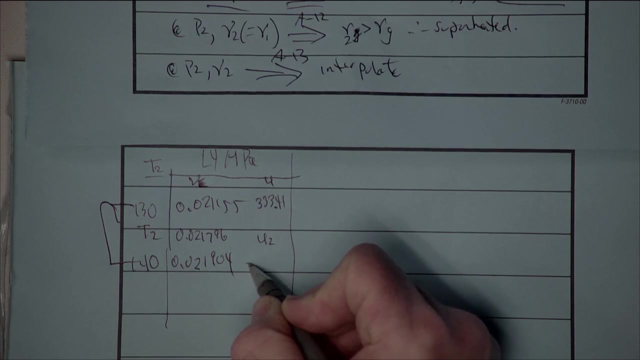 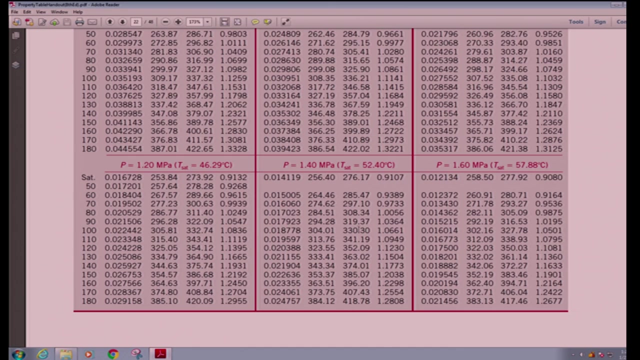 It's unknown, But I know that it's found similarly by interpolation. The internal energy that corresponds to this pressure, but at 130 degrees, is 333.41.. And then corresponding to 140 degrees is 343.34.. So here's the internal energy column. 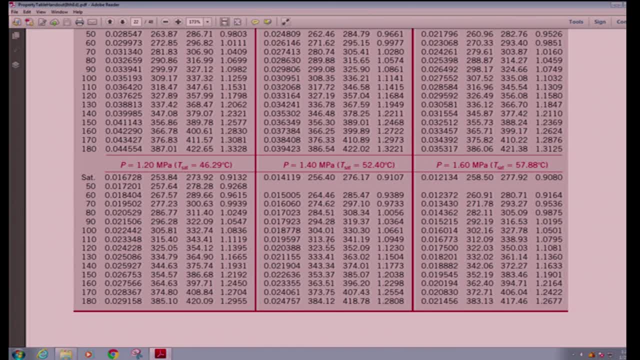 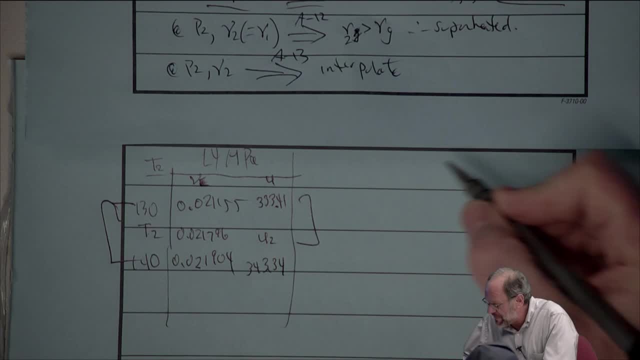 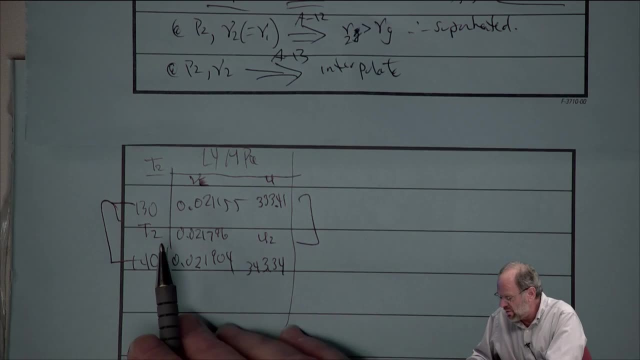 Whoops. no, Here's the internal energy column And here's my internal energy column And here's my numbers right down here. All right, so we interpolate And remember that interpolation is really just finding the ratio of property differences. So let's just start by interpolating. 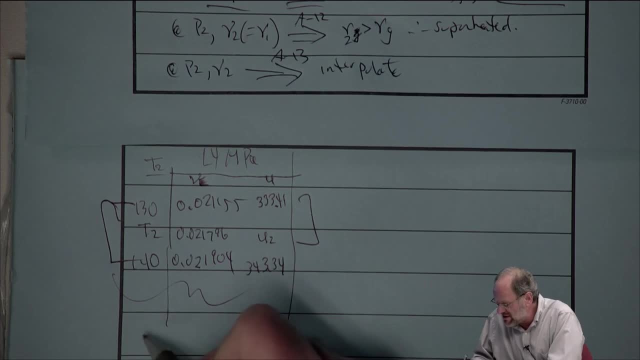 on temperature and specific volume. So basically I would get 140 minus T2 over 140 minus 130. So it's basically this temperature difference over the full temperature difference And then that will have to equal the corresponding specific volume differences, So that what corresponds to 140 is 0.021904 minus. 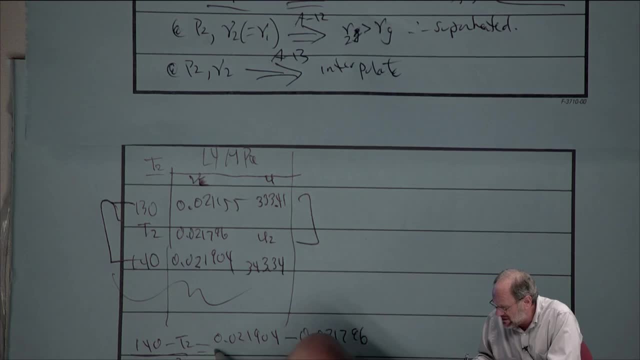 And then my specific volume is 0.021796.. And then again divided by the specific volumes that correspond to 140, 130.. So 0.021904 minus 0.021796.. And this will equal the total volume differences. 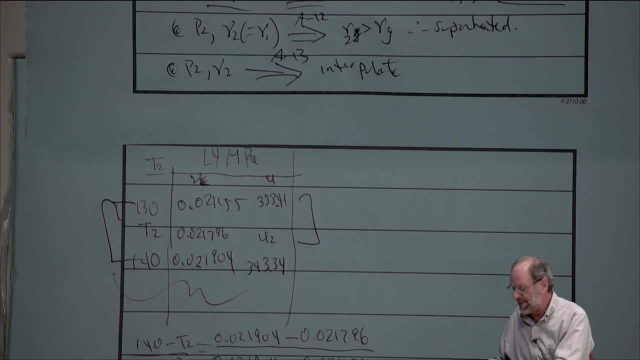 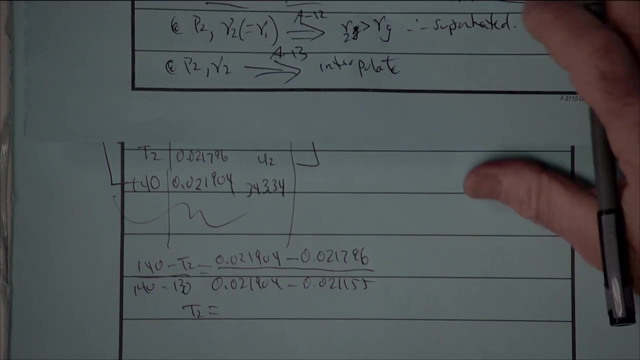 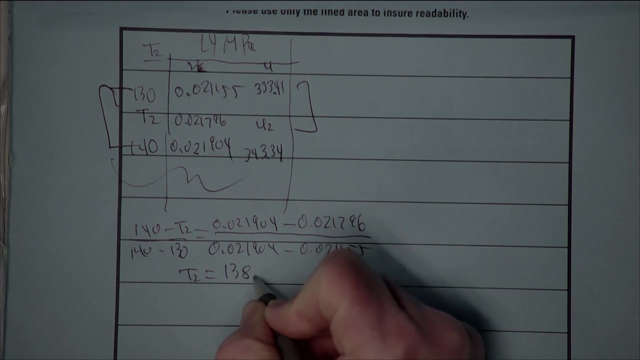 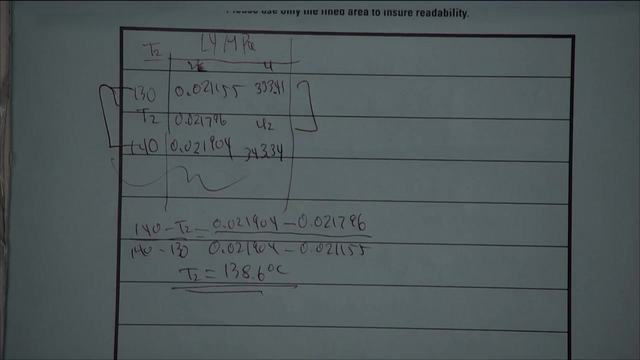 So now we just go through a little bit of mathematics. There's only one unknown, so it's pretty easy to solve for, And we end up with a value of T2 equal to 138.6 degrees Celsius. So it's just a matter of interpolating on the tables. 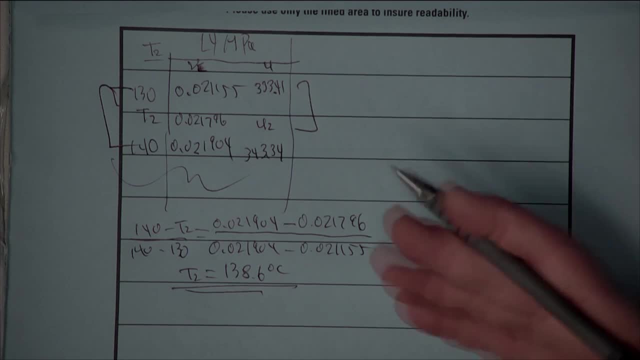 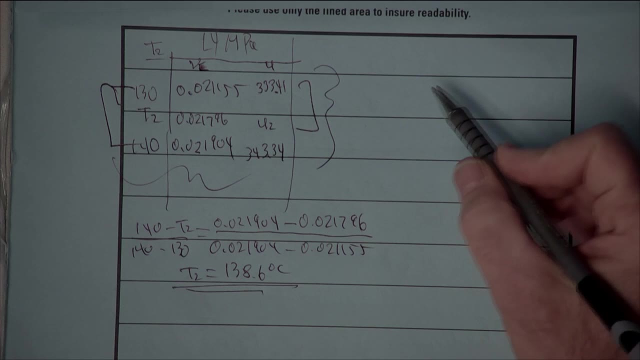 Now we have to do the second interpolation, and this interpolation deals with internal energy, but it's the same type of interpolation, right? So let's just do this one over here, to the right. So we're going to do the same thing we did before. 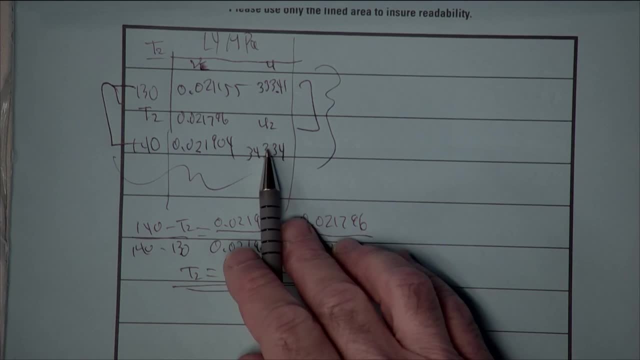 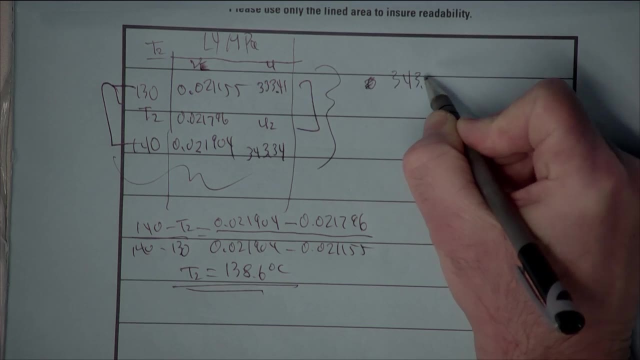 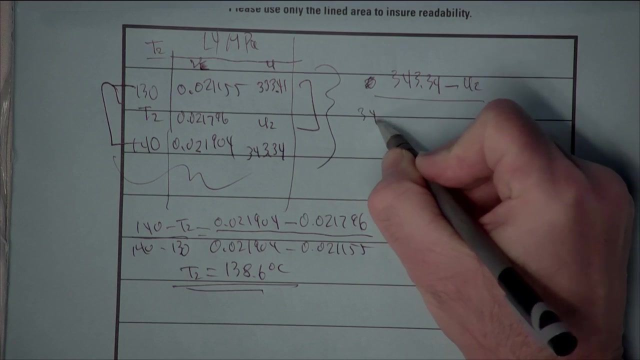 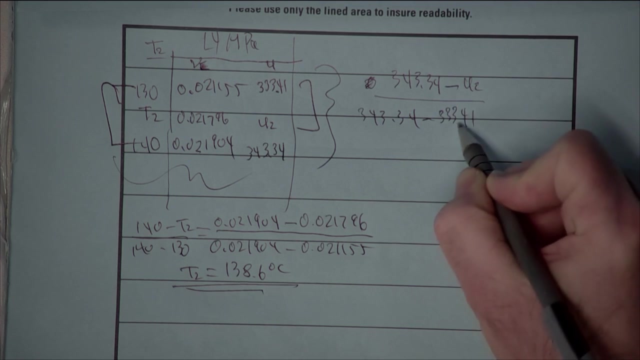 We have the internal energy that corresponds to 140.. So, whoops, 343.34 minus U2 over the internal energy that corresponds to T2.. So we have the internal energy that corresponds to 140 minus the internal energy that corresponds to the temperature of 130, right. 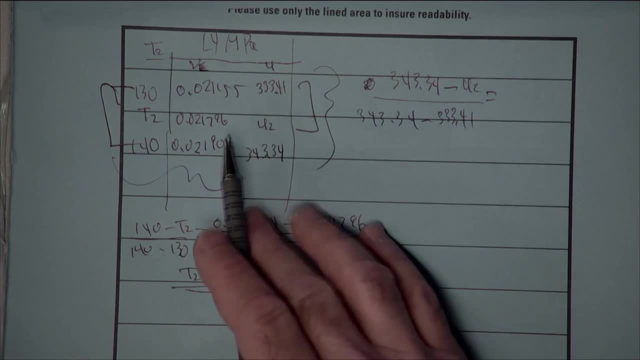 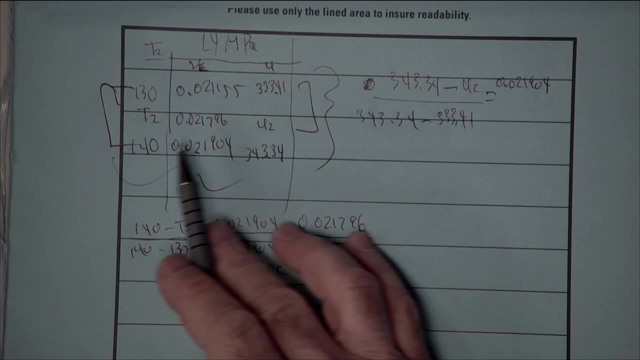 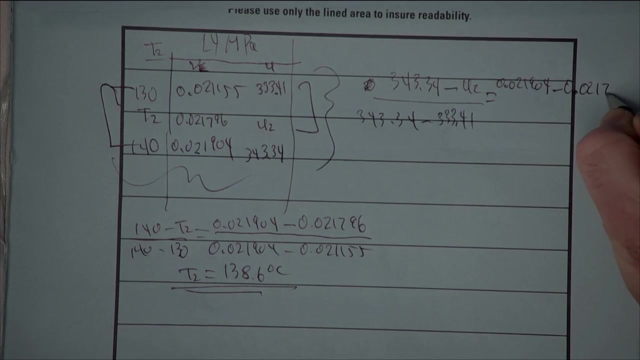 And now we're doing this based on the specific volume data. So we have the specific volume of .021904.. That's the specific volume that corresponds to 140.. And then minus the specific volume of .2, which is .021796.. 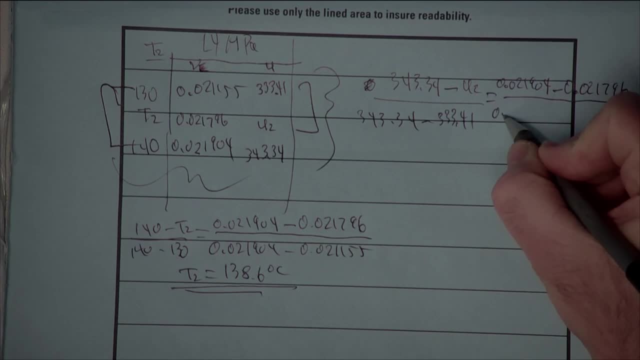 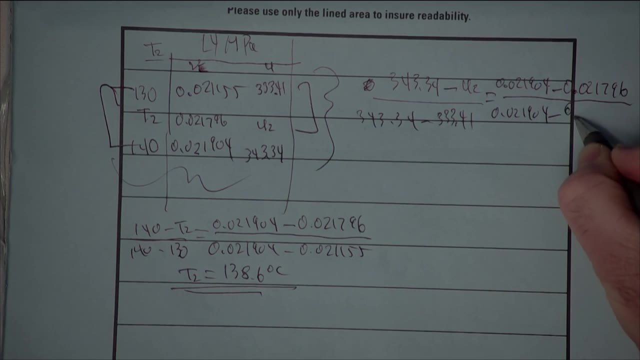 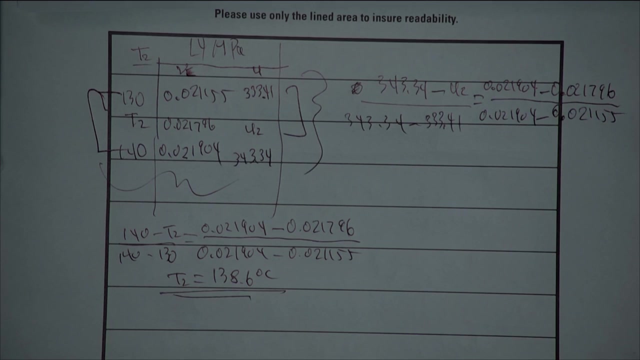 And then divided by So we have those same specific volume terms: The one that corresponds to 140,, like this temperature does less the one that corresponds to 130.. So that's .021155.. Okay, So it's essentially the same thing. 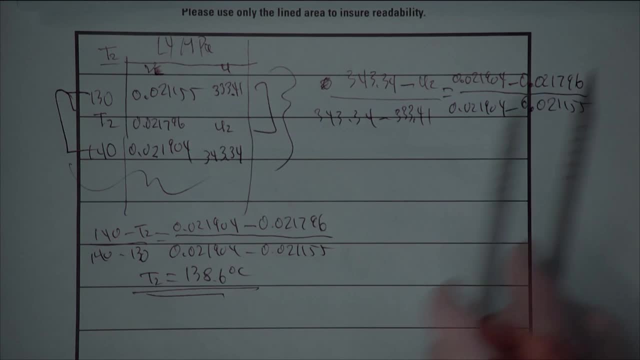 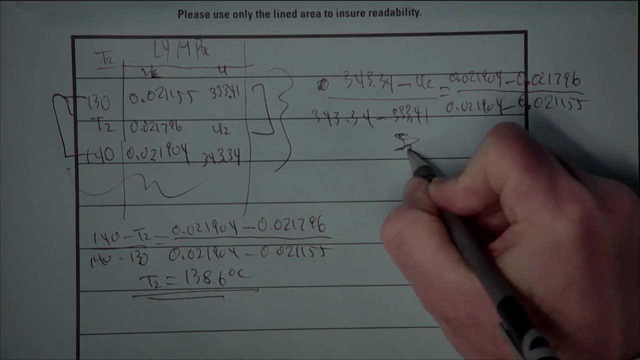 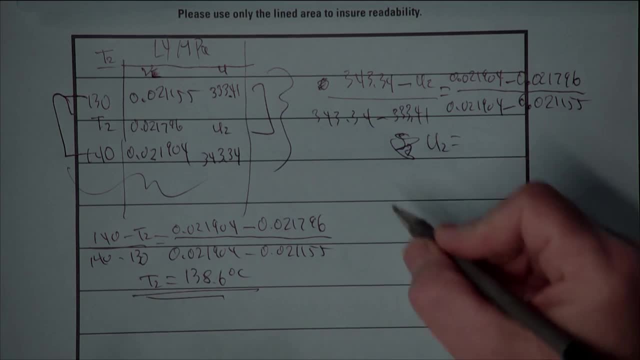 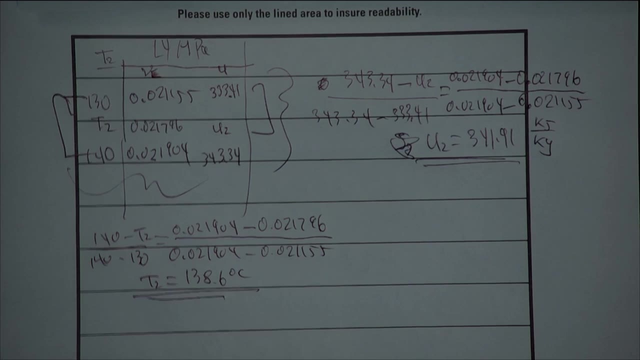 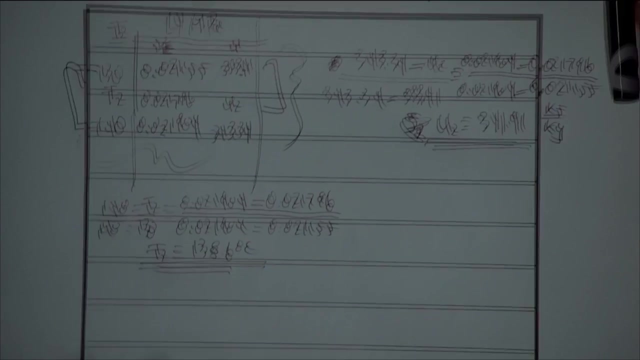 this one's pretty easy as well. You end up with a value of 341.91.. And this is going to be in kilojoules per kilogram. So now we have all the thermodynamic property information that we need. Now we can finish up the problem. 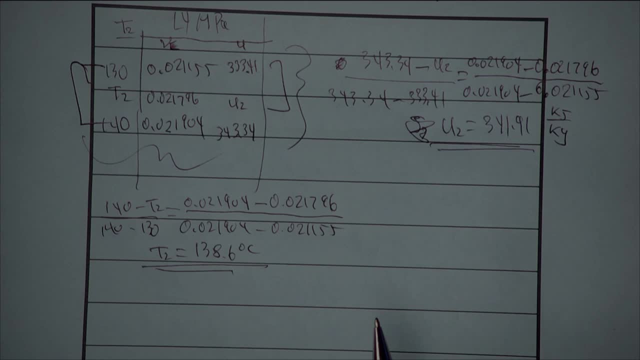 All right. So let's see, We have T2.. We've already found V2.. We need to find two more things. We need to find heat transfer and we need to find the work. Let's do the work first. Well, we're done. 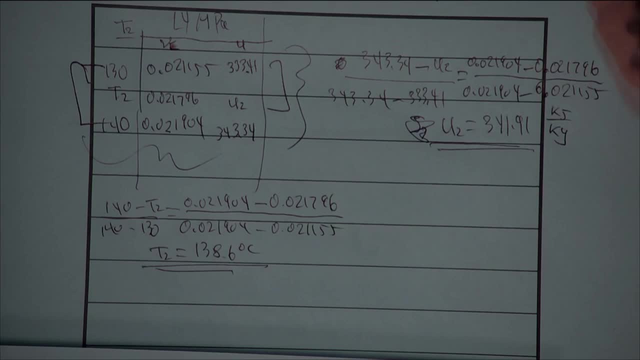 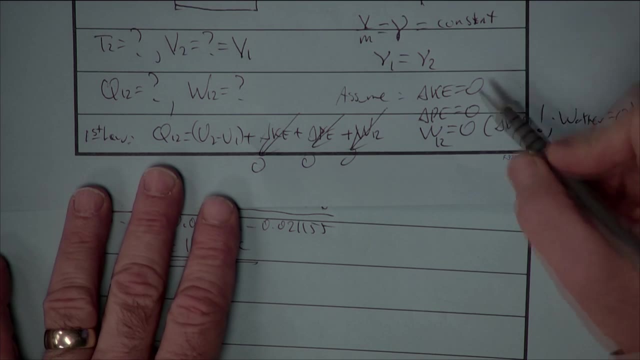 We already talked about the work, right. I guess I should have made a better point of that, But when we were talking about the work before you know, we had noted that there's no volume change, so therefore there's no boundary work, right. 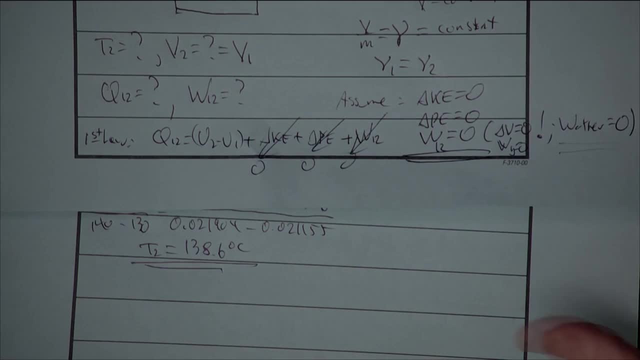 And there's no other forms of work, so the work is just zero. So we're actually done with the work part already. So if you want to go back a page or two, you can underline that or you can just rewrite it here. 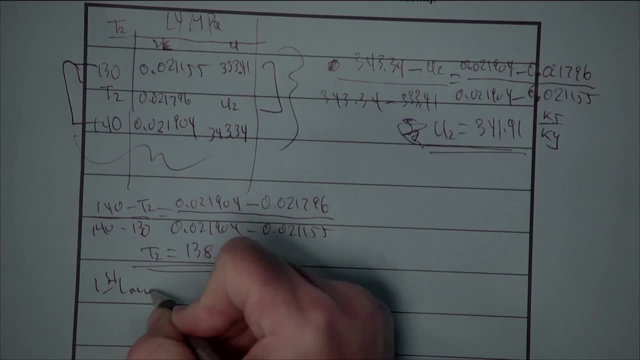 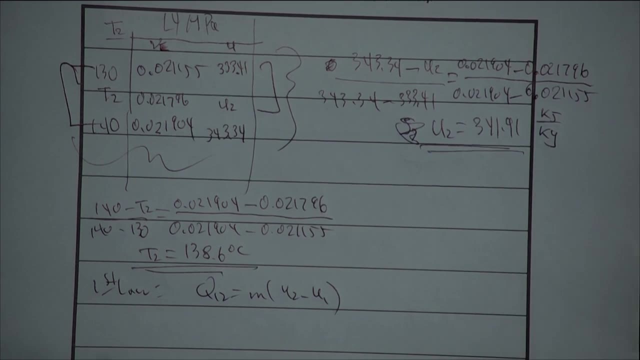 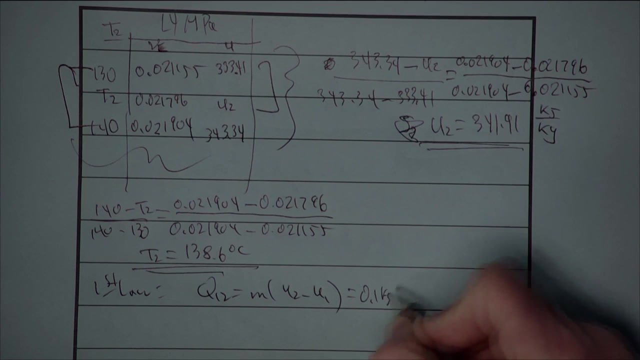 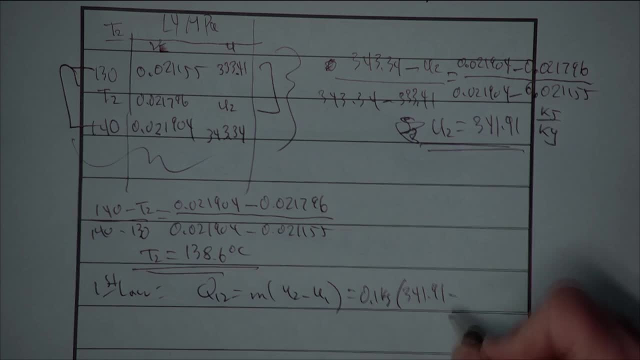 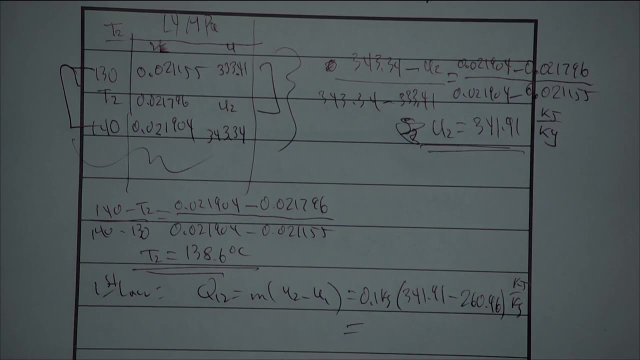 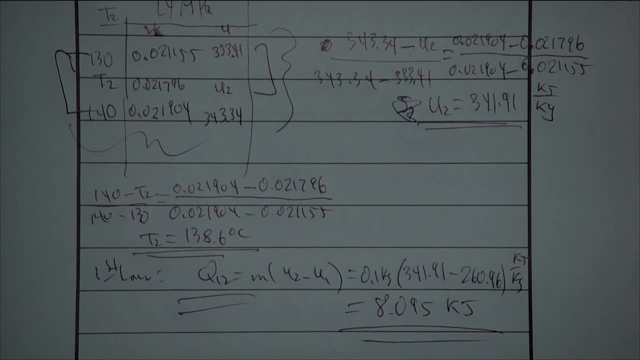 Okay, And that completes the problem. Now, before we're completely done, you know, maybe we'll just look at some of the results and make sure they make sense. One thing I didn't do, which always makes sense, is to look at the interpolation and see. 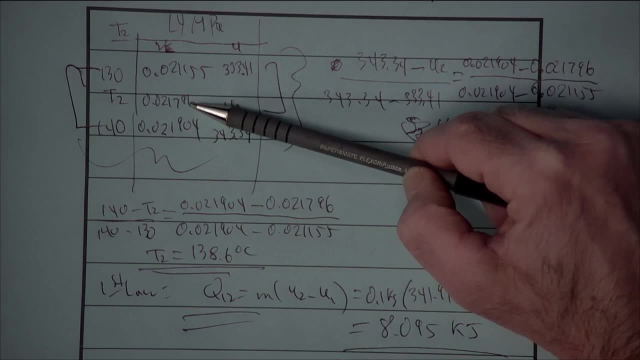 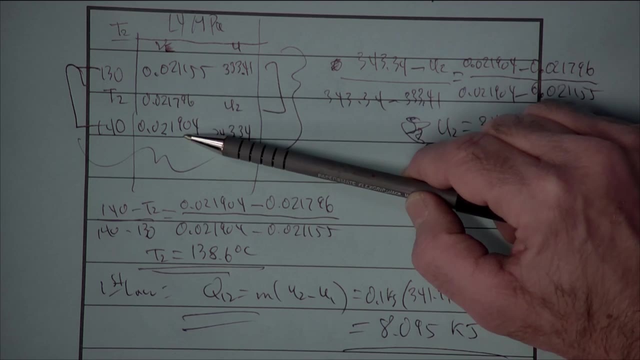 if the number you end up with makes sense. For instance, if we come here to the specific volume data, you can see that this is about what? 0.0218.. That's certainly a lot closer to 0.0219 than 0.0211.. 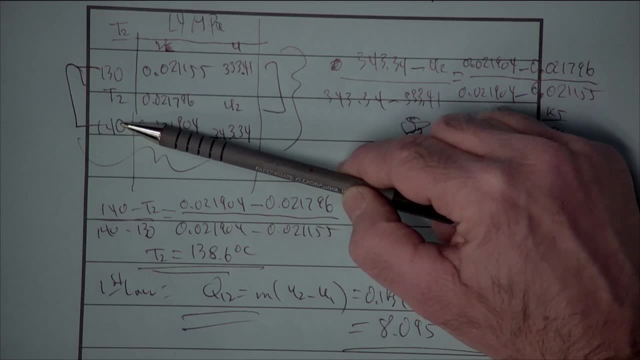 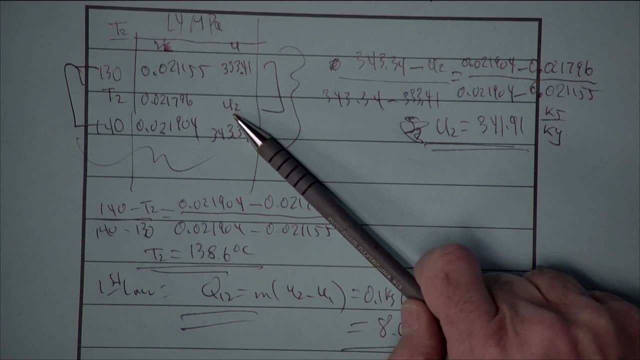 So you would expect that the final temperature is significantly closer to 140 than 130. And indeed we found that it is. And the same thing goes for the final temperature. It goes with the internal energy right. We would expect the internal energy to be a lot closer. 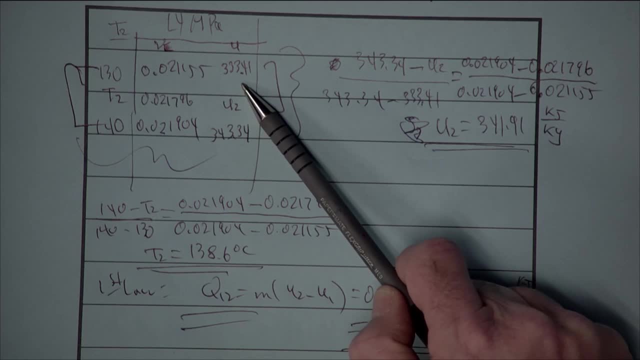 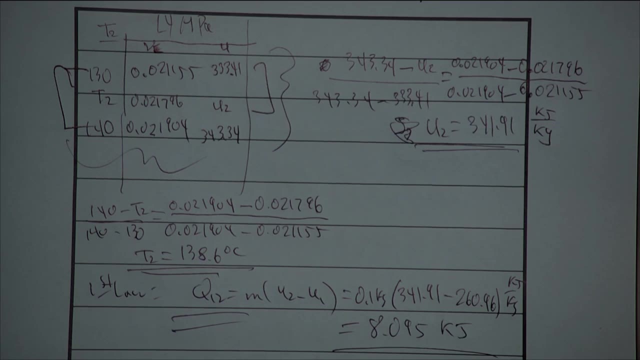 to 343 than to 333.. And we find that as well right That the internal energy equals about 342.. So you know, the interpolation at least appears that we've done it properly. We have heat transfer at the end here. 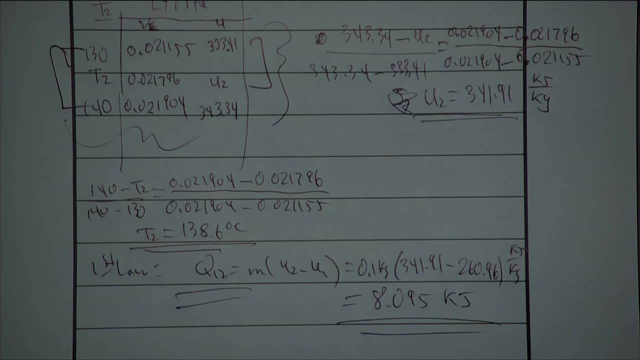 We find that the heat transfer is a positive number, which implies heat is being added. Does that make sense? Well, that should also make sense. Some energy is being added into this. Some energy is being added into the system And that's causing the temperature. 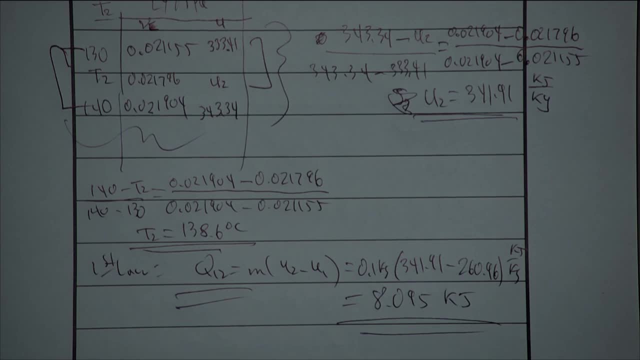 and the pressure to both rise. Well, there's no work, There's no kinetic and potential energy. So where does that energy come from? I mean it has to be heat, right. So the fact that you have a positive heat transfer term means. 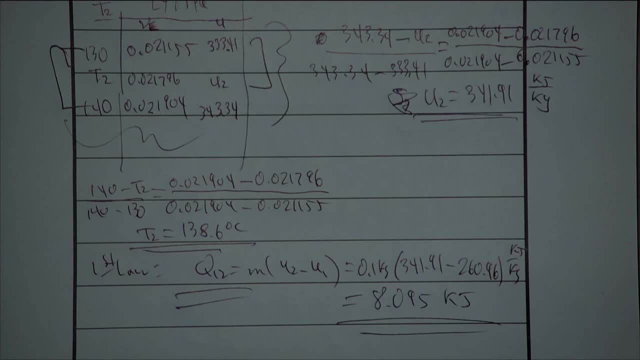 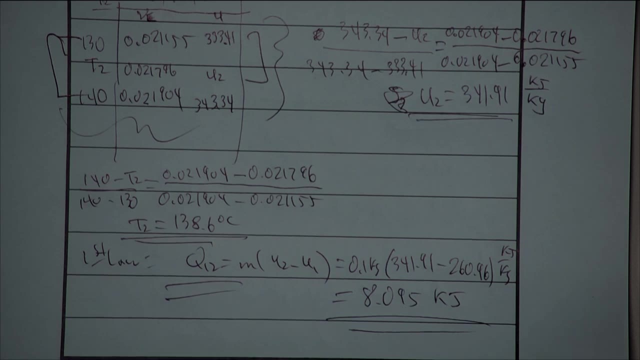 that you have heat added to the system, which is consistent with the nature of this problem. So the numbers look good, The signs look good. That's this problem. Yeah, So you could call this isochoric, even though it's not. 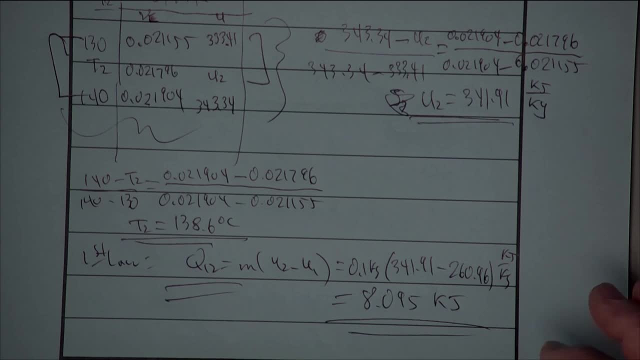 Yeah, the word isochoric would just mean that you have a constant volume process. So I mean I could have said, instead of the sealed rigid vessel, I could have just said you had .1 kilograms of R134A at these conditions undergoing an isochoric process. 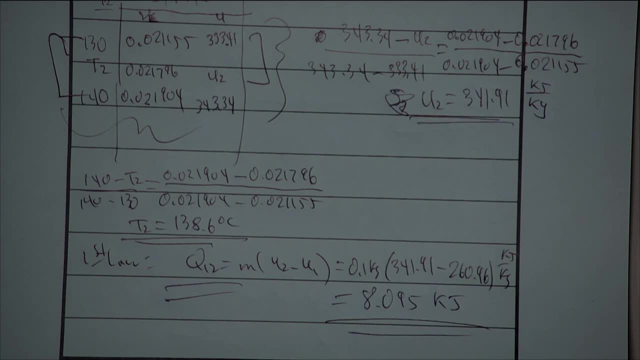 until it reaches a final pressure of 1.4 megapascals. You could look at that and say: well, okay, it's a constant volume process. The only thing is that that doesn't specifically tell you that it's a constant mass process. 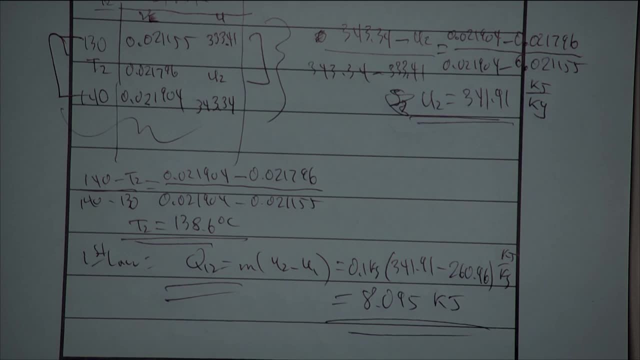 It still has to be a sealed tank. So yeah, if one is told that it's isochoric, you should also be told that it's a closed system problem or a constant mass problem or something like that. So all that should be given to you. 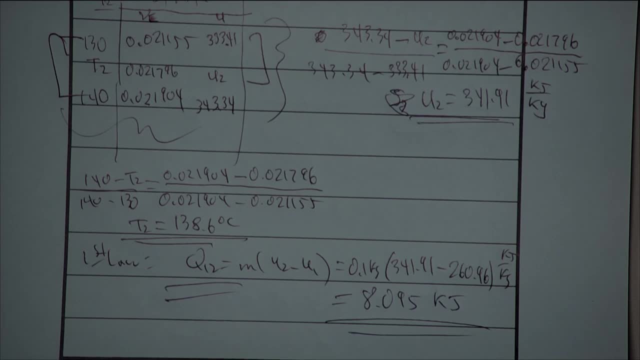 These problems are obvious, right? They're all from Chapter 4.. They're all closed system problems, So there's no real question as to how to solve these problems. But on your final exam, I'm not going to tell you. this is a. 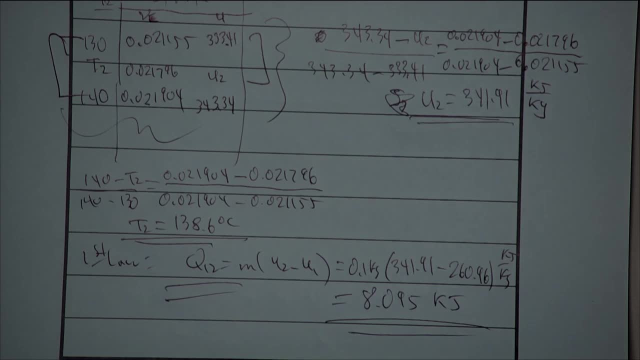 closed system problem. I'm just going to tell you the problem. You're going to have to look at that problem and say, oh, I recognize this, This is a closed system problem, and solve it using the appropriate method. So same thing for this problem. 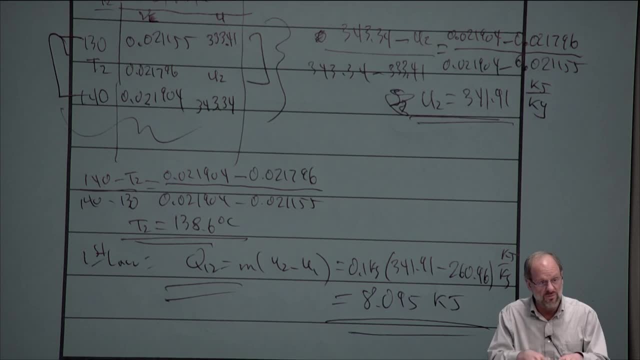 Same thing with the homework right. The author of your textbook identifies homework problems by section of the book, So it tells you what type of problem it is before it even gives you the problem. So there's that big clue as you solve those problems. 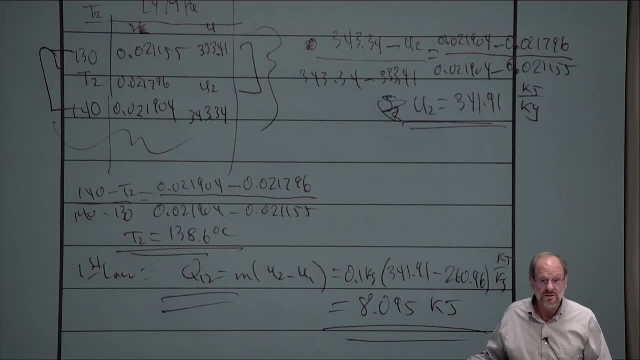 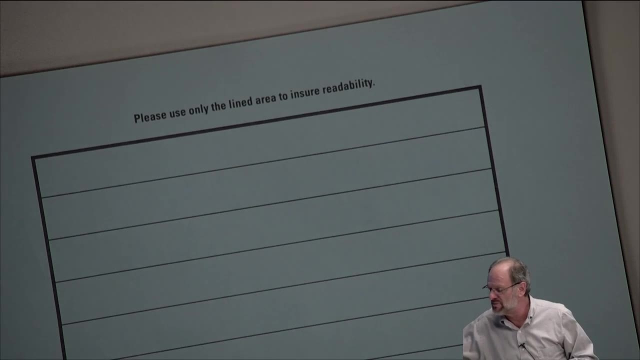 Again, I'm not going to do that on your exams. Any other questions? All right. So that was one problem And really this is about the simplest that these problems get. Now you might look at that problem and say, well, 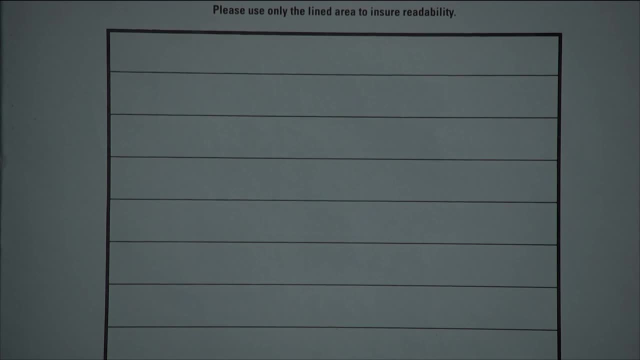 that sure doesn't seem very simple, But it wasn't hard. I mean, each step we went through is very similar to what we've already been talking about. right, We looked at some basic equations, We looked at some data, We've gone through some math, some units. 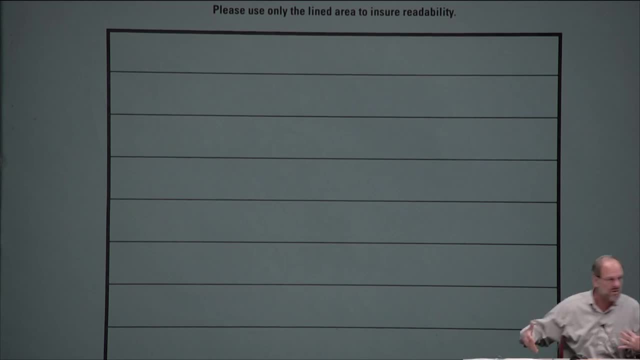 And we've come to the conclusion that there's a final temperature, There's some work, There's some heat. This is simple, because it's a nice, sealed, rigid vessel. There's no work, no kinetic and potential energy. We could certainly have problems that are a lot more complicated. 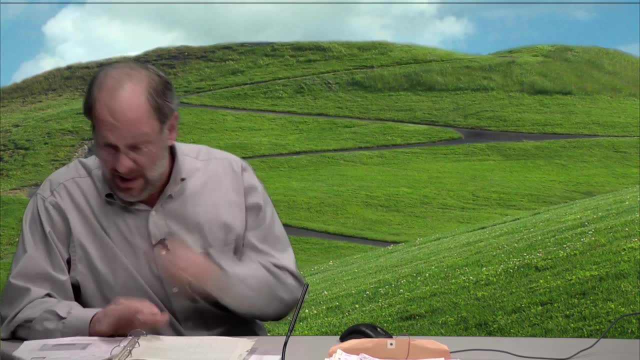 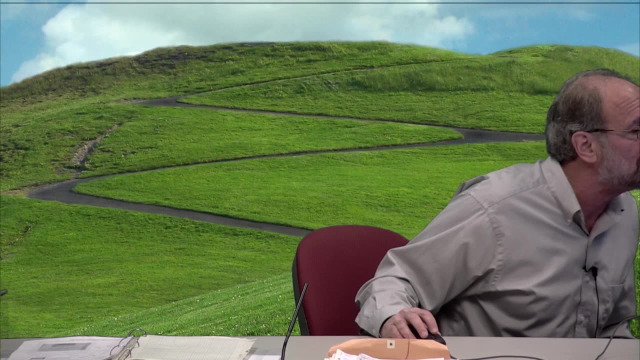 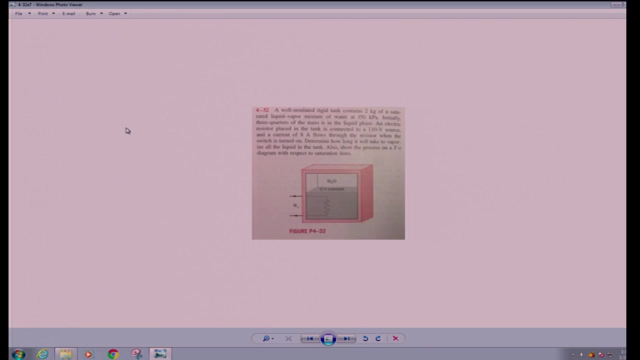 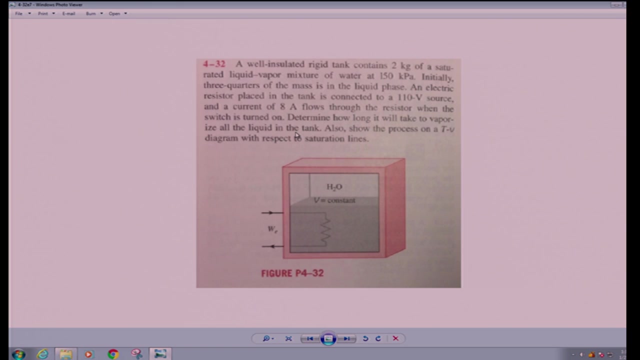 So let's go through another one which is more complicated. This one's actually from the 7th edition of this textbook, So this is actually problem 4-32, but from edition 7.. So you should write this down, because I don't believe. 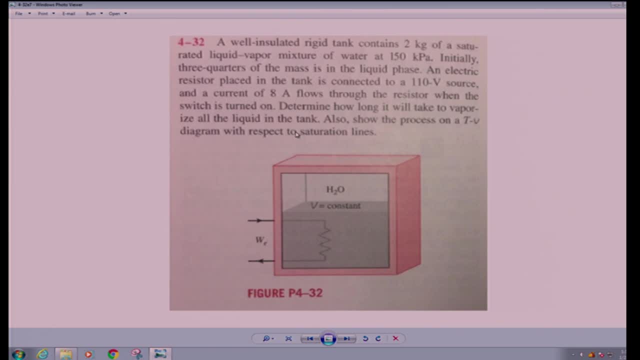 that most of you have access to edition 7 of this book, So let me just read this. I'm going to read this to you and explain it, And then we'll go through the whole process. All right, so this one's a little bit similar. 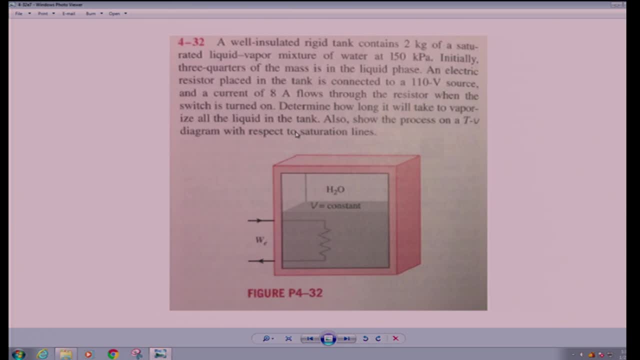 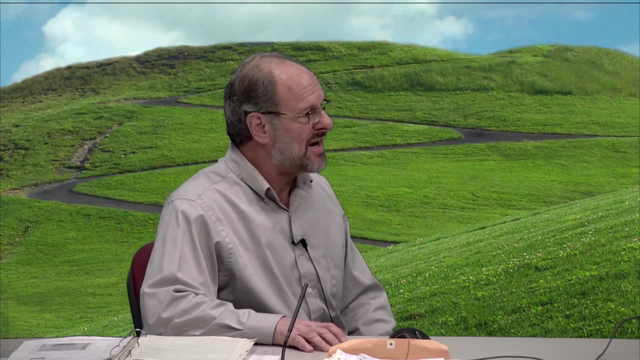 and a little bit different. First of all, it tells you that you have a well-insulated, rigid tank. Well-insulated, by the way, is a clue as to something. It contains 2 kilograms of a saturated liquid vapor mixture of water at 150 kilopascals. 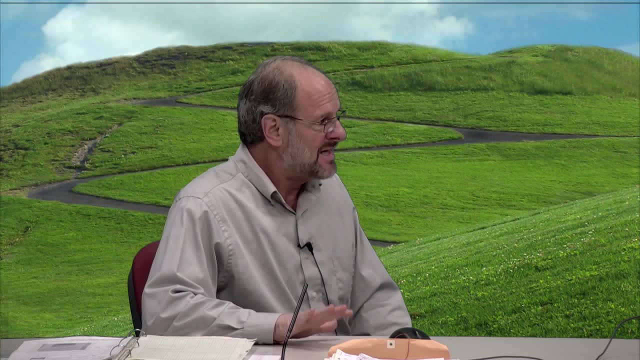 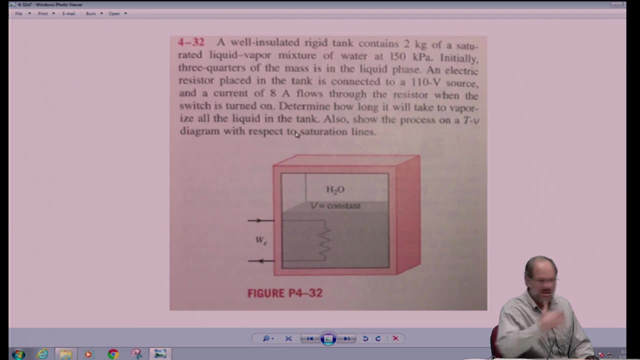 So they're telling you that it's a two-phase mix. at a given pressure, It says initially that is at this state, three-quarters of the mass of water And three-quarters is in the liquid phase, which also tells us something about the mixture, right? 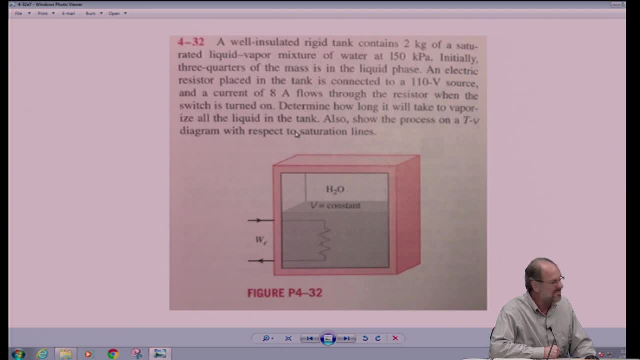 If three-quarters is in the liquid phase, that means one-quarter is in the vapor phase. Does that mean that the quality is 25%? So indirectly they've given you the quality. Now it says an electric resistor is placed in the tank. 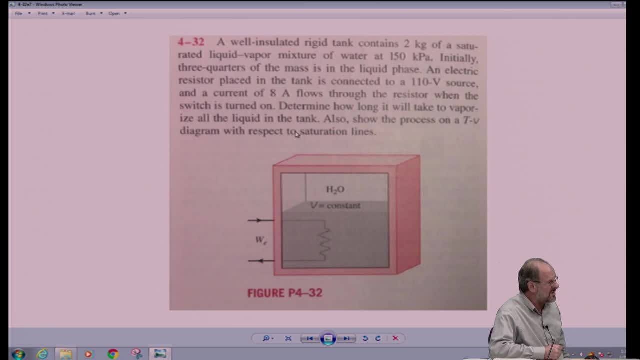 and it's connected to a 110-volt source. Eight amps of current flows through it when the switch is turned on. So it basically is asking you how long will it take? In other words, how long do you have to have that switch on in order? 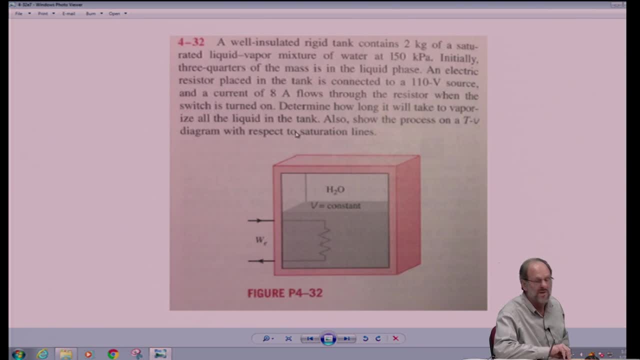 to vaporize all the liquid in the tank. You start with a two-phase mixture. You're adding electrical work And eventually you'll get to the point where all that water turns into water vapor And at that point where it just turns into water vapor. 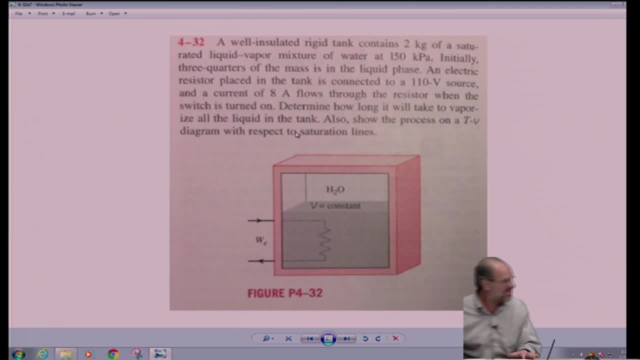 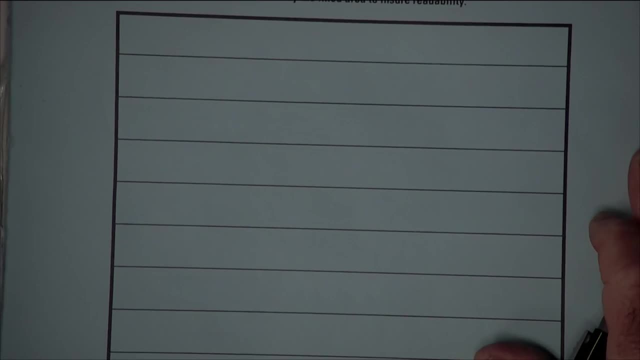 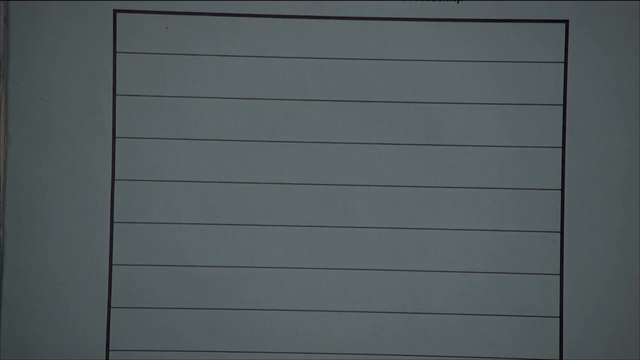 that's when the process ends. So they're asking you how long that whole process will take. Now, this one is by no means as obvious as the previous one, if the previous was obvious. So again, you might want to rewrite the problem. maybe rewrite it in terms: 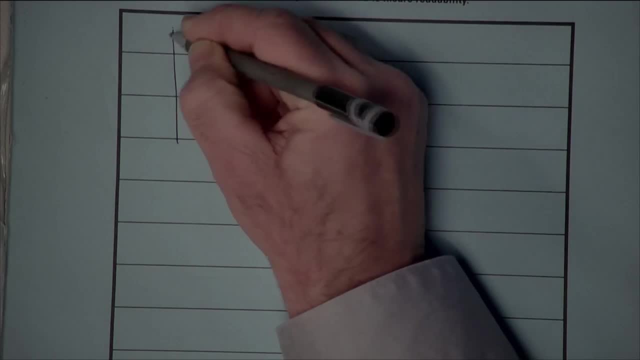 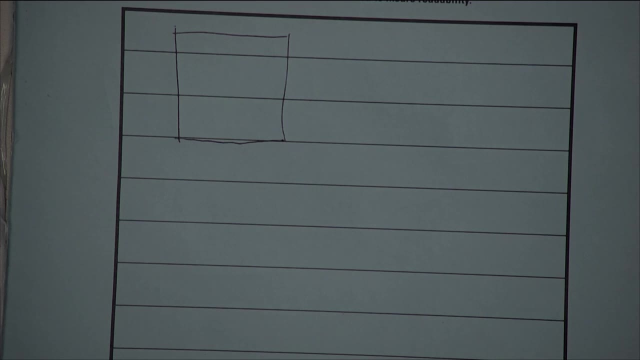 that make more sense to you. assuming that's already been done, Let's just create our sketch. So, again, it's a sealed, rigid tank. So I'm just going to show it as a closed tank like this. We know that it's well insulated. 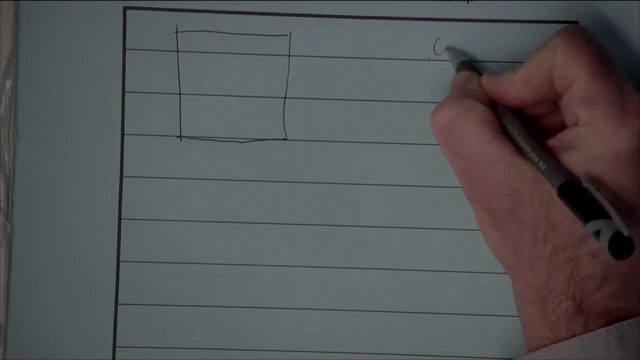 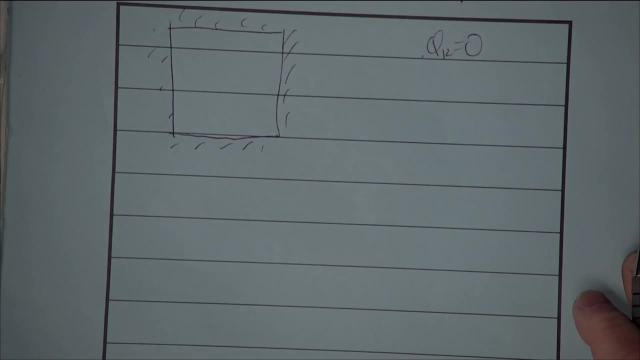 So again, well insulated is the book's way of saying no heat transfer. Okay, You can show this with insulation all around it, But whenever the problem is well insulated, it's no heat transfer, adiabatic same word. 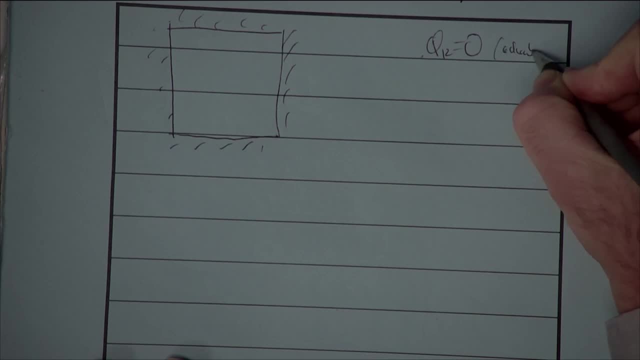 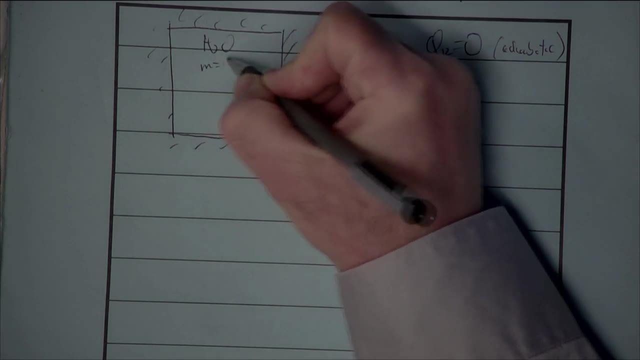 Adiabatic means no heat transfer, And that's given in the first statement of the problem. Okay, Now we're given that it's water, We're given that the mass is 2 kilograms, We're given that it's a two-phase mix. 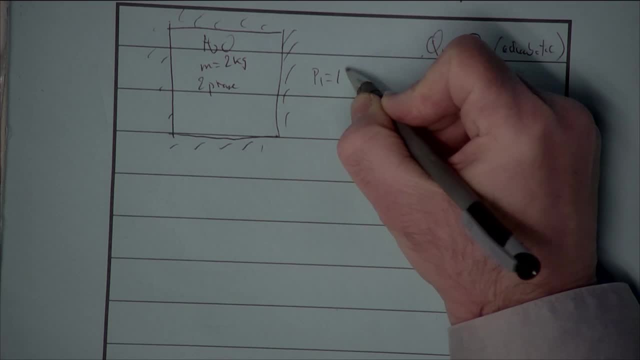 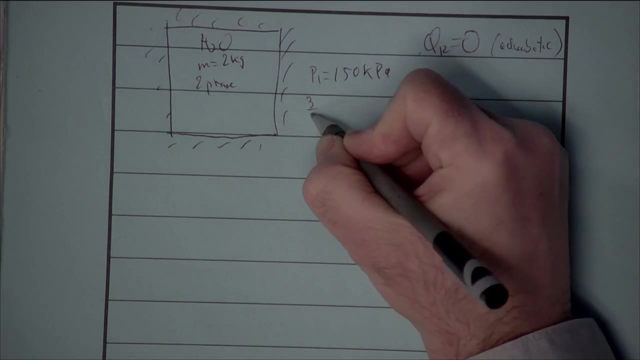 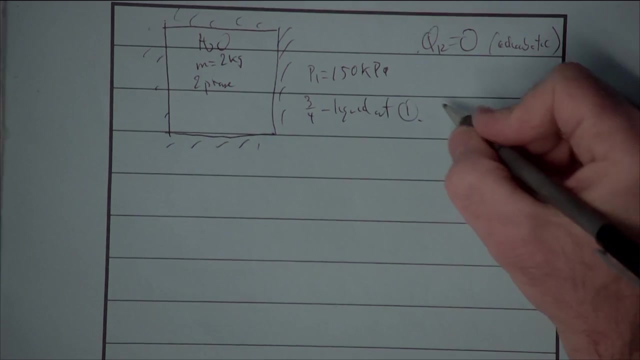 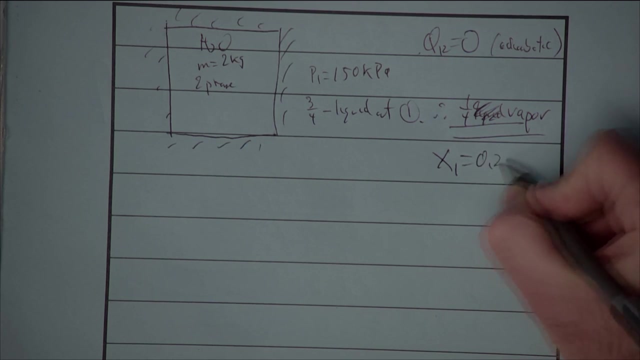 And we're given that the initial pressure, anyway, is 150 kilopascal. Okay, Now it says three-quarters is liquid at one. Therefore one-quarter is liquid, I'm sorry. Therefore one-quarter is vapor And therefore the initial quality, as we call it, is 0.25. 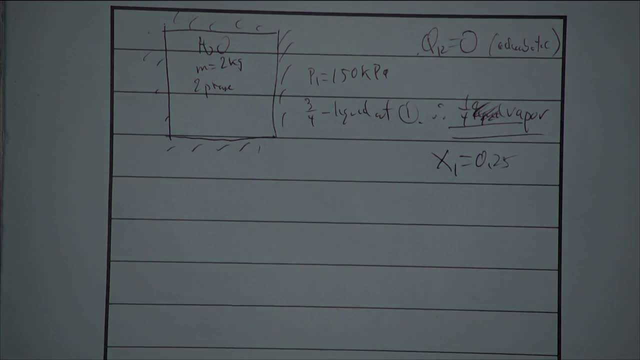 So that's also given to us in the problem statement. By the way, you've got to be really careful. This says three-quarters of the mass is in the liquid phase. It doesn't say three-quarters of the volume is in the liquid phase. 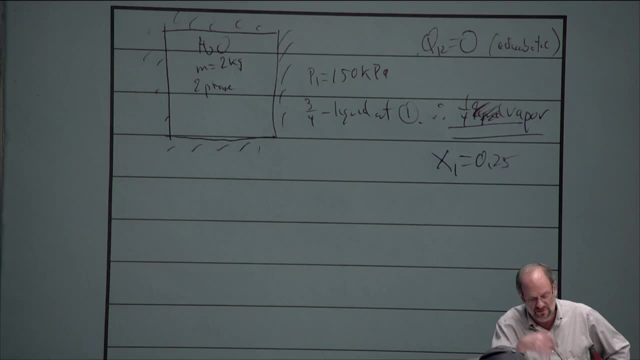 Some problems. you'll be given a volume fraction instead of a mass fraction, And volume fractions are definitely not the same as mass fractions. Okay, So you know, keep in mind that the vapor takes up a lot more physical space than does the liquid. 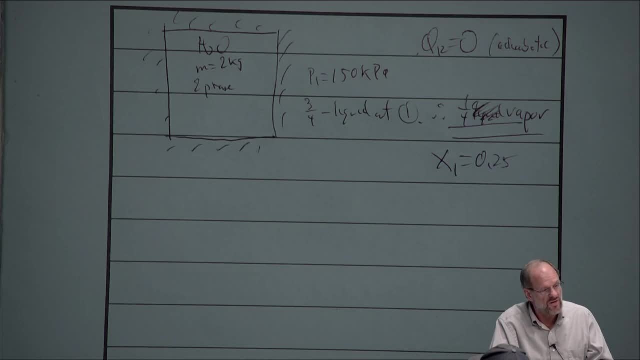 If you have something that's got a 25% quality, in other words 25% mass, you're going to have a lot more space. I will tell you that this drawing is not accurate. You're probably going to have 90% or more vapor volume, just. 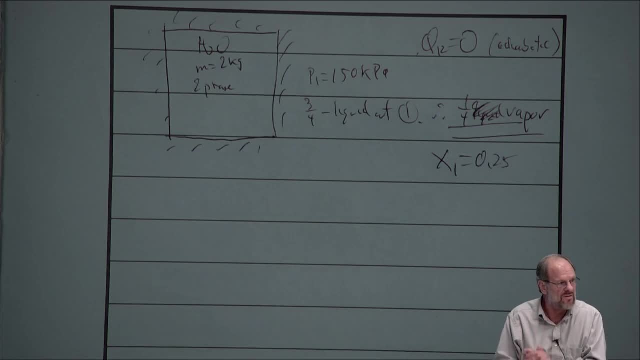 because the specific volume of the volume fraction is so much greater than the specific volume of the liquid fraction, right? So that's not really a two-scale diagram, even the one that's in the book. All right, So we know the quality. 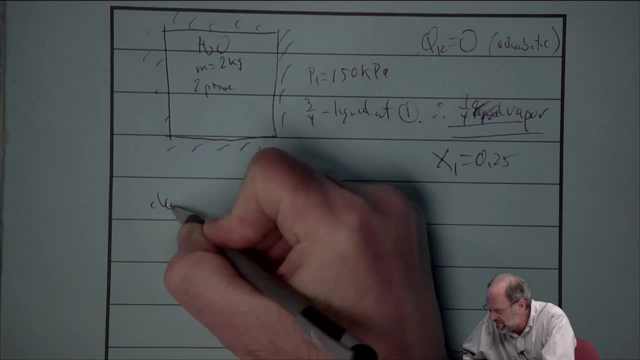 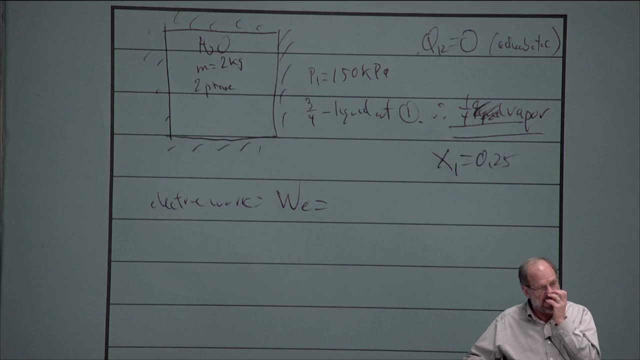 Let's move on. We have an electric resistance heater, So that means we have some electric work, And the electric work is something you'll actually have to find Now. I did mention that I'm generally not going to give you problems that have other forms of work. 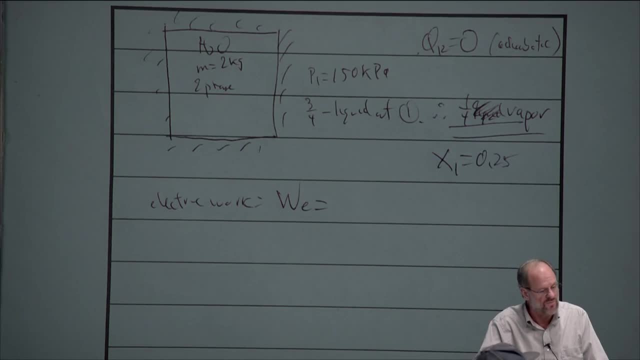 This is one of those other forms of work. If you have a problem with one of these other forms of work, you would have to be given the equation. If you go back into either section 2-4 or 2-5, it talks all about electrical work. 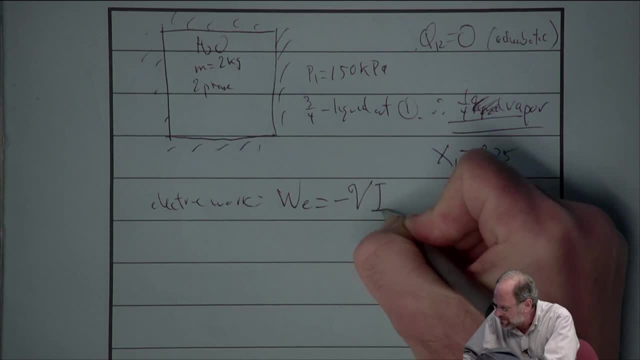 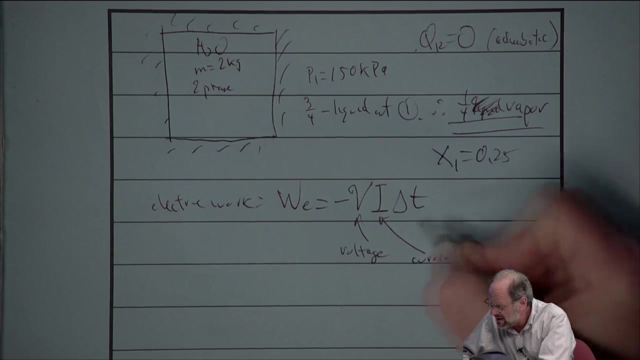 And the electrical work is a very simple equation. It's just this one. Now here, this is the voltage, And the voltage is going to have the units of volts. I is the current And delta T is just the timeframe. So we're definitely going to have to use this equation. 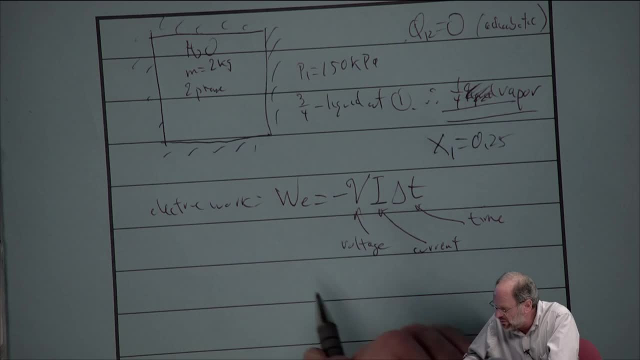 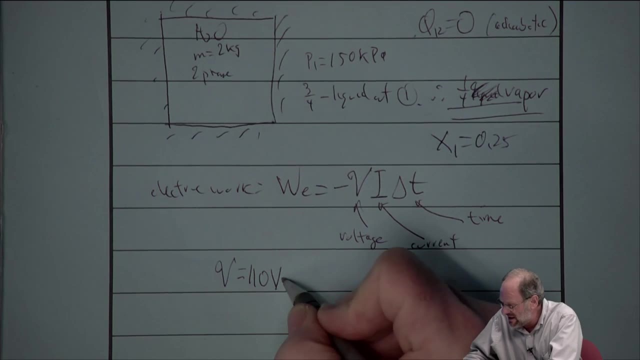 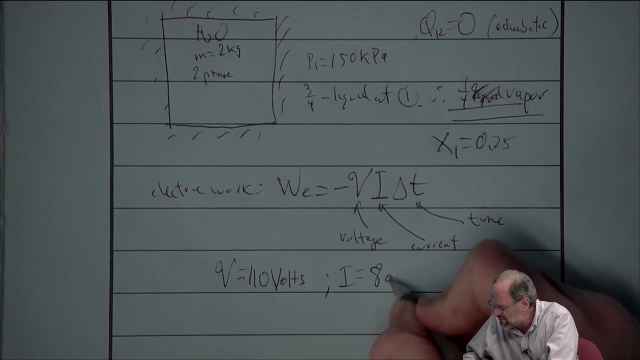 for electrical work in solving this problem. We are told, again writing down all the information, that the voltage is 110 volts. This V is the unit of volts And we're also given the current. The current is 8 amps. 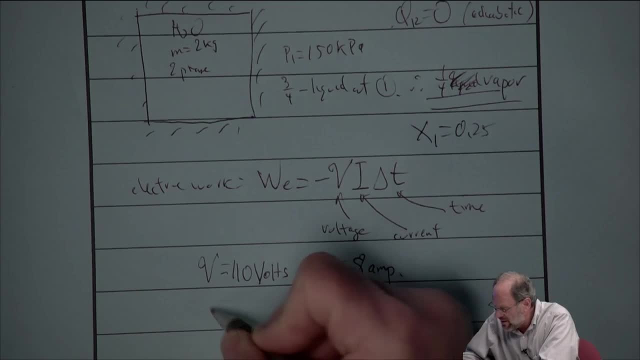 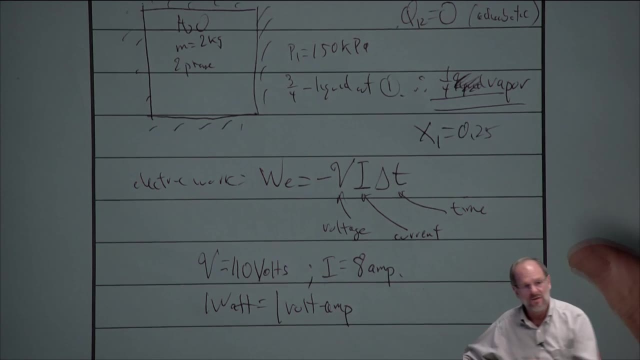 So this is the information we have. One thing that's also worth noting: one watt equals one volt amp. Okay, So the product of voltage times current is power in watts, So this electrical work will have the units of watts. So maybe over here. 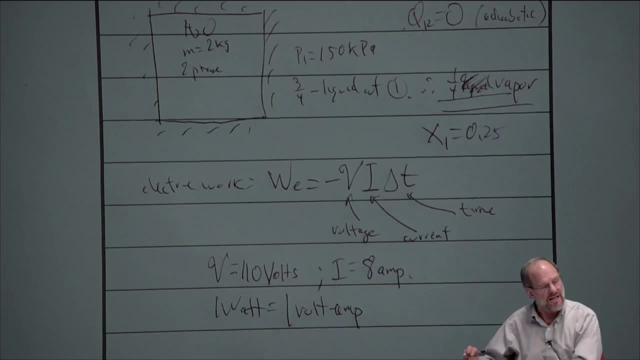 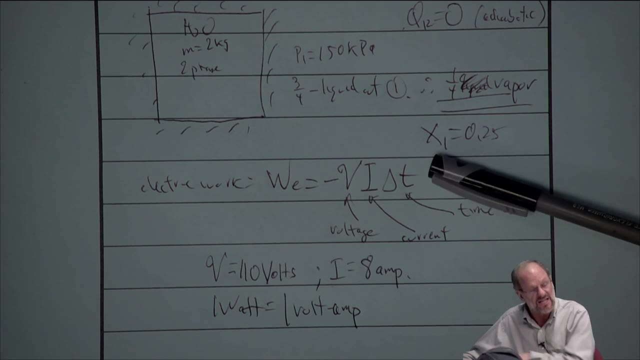 Well, I take that back, The voltage times. the current is going to be watts, which is joules per second, And then we multiply it by time. The seconds cancel, so we end up with joules. So watts is certainly the appropriate power units. 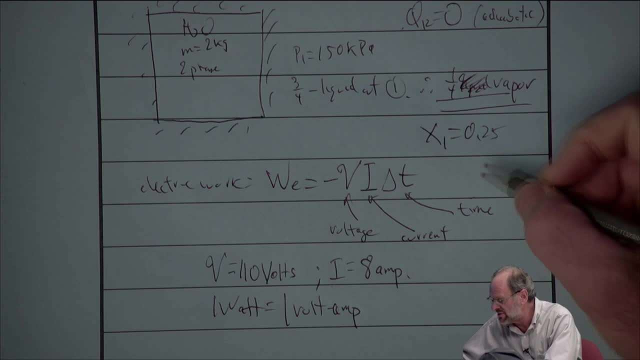 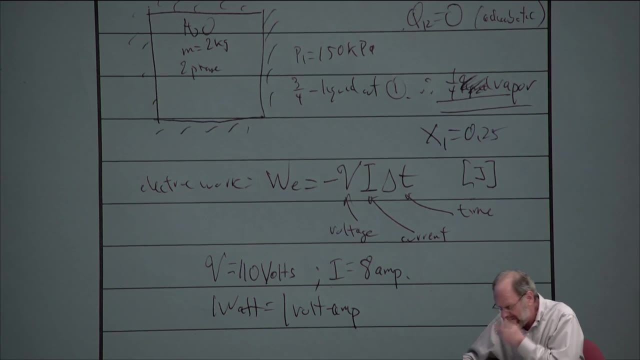 When we multiply by time, we get joules or kilojoules. So this is in the SI system, So this is going to be in joules or kilojoules. Now let's just continue reading the problem: The switch is turned on. 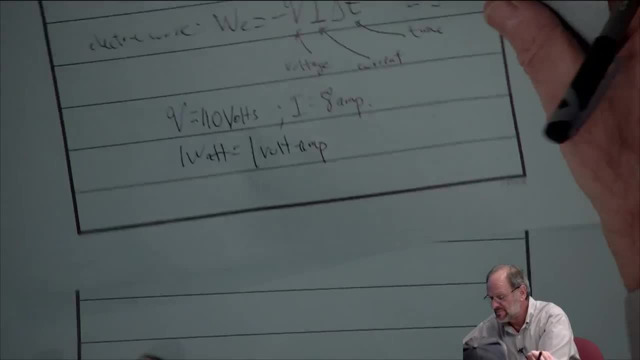 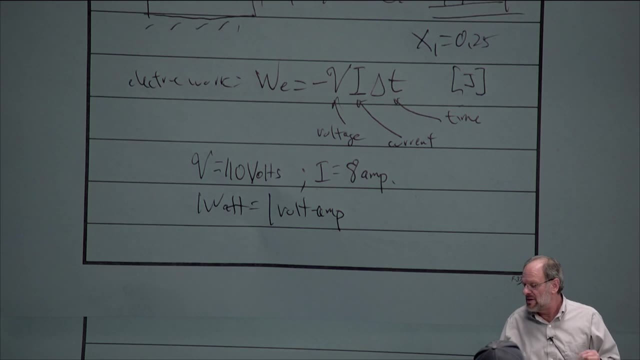 How long will it take to vaporize all the liquid in the tank? You said it's negative because it's doing work to the system. I didn't mention that, but that's true. Keep in mind that our sign convention for work is different than for heat, right. 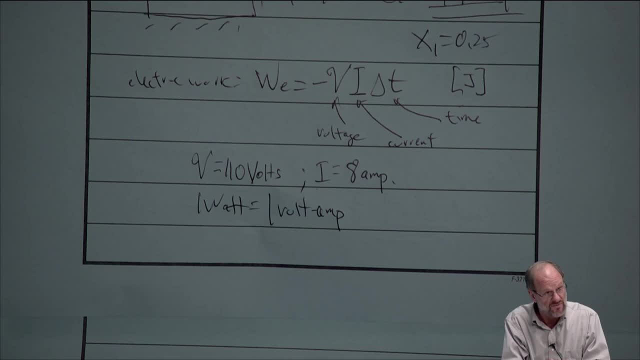 Work added to the system is considered negative. Work added or done by the system is considered positive. Whenever we have electrical work, we're actually doing work to the system. You know current is passing through the resistance coil. Work is coming into the system. 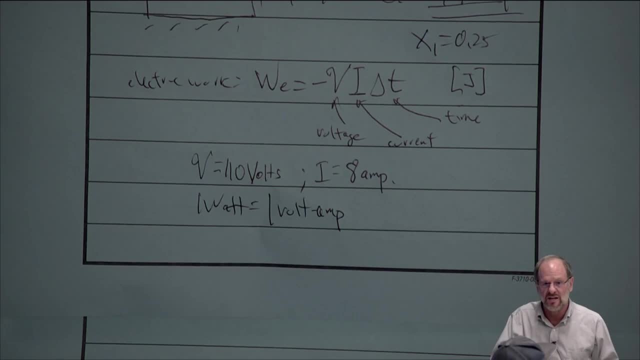 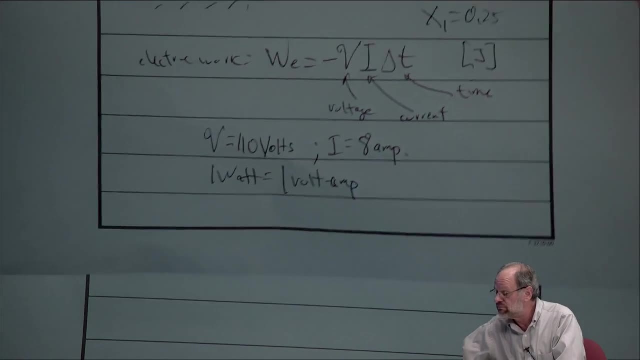 That's considered negative. So that's why we have the negative sign and that was a good observation. I should have mentioned that before A couple other things we know. So let's see, We're trying to find delta T, right? 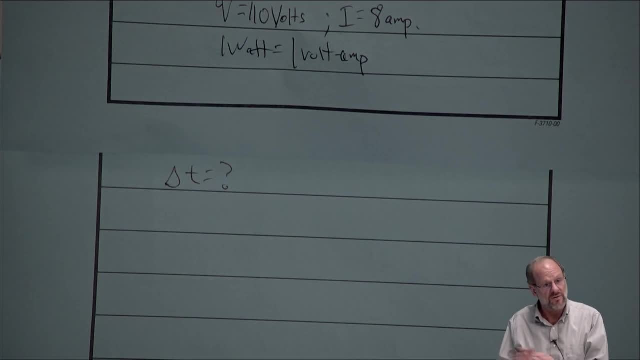 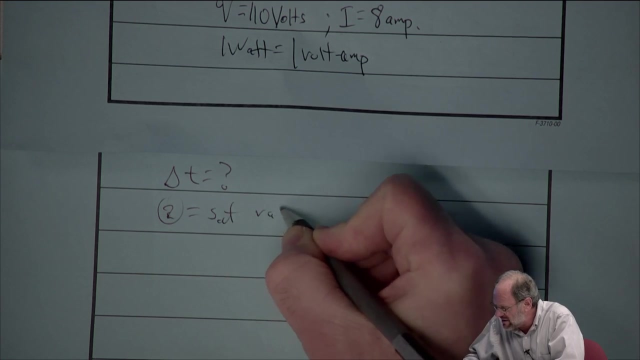 It's asking us how long it's going to take for all the liquid to vaporize. But that gives us another clue. When it says that all the liquid is vaporized, then that tells us that the final state is a saturated vapor. So 0.2 is a saturated vapor. 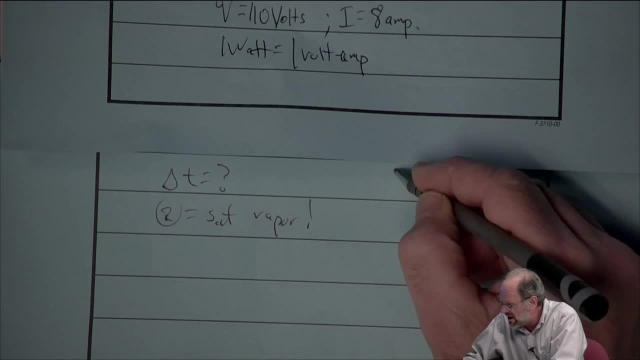 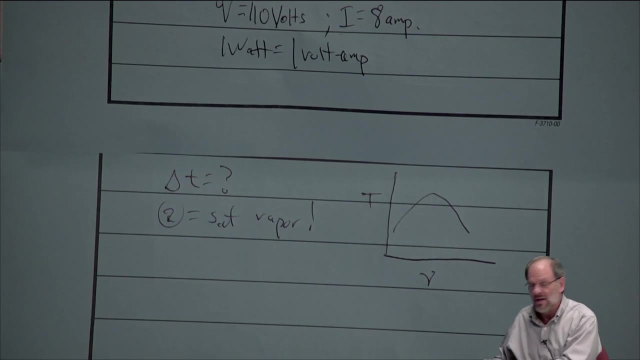 Okay Now maybe this will be a little more obvious if I show this on the appropriate diagram. And again, I could show this on a TV diagram relative to the saturation lines. If we're starting with a high quality two-phase mixture, we know we're going to be over here somewhere, right? 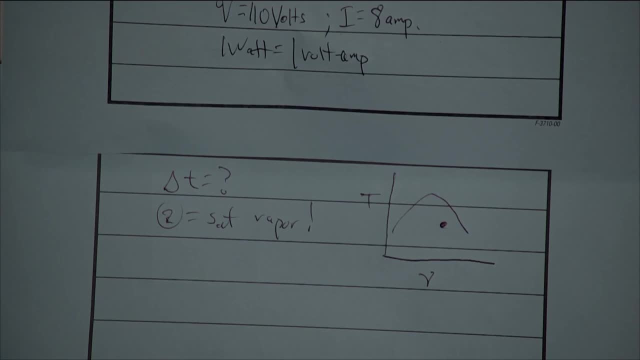 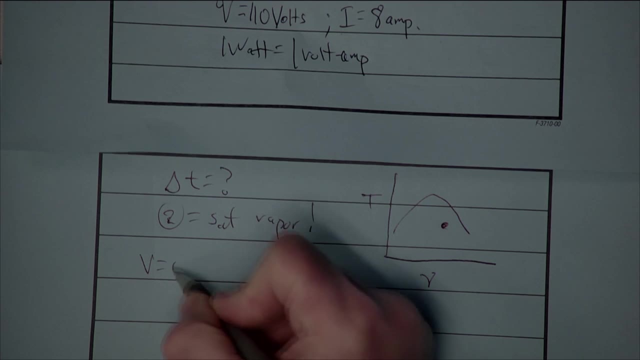 And we know, like the diagram, that we're going to be over here somewhere, right? But the previous problem, that this is a constant volume process. it's a sealed rigid tank. there's no change in mass, there's no change in volume. so I'll put: V is equal. 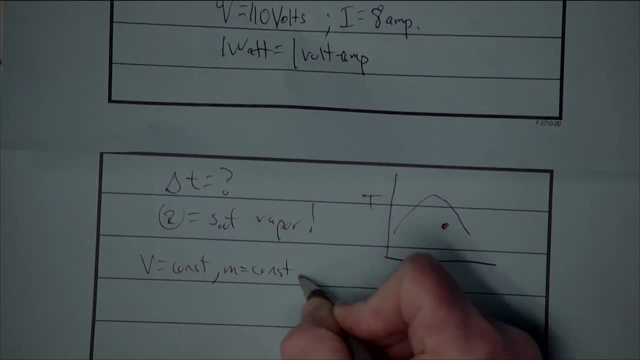 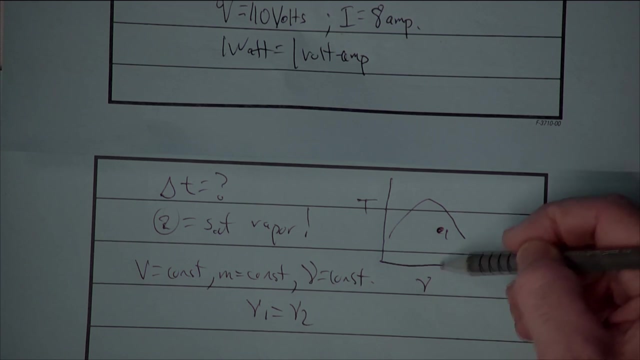 to a constant. M is equal to a constant and therefore the specific volume is equal to a constant. So V1 equals V2.. So that's more information we have. If this is state point one on the diagram, and I know that I'm moving along the constant volume line- 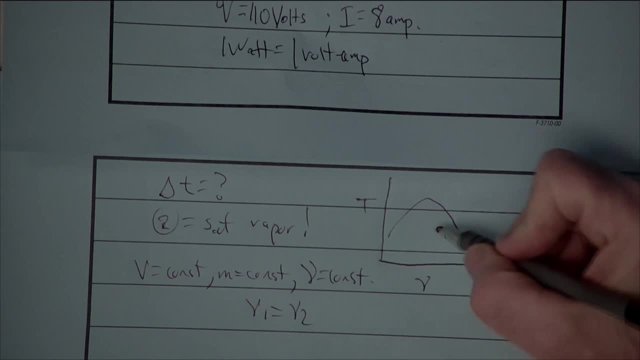 that means I have to be going vertically, And since I know that the point where the last drop of liquid has finally turned into vapor is when I finally hit that line, that is point two. It is a saturated vapor, Some of you might have said. well, 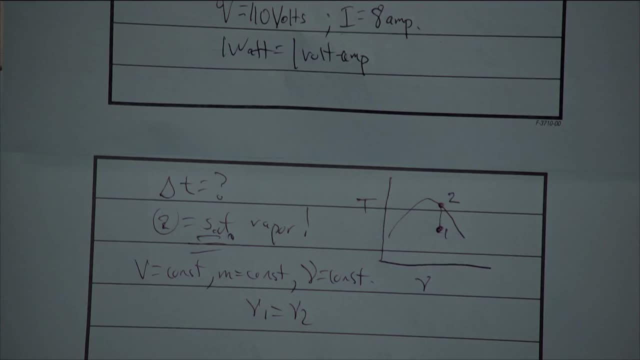 how do I know it's a saturated vapor and not a superheated vapor? Well, it's because of the problem statement It says: how long will it take to vaporize all the liquid? All the liquid is vaporized for the very first time. 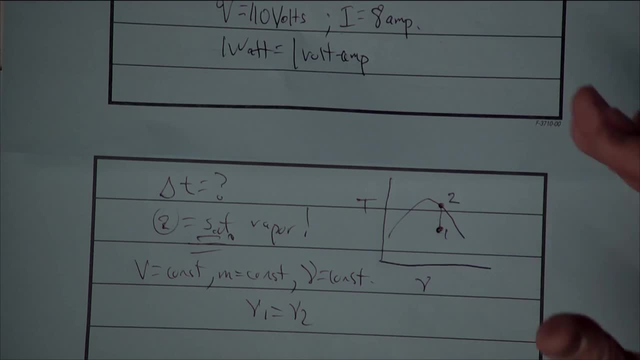 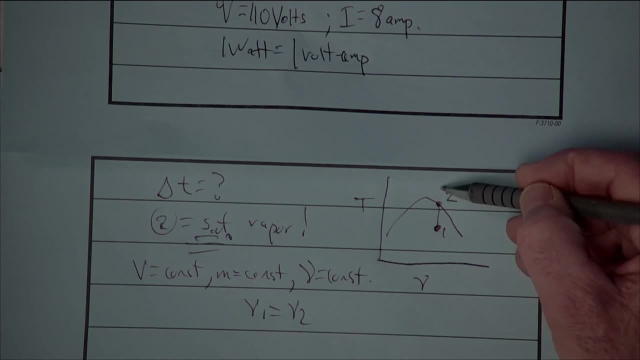 when you finally get to the saturated vapor line, You could continue adding heat or electrical work and you could start superheating, in which case you go above point two. But that's not how long it will take to vaporize all the liquid. 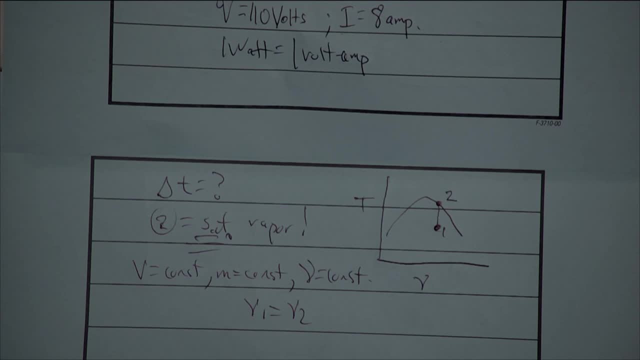 That's how long it will take to vaporize all the liquid, plus the extra time you've spent leaving the heater on because you forgot to turn it off. So make sure you understand the problem right. Point two is definitely saturated vapor. So now we're pretty much done setting up the problem. 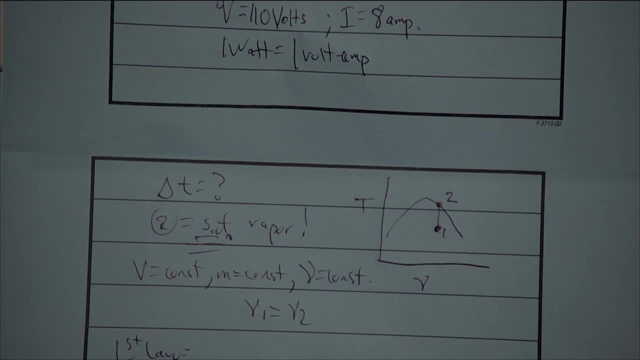 Let's go to the equations. So we need the first law: heat transfer Equals change in internal energy- and these are supposed to be u's Again- plus the change in kinetic and potential energy, and then plus the work. Now we're not quite done with this. 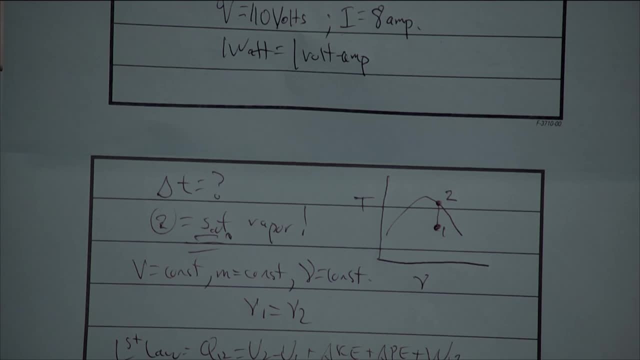 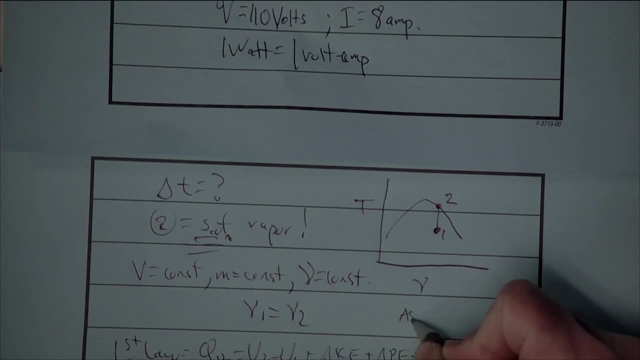 We haven't made our assumptions yet. We can make the same kind of assumptions that we did in the last problem, though, can't we? There's no velocity associated with this problem, So I could assume that, therefore, there's no change in kinetic energy. 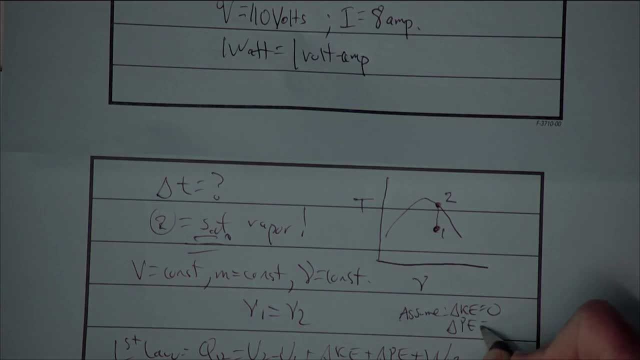 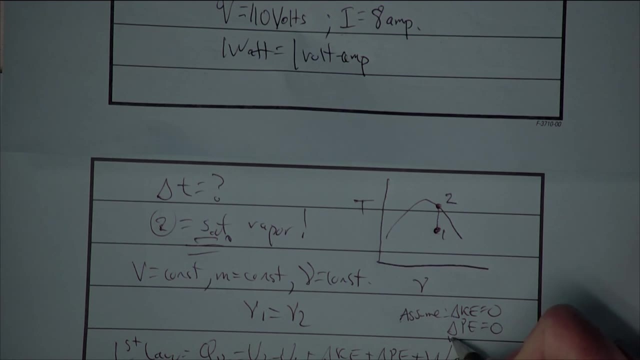 It's just a tank, so there's no height change. That's associated with the problem, So we know there's no change in potential energy. We would also note that there's no boundary work. right, That doesn't mean there's no work. 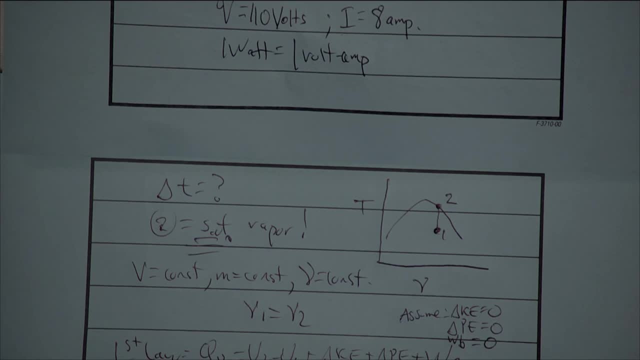 There's clearly electrical work, but there's no boundary work. So there can't be any boundary work because there's no volume change again. So no volume change, no boundary work. So kinetic energy goes to zero, Potential energy goes to zero. 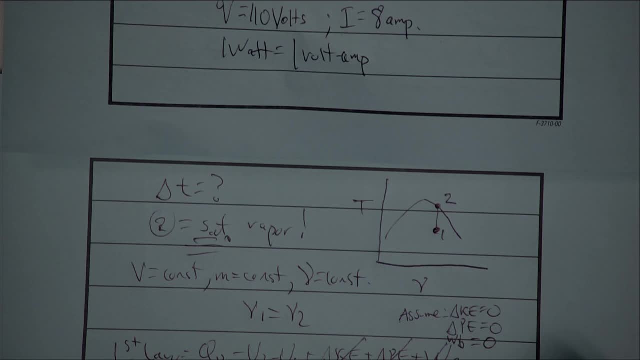 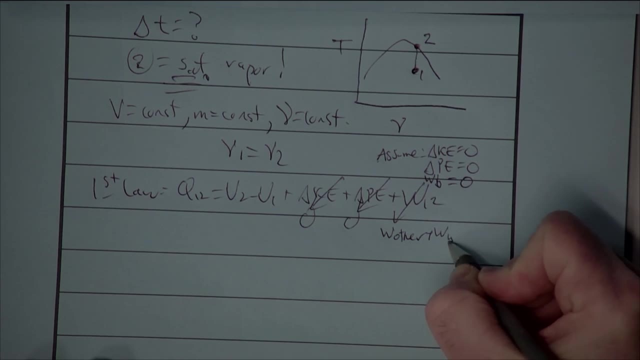 The work from which we're going to be doing this, we're going to be doing this, we're going to be doing this, and the work from one to two doesn't go to zero. It's other work plus boundary work. The boundary work goes to zero. 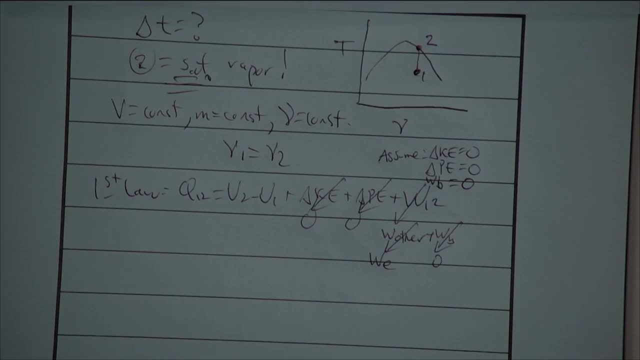 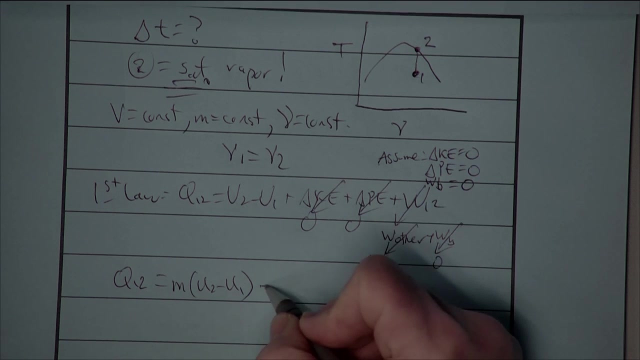 but the other work is the electrical work right. So we get heat transfer equals change in internal energy. We'll do like we did in the previous problem: Let's just show this as mass times, the change in the specific internal energy And then plus the electrical work, right. 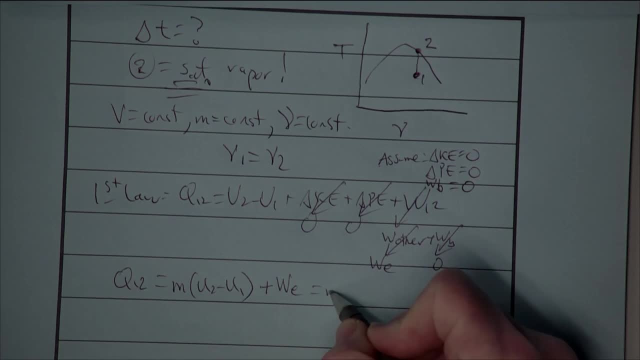 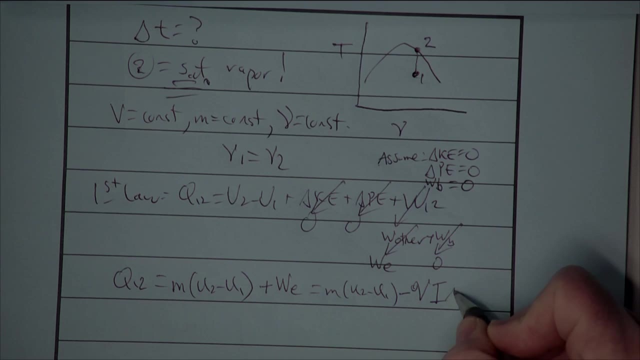 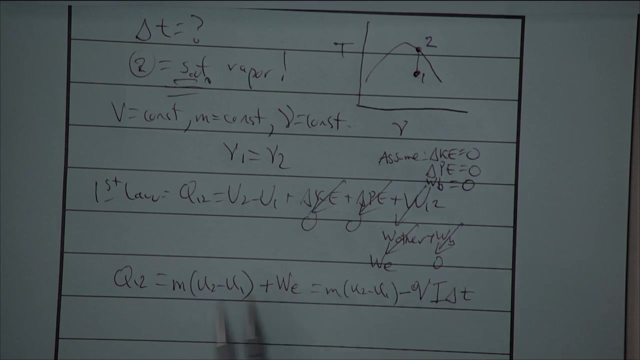 So this is our equation. Let's rewrite it: Mu2 minus U1 and then minus voltage, current times time. So this is the equation. Oh, and I forgot one other thing. I mean, I didn't forget it, I just forgot to cancel it out. 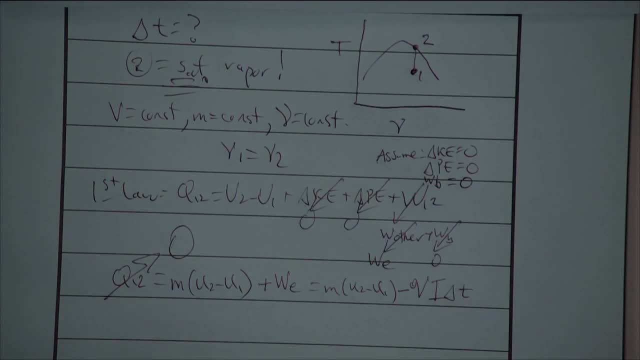 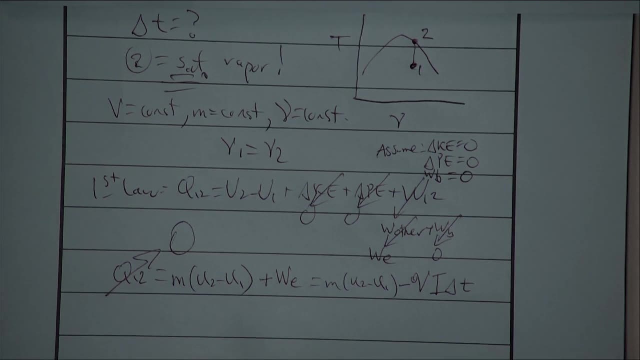 We already noted at the very beginning that there's no heat transfer. right, It's well insulated, So there's no heat transfer, So the whole thing equals zero. So we can now rewrite it one more time. We get voltage times, current times. time is then equal. 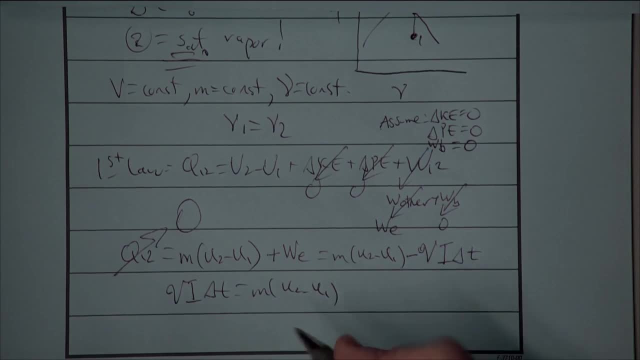 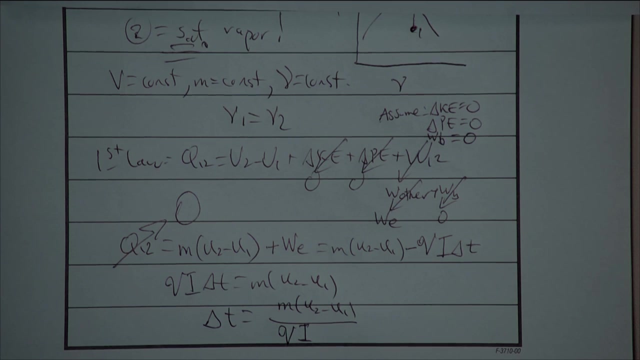 to the change in the internal energy, And remember that it's the time we're trying to solve, for So delta T is the mass times, the change in internal energy, divided by the voltage times, the current. So now we have to ask ourselves: can we solve the problem? 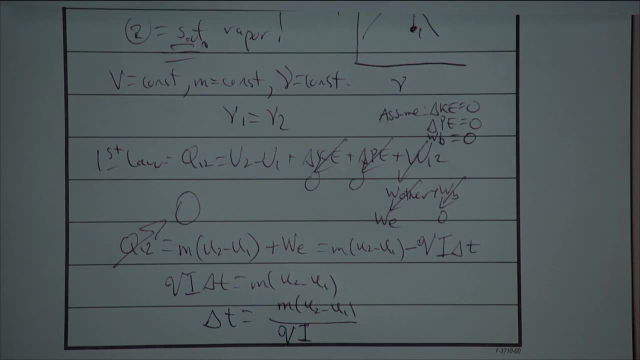 OK That there's nothing more we can really do here. We know the voltage because it's been given. We know the current because it's been given. We know that we have the mass, We know that we have the initial pressure and we have the initial quality. 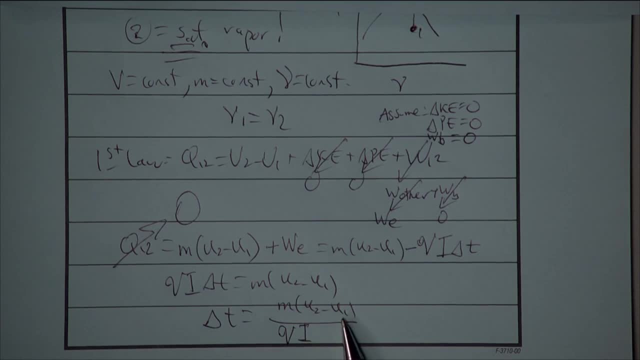 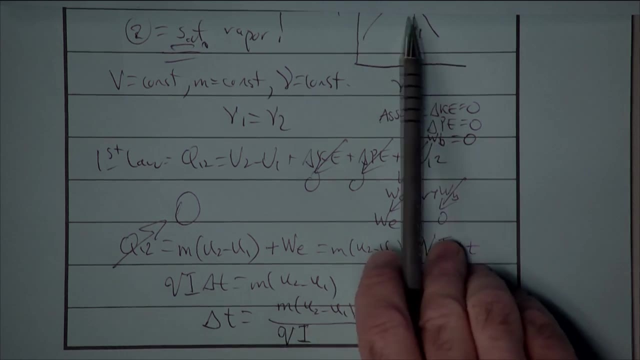 So two properties. So we can find the initial specific internal energy And we know that we have the final. well, we know the final internal energy. So the final, one final phase. we know there's a saturated vapor, so essentially the final quality. 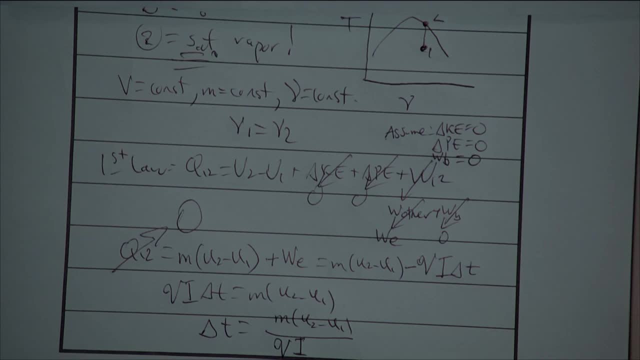 is 100% or just one. and we also know that at the final state the volume is the same as at the initial state. so we know the volume and the quality. so again we have two properties, I should really say specific volume and the quality, that is that it's a saturated vapor. so we have the final state. so the discussion. 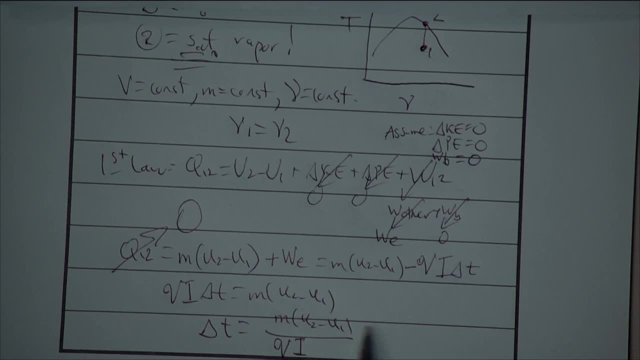 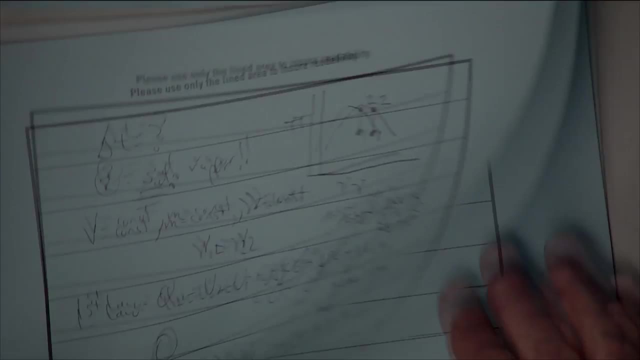 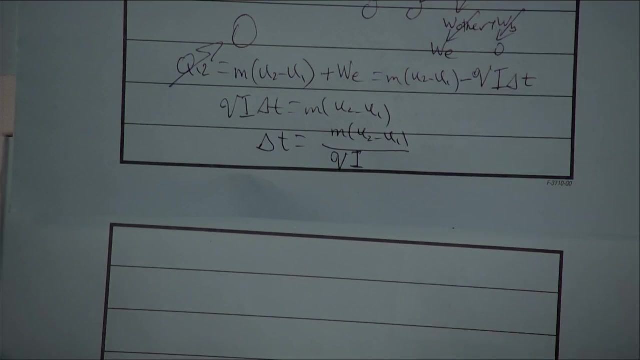 isn't hard right. we've got some equations, we've recognized that we have the ability to find all the data, so now it's just a matter of finding all the data. so let's do that, and we'll just start at state point 1. yes, oh, simply because we were told that it's a well insulated leak. well insulated is just. 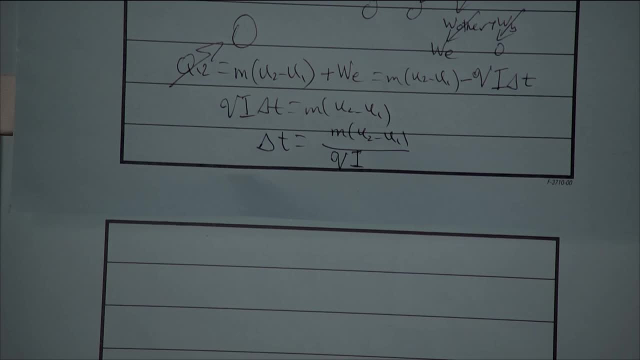 the author's way of saying no heat transfer. sometimes the author uses the word perfectly insulated, sometimes it just uses word insulated, but whenever they're telling you that it's insulated, assume no. all right, so back to the beginning. we'll start at state point one and we know the 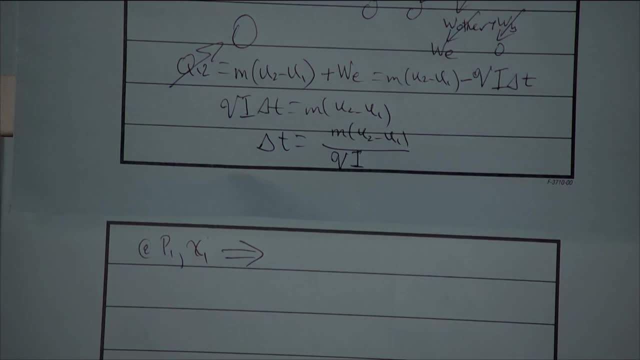 pressure and we know the quality at one, so we know that it's water. we know pressure and quality, so that means we go to table a5. there's no test to make here, so I'm going to take this down now. all right, I'm just gonna go to the property table. 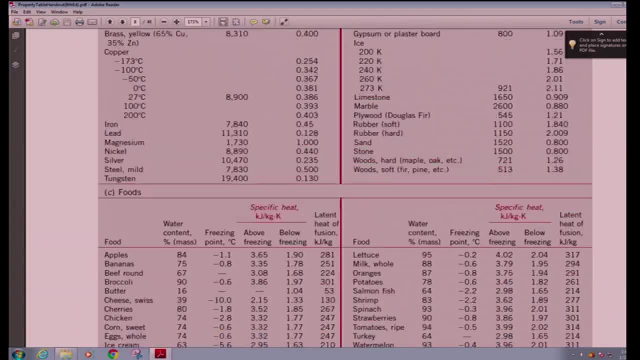 all right, so we've got water. we have pressure, so we're gonna go to table a five. all right, so we're gonna go to table a5. all right, so we've got water, we have pressure, so we're gonna go to table a5. and here's table A5, and the pressure is given. 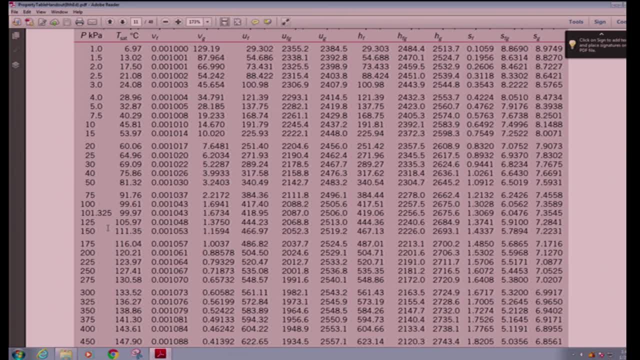 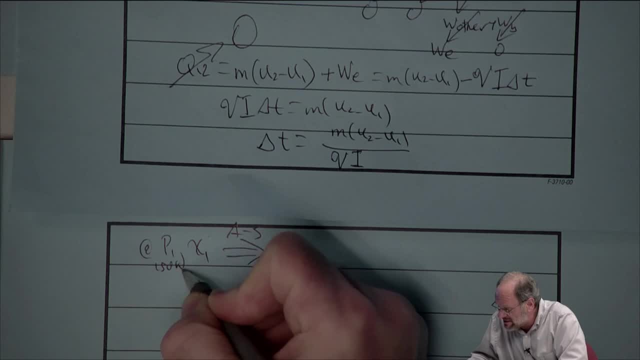 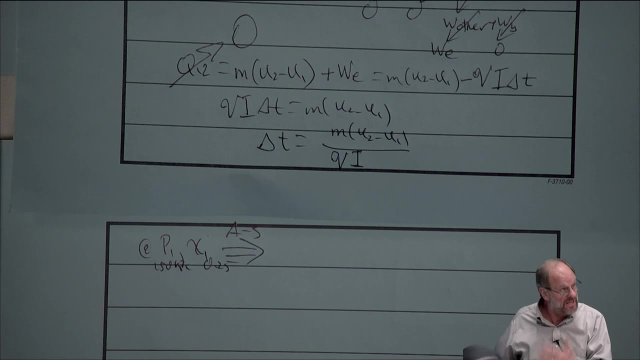 as 150 kilopascals. so I think that's right. yep, at 0.1.. So at 150 kilopascals and at a quality of 0.25, we find whatever information we need, And we're really looking for two things right. 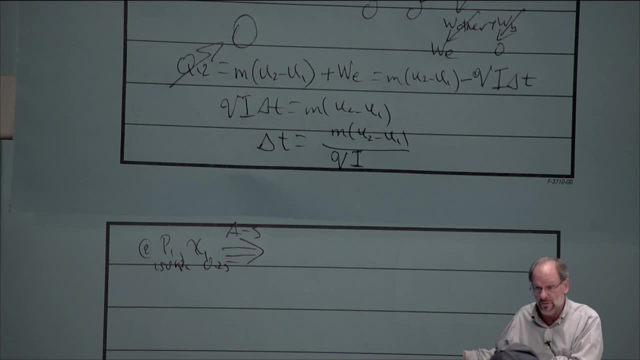 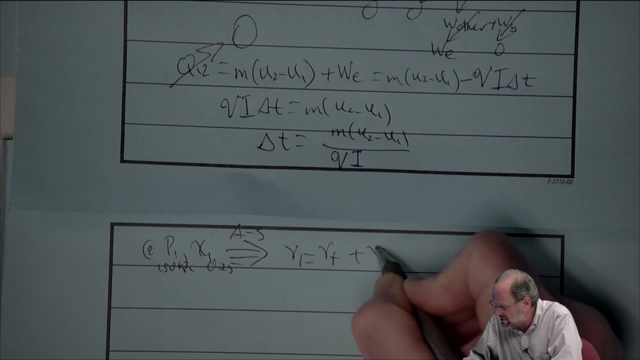 We need the specific volume because V1 equals V2, and we need V2, and we need the internal energy. So let's just start with the specific volume. So V1 is VF plus the quality at 1 times VFG. So remember, this is the equation we would use whenever we 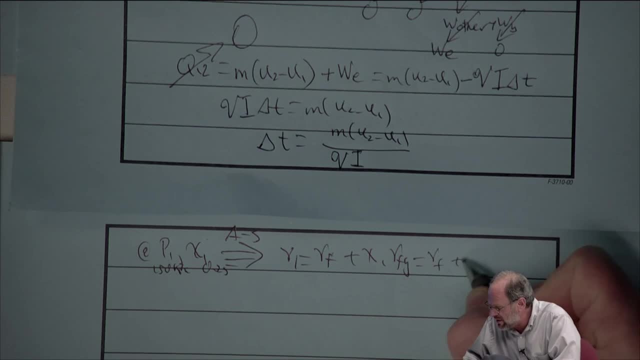 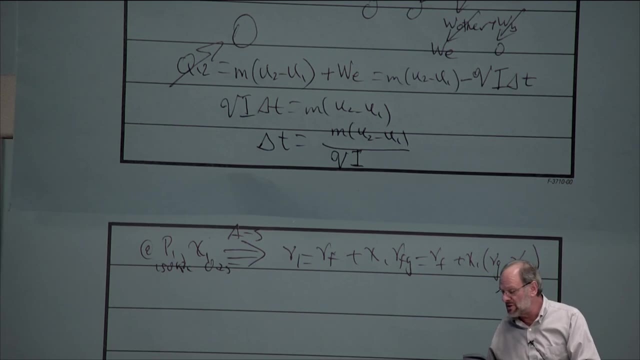 have a two-phase mixture. I will note once more that the author doesn't have a column of data called VFG, so we actually have to take the difference between VG and VF. So we just go into the book. The value of VF at 150 kilopascals is 0.1.. 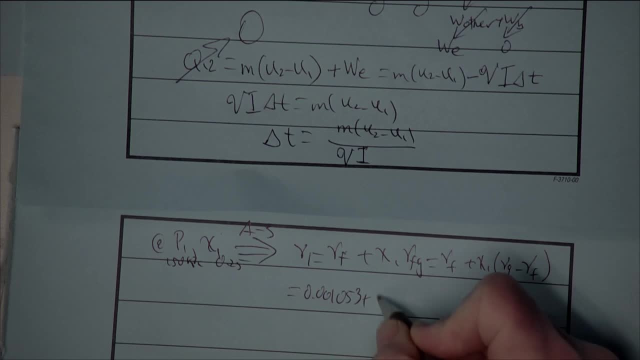 0.001053,. the quality is 25%, right, 75% liquid means 25% vapor, and then VFG is just VG minus VF. So VG is 1.1594, and then minus .001053.. 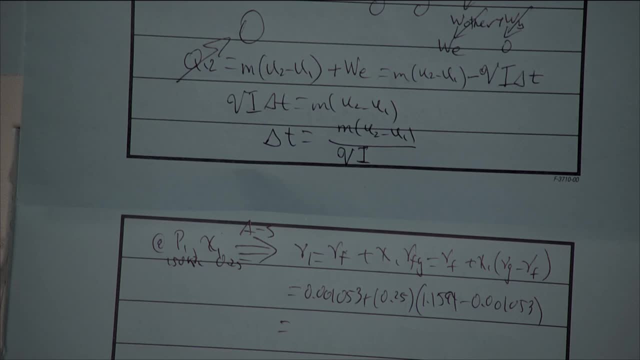 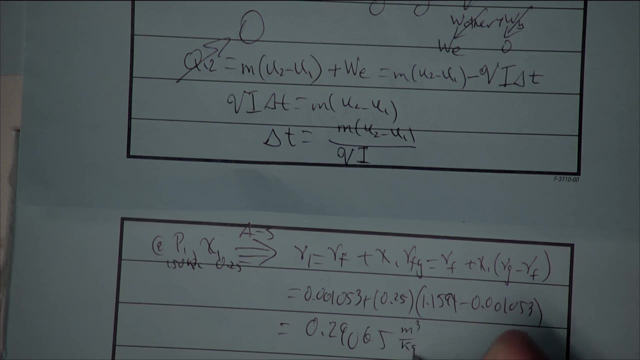 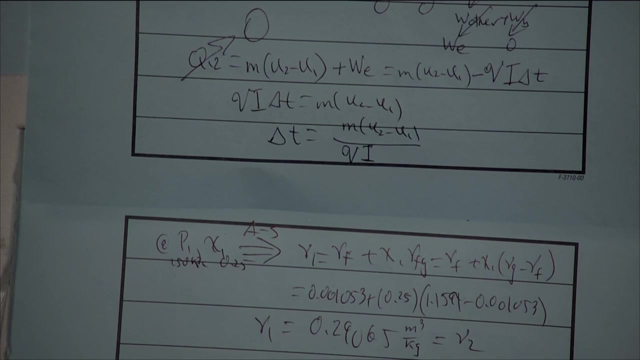 All the units here are the same. They're all in cubic meters per kilogram. So if we go through a little bit of math, we get .29065, cubic meters per kilogram. So there's my value: V1, which also equals V2, correct. 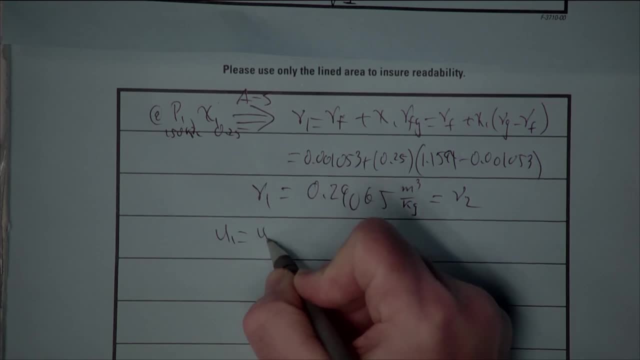 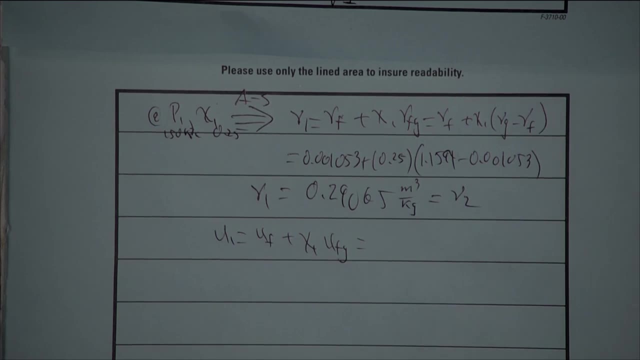 Now we do exactly the same thing for the internal energy. So U1 is UF plus the quality at 1 times UFG. So again, you can see, at 150, we're going to come over here, Here's UF And here's VF. 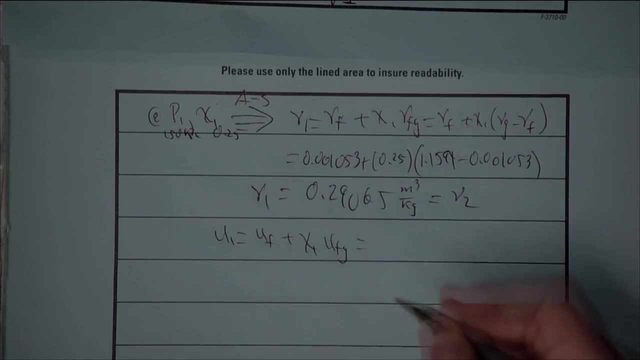 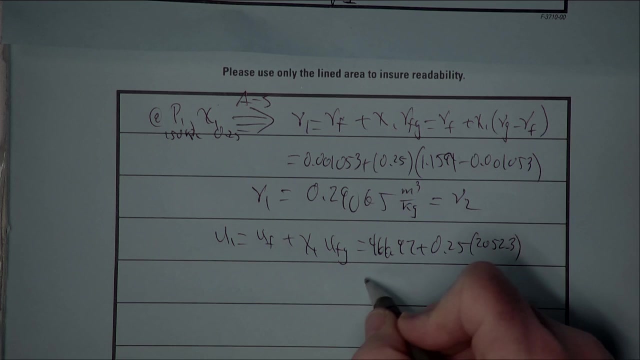 And here's VF And here's UFG. So UF is 466.97.. Quality is .25.. UFG is 2052.3.. All our units are kilojoules per kilogram. So again, we just go through a little mathematics. 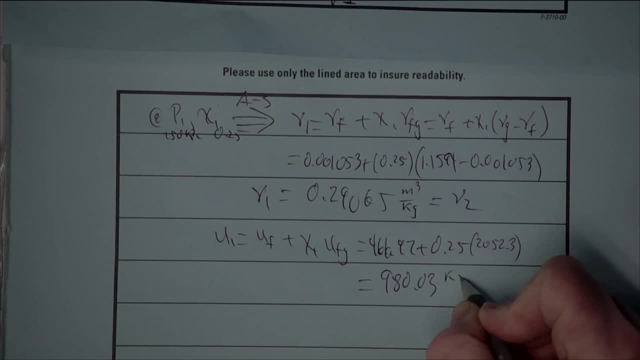 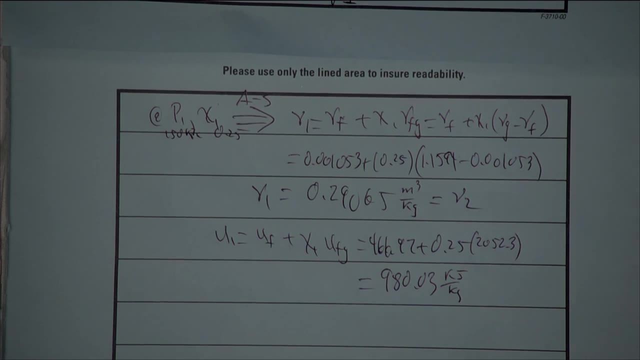 and we get 980.03 kilojoules per kilogram as the internal energy at .1.. All right, So now we're done. We're done with state .1.. Now we need to move on to state .2.. Now we know that it's a saturated vapor. 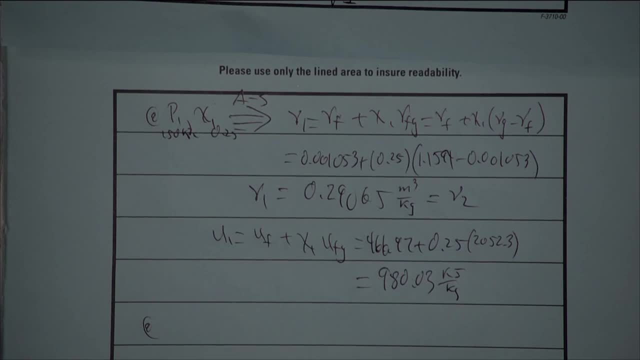 And we know that we have the quality as 100%, So we don't really have to think about quality. What's the other property we know at state .2? Well, it's the volume, right. So at V2, and for a saturated vapor, well, 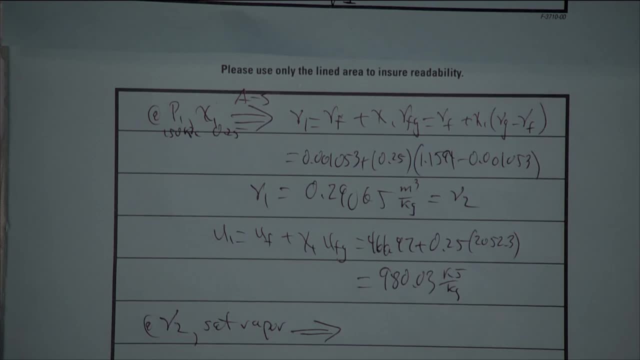 where do we go? Well, quite frankly, we could either use the pressure tables or the temperature tables. In other words, if you use A4 or A5, it doesn't matter. We know that we're a saturated vapor. So what we could do is just interpolate along the saturated 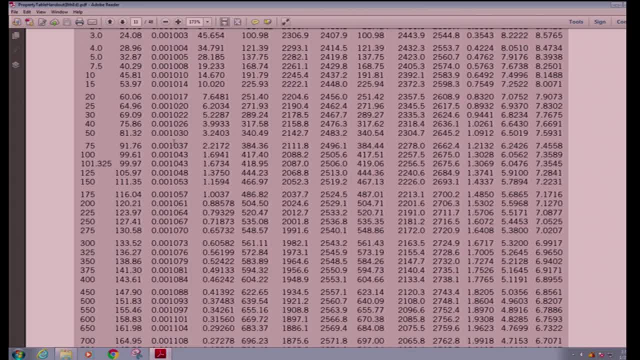 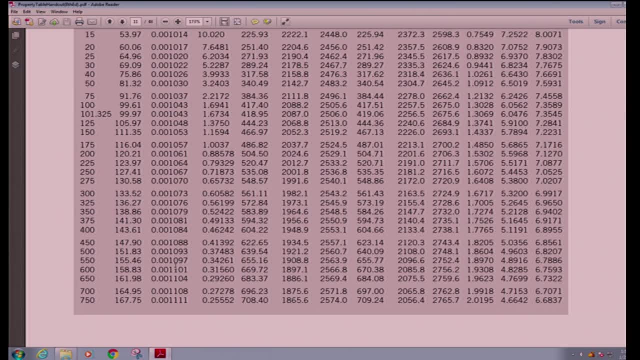 vapor conditions. okay, Why don't we just stick with A5, since we're in this particular table? My specific volume at state .2 is .2906.3.. And it's a saturated vapor. So let's see .2906.5,. that's going to put us right there. 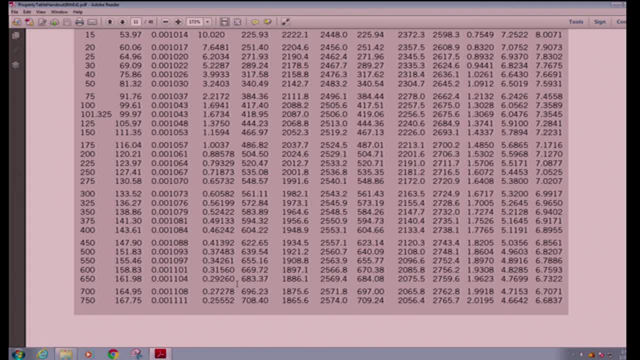 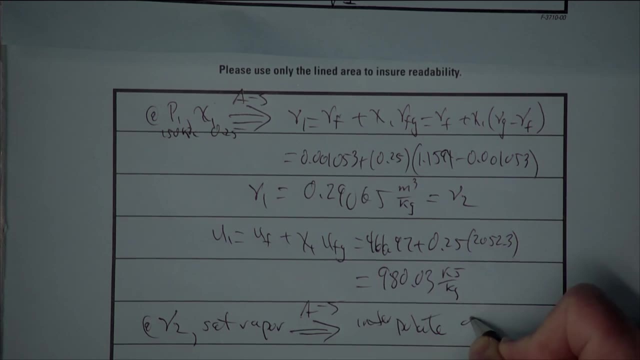 between 650 and 700 degrees right. Vg at 650 is .292.. Vg at 700 is .272.. I'm at .290, so I'm in between those values. So I go to table A5.. I interpolate on Vg. 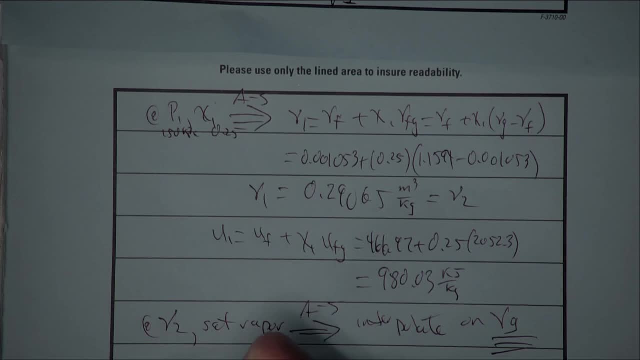 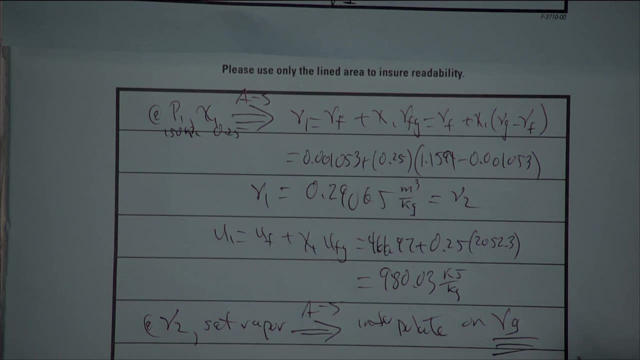 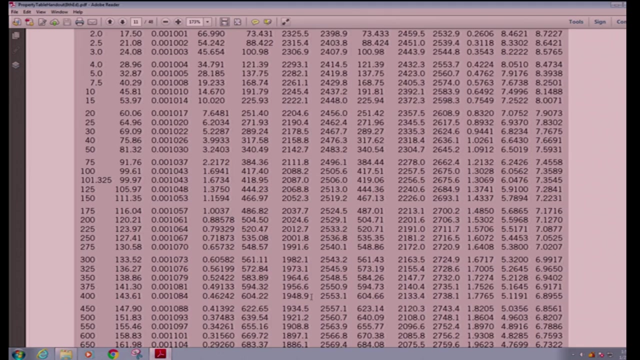 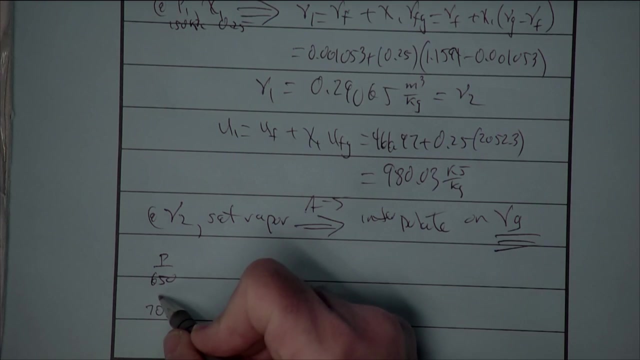 So let's just make a little sub-table, if you will, All right. so pressure: I'm going to be between 650 and 700.. Yep, Between 650 and 700.. My actual pressure, My actual pressure, is not really known. 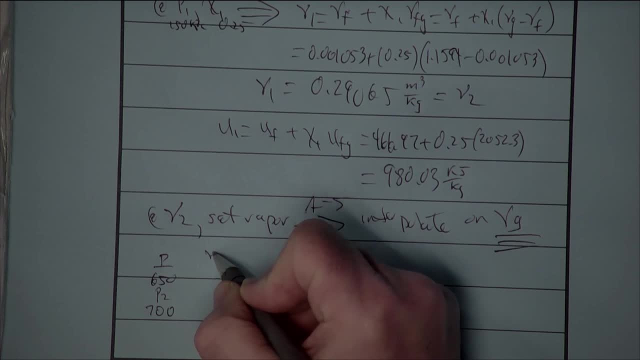 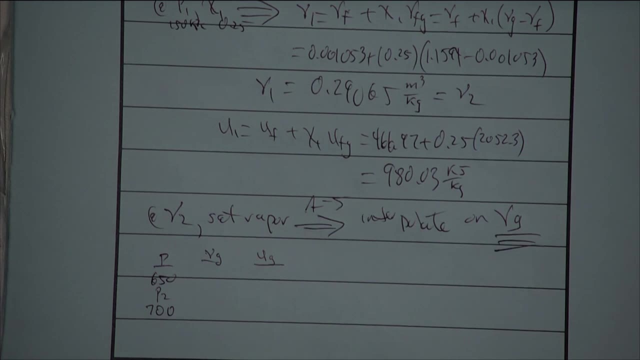 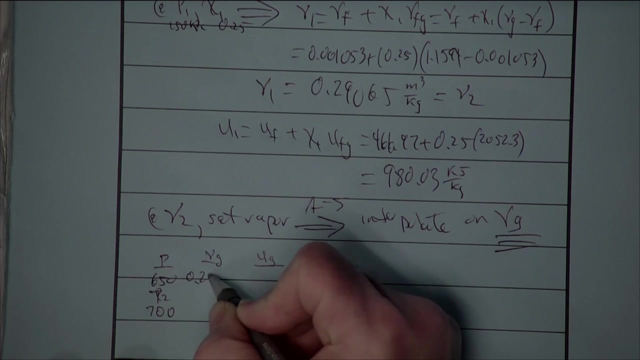 but it doesn't matter at this point And I need both specific volume and eventually I'm going to need internal energy data And this is all saturated vapor data. So at 650, Vg is .29260.. So .29260.. 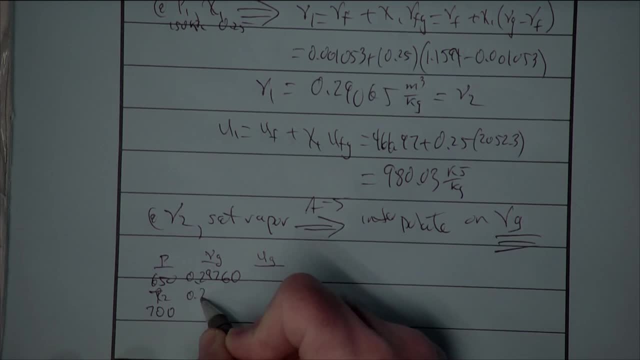 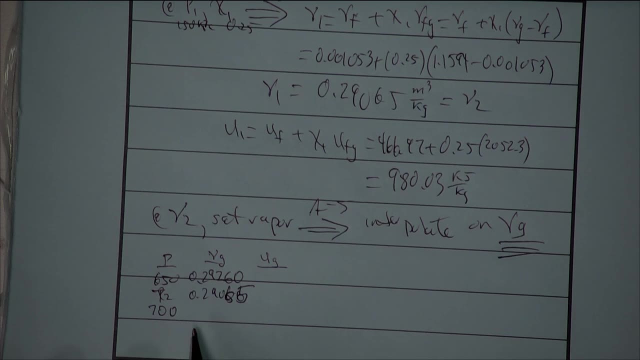 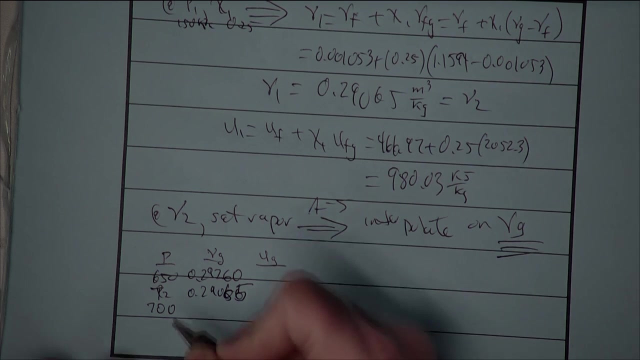 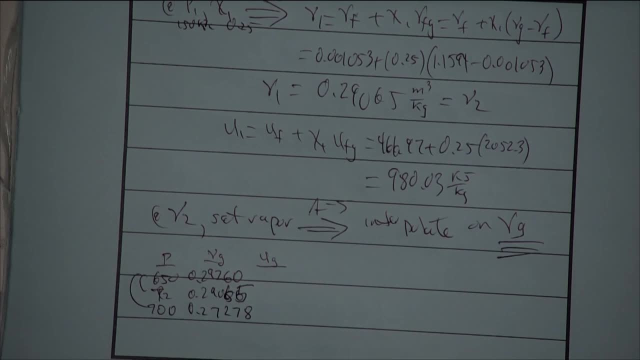 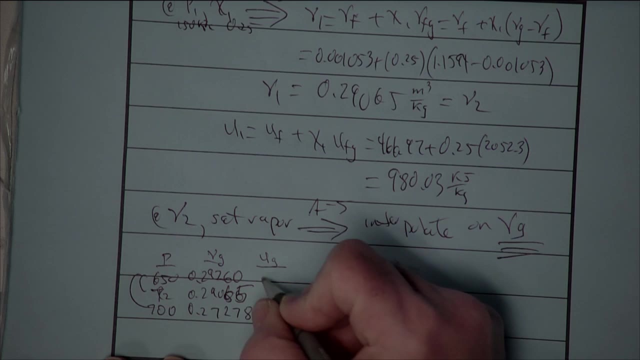 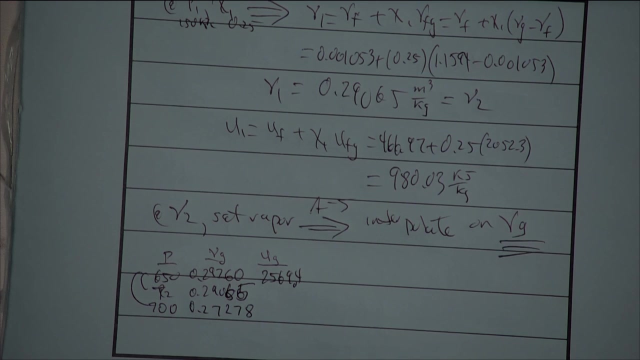 .27278.. All right, so I'm going to do an interpolation in here And then I'm going to do the same thing on the internal energy side. So I have 2569.4.. And that corresponds to 650.. So I'm over here. 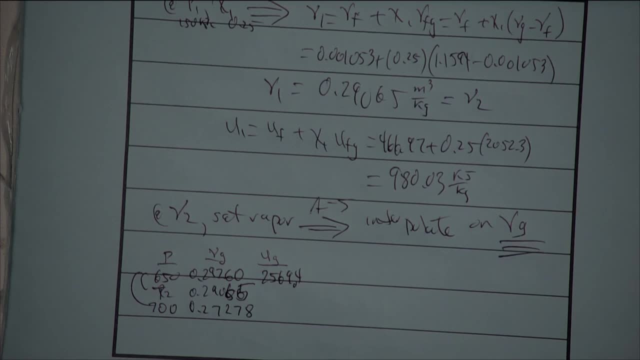 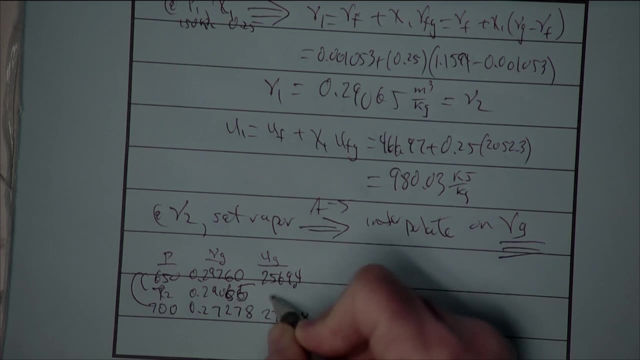 This is the Ug column. So yeah, 2569.4.. And then, corresponding to 700 is 2571.8.. All right, So I'm going to do an interpolation in here, And this is my unknown value of U2.. 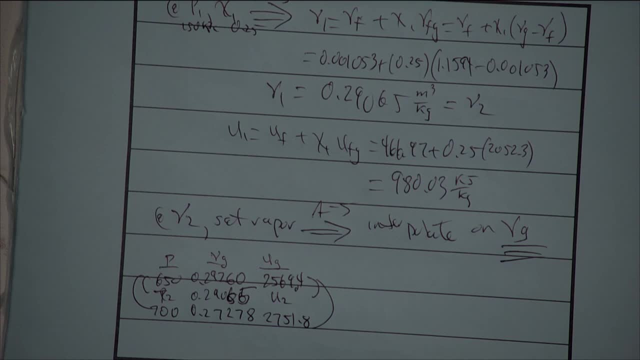 So I'll interpolate it here Now. I haven't actually been asked for the final temperature. I could do it pretty clearly. I can just do it from this particular interpolation, But I don't need it, so I'm not going to spend the time on it. 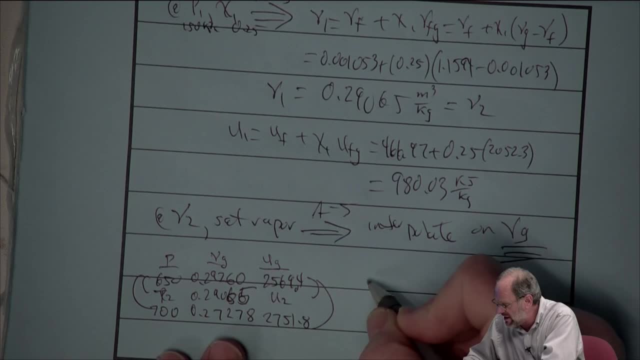 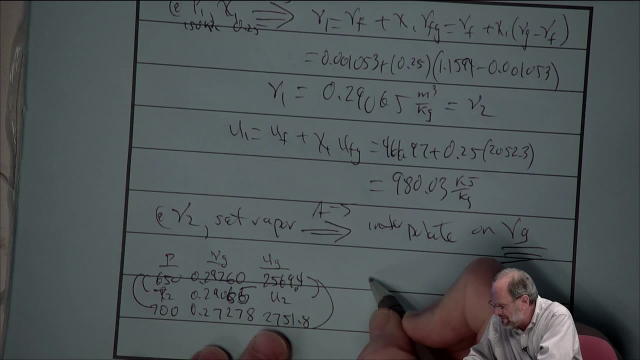 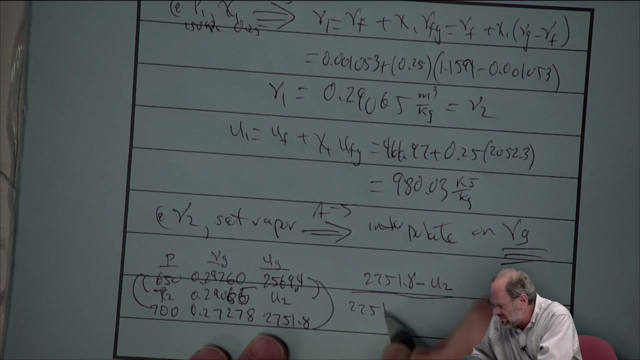 I'm just going to look at the internal energy. So we have the internal energy and I'll relate that to the specific volume. So let's see: Corresponding to 700, I have 27.7.. So 2751.8 minus U2, and then over 2751.8 minus 2569.4.. 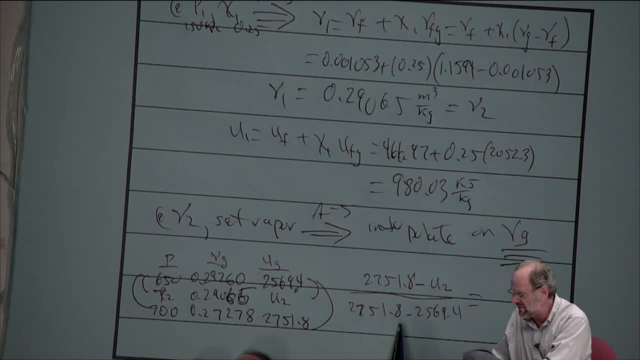 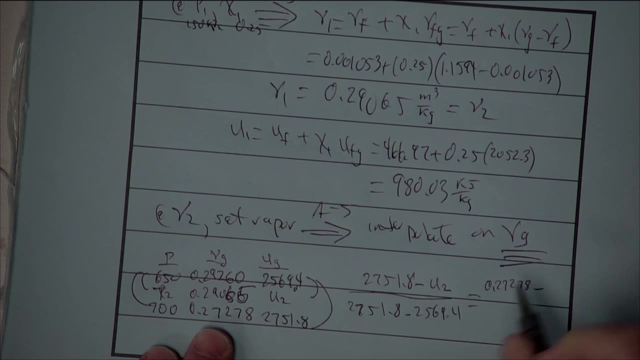 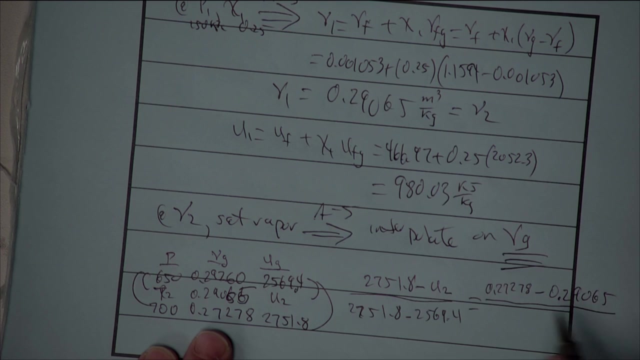 And then this equals the similar ratio of the differences of specific volume. So that corresponding to 700 is 0.27278.. That corresponding to my internal energy- 0.2, is 0.29065.. And then we divide it by the total. 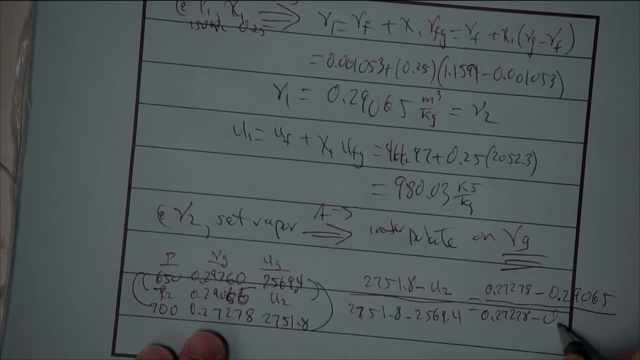 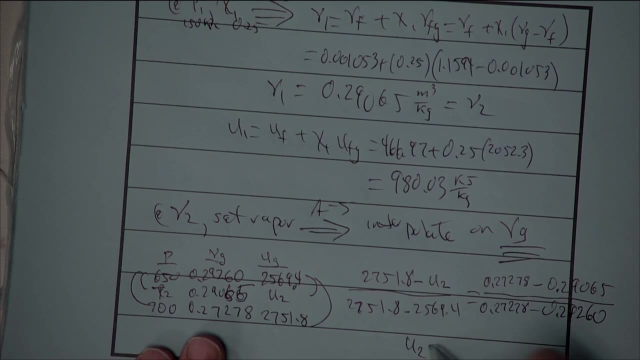 So 0.27278 minus 0.29260.. And you can see then that we just solved for the internal energy at state 0.2. And we'll get 2569.7.. And all these units are the same. 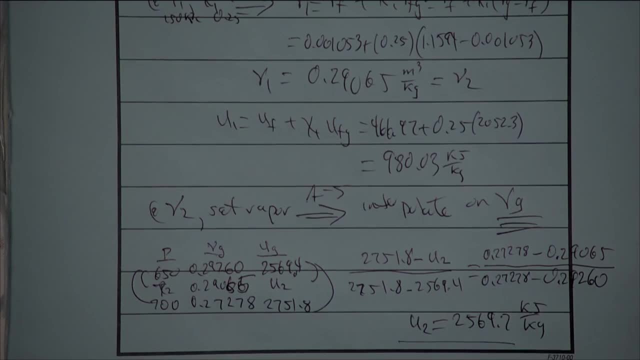 They're all in kilojoules per kilo. Okay, So now I have the specific internal energy at state 0.2.. So all I've done is I've interpolated along the saturated vapor line. all right, I interpolate between the entry at 650 and the one at 700. 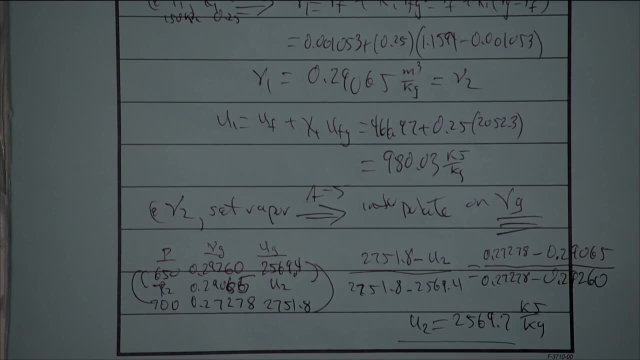 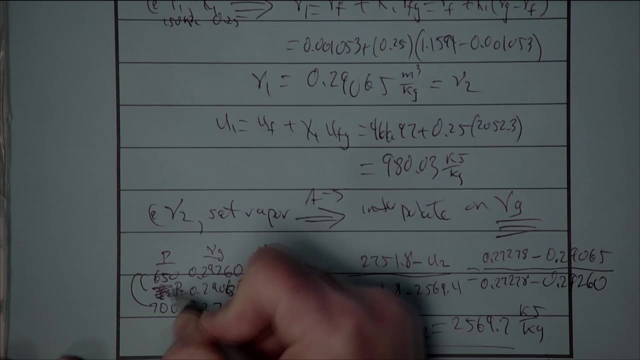 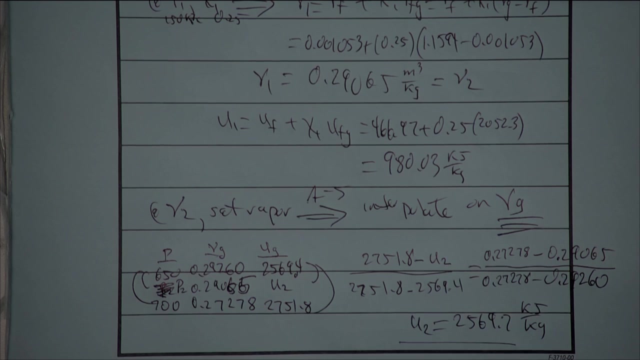 And, by the way, I put T2 there. That's not T2.. That's P2, right? This should say P2.. Sorry about that. Okay, Nonetheless, there's my answer. One thing that you can do is you can also note: 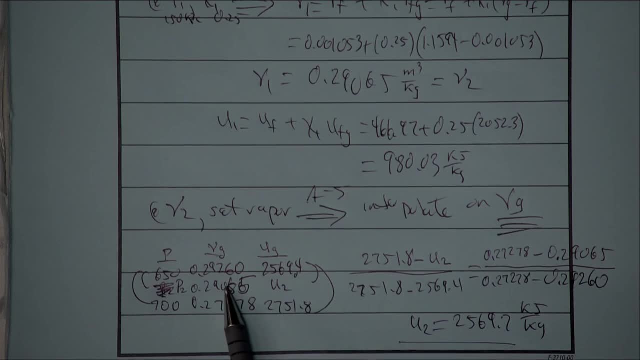 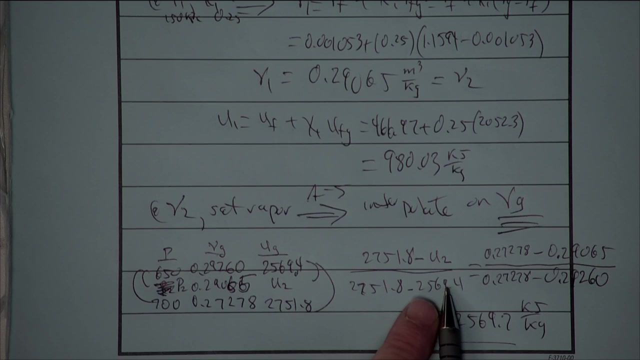 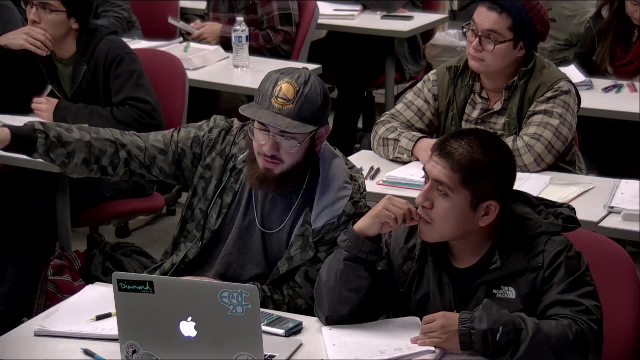 that my value of specific volume. it's kind of hard to tell. you know how close it is. Did I write something down wrong here? Yeah, Yeah, there's something wrong with the internal energy here. For the 700 pressure, the UG is, you switched the 5 into 7.. 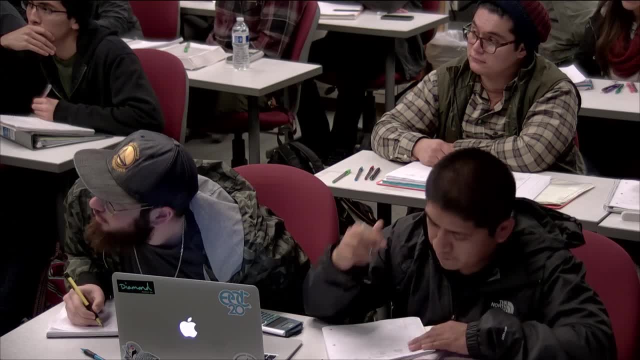 Oh, that's why it's wrong. It's this should be 25, not the 25.. Okay, Okay, Okay, Okay, 25, 7, 3, 2, 1.. Yeah, Okay, 25, 7, 3, 2, 1.. 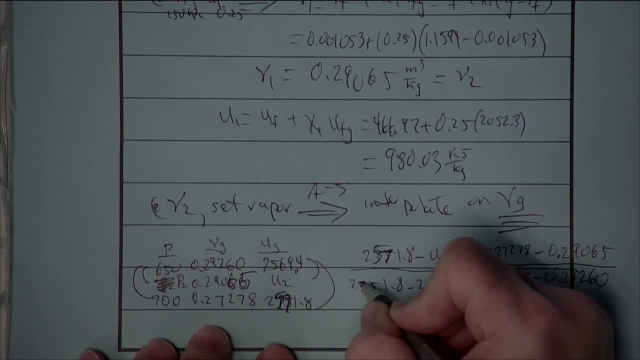 And then this should say: 25, 7, 3,, 2, 1.. This should say: 25, 7, 3, 2, 1.. Yeah, 25, 7, 3, 2, 1.. 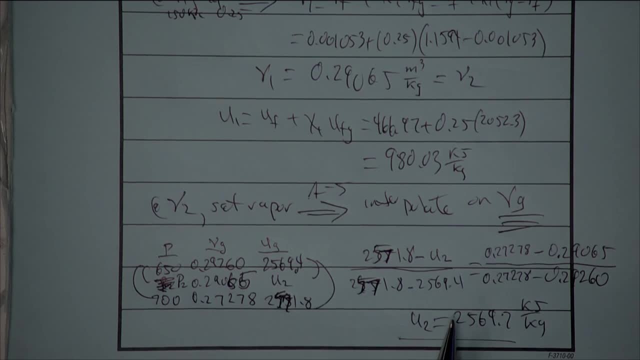 Okay. So I mean, I've prepared this problem and I've reviewed it several times and I'm still making stupid mistakes. Imagine how you guys are going to do when you solve your homework right. Remember what I said last week: that I think it's very difficult. 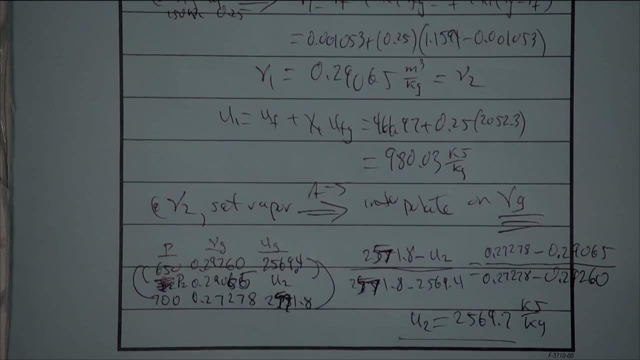 to get a final answer That's exactly correct. There's so many easy ways to make mathematical errors, So that's why I'm not so concerned with the math, I'm making math errors. You're allowed to make math errors, Just don't make too many of them. 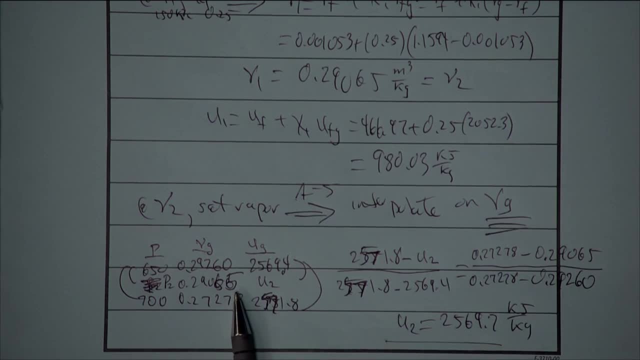 Anyway, now that we've corrected the numbers here, you can see that my value of 0.29065 is really a lot closer to 0.292 than it is to 0.272. And therefore I should get an internal energy. that's a lot. 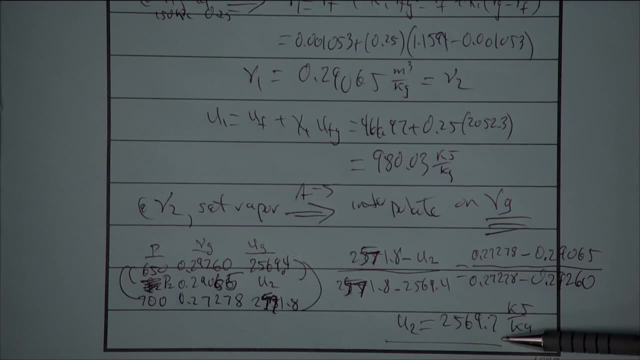 closer to 2569.4, and that's what I have: 2569.7.. So you know, if you go through the mathematics and you see that your numbers just don't look quite right, which clearly they weren't, but now we fixed that. 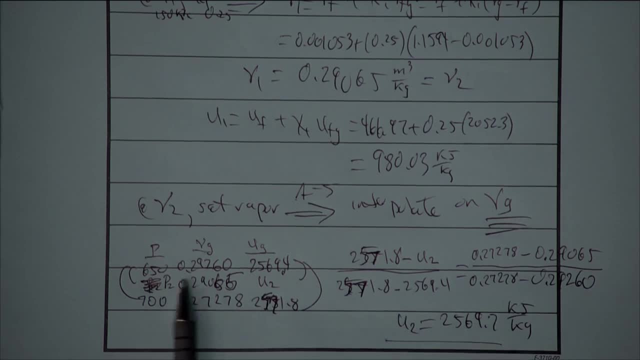 then find your mathematical error. I mean, I recognize that I made an error. I didn't know exactly what it was right up front, But nonetheless, we now have a value of U2, and we're ready to finish the problem now. 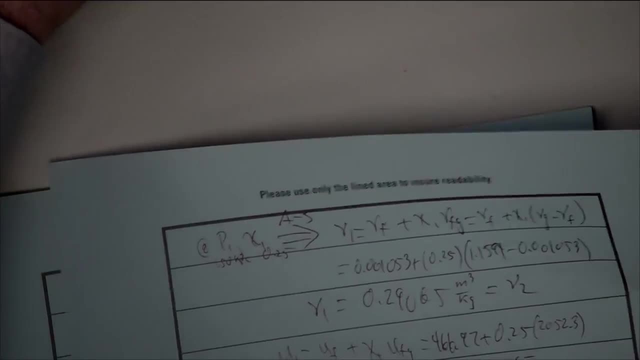 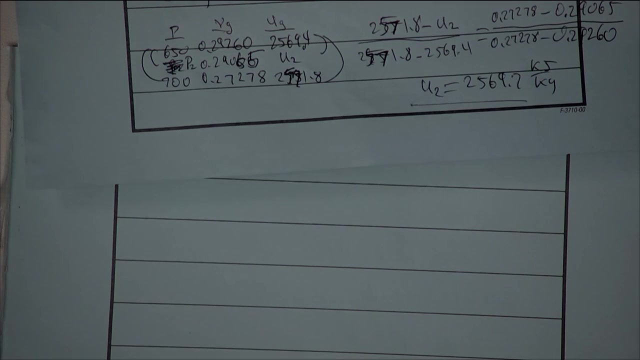 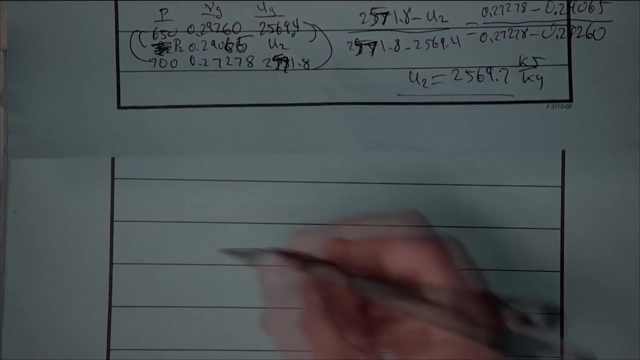 So we have everything. Now it's just a matter of going back to our So, back to our general equation. we have the mass, We have our internal energy data, We have the voltage and the current. Let's solve for time. 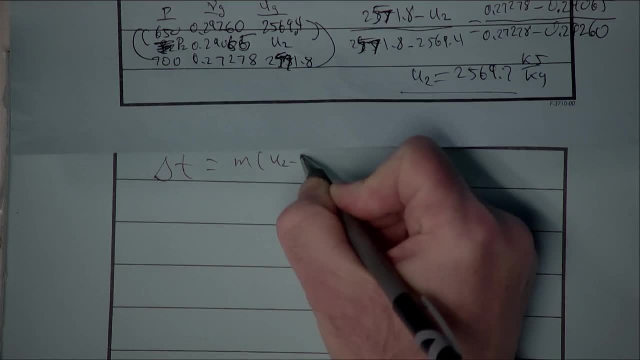 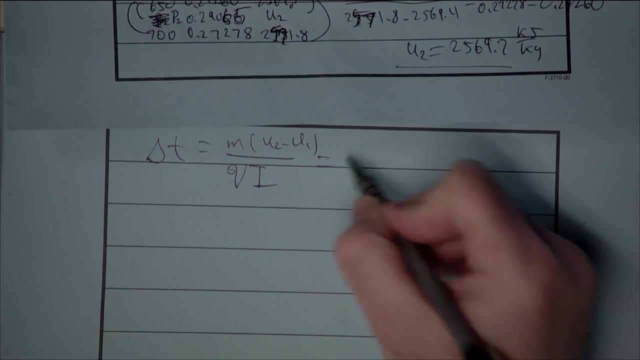 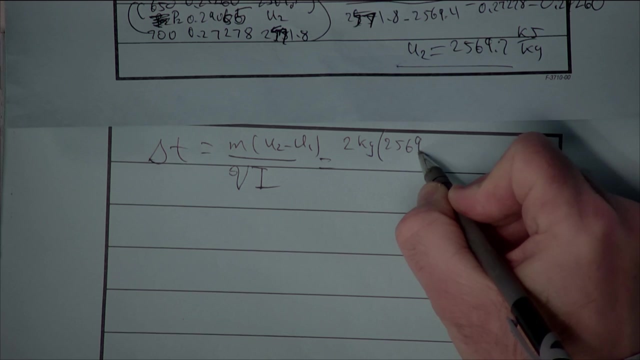 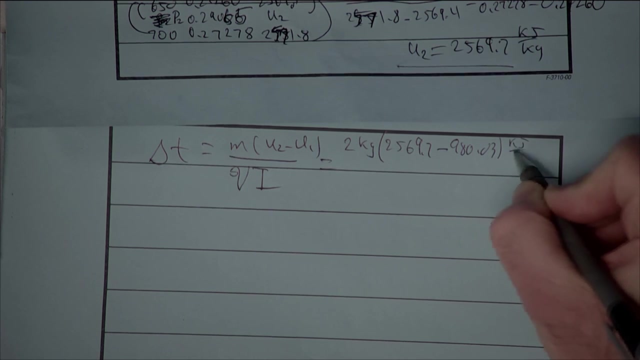 So back to the general equation. This was derived just a moment ago, So this is the equation we're trying to solve. for Let's just plug in the numbers. So we have 2 kilograms as the mass, 2569.7 minus 980.03 kilojoules per kilogram. 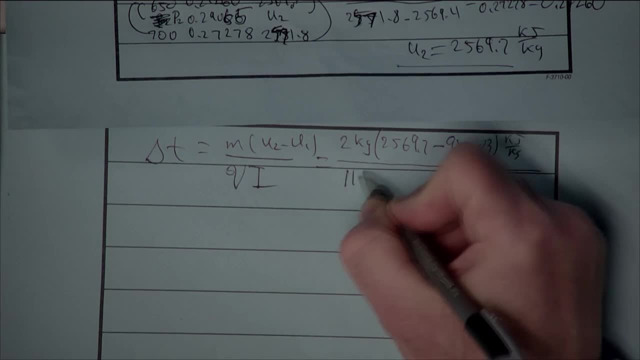 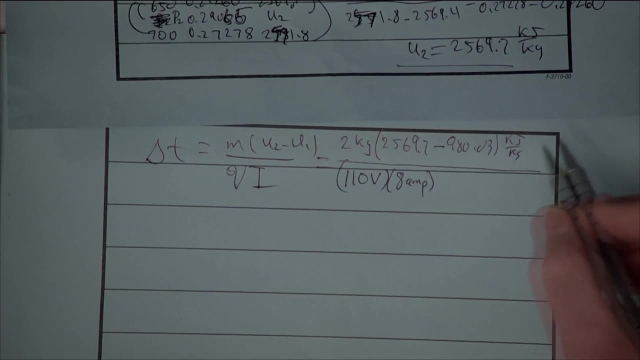 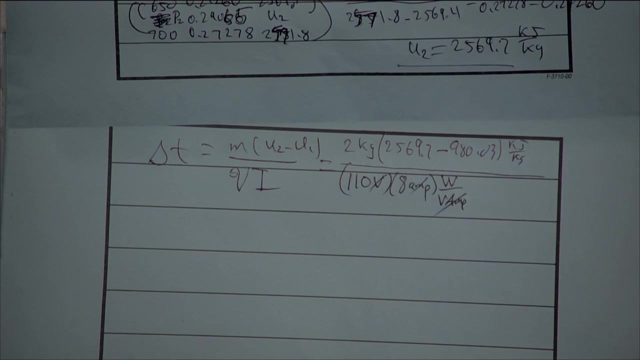 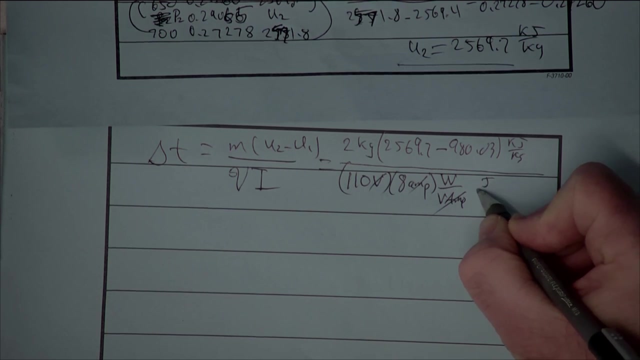 And now in the denominator we have our voltage, So we have 110 volts. And then the current 8 amps, And 1 watt is the same as a volt amp, So the units are watts, And then we know that a watt is the same thing. 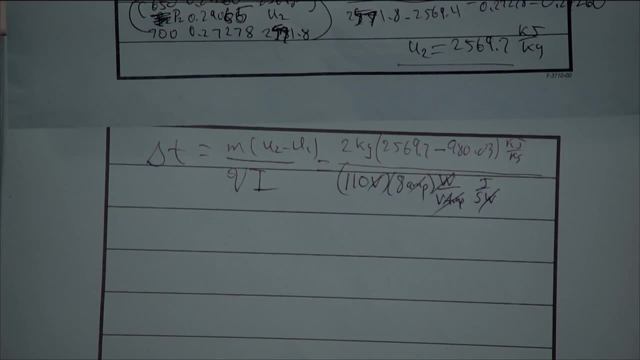 as a joule per second. So as long as our delta T is in seconds, then I should be okay. Well, almost okay, I'm off by 1,000 somewhere. right, I've got kilojoules in the numerator. 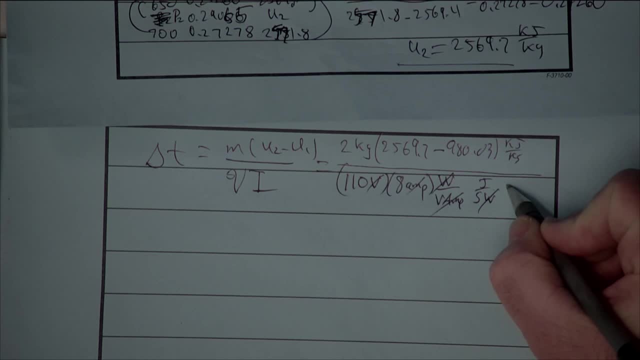 but joules in the denominator. So at some point you're going to have to fix that. So why don't we just throw in 10 to the minus 3 kilojoules per joule into the denominator. Right, I could have put 1,000 joules per kilojoule. 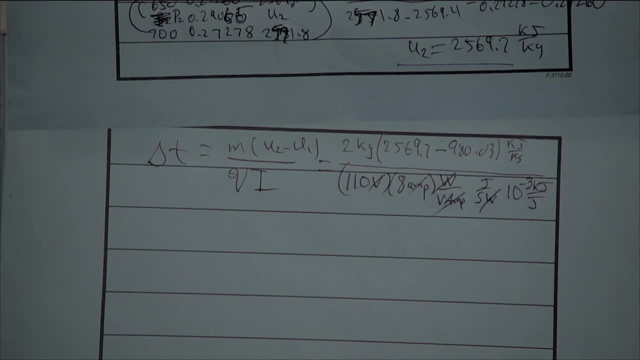 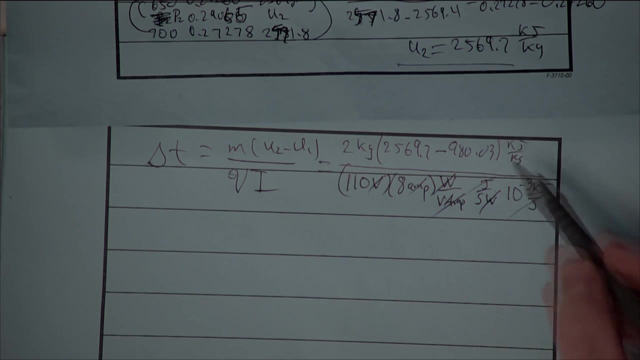 in the numerator, or 10 to the minus 3rd joule kilojoules per joule in the denominator. But nonetheless you could see then that now the joule units cancel, Kilojoules cancels, kilograms cancels. 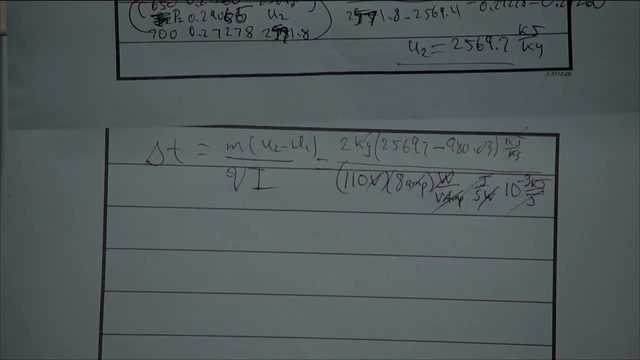 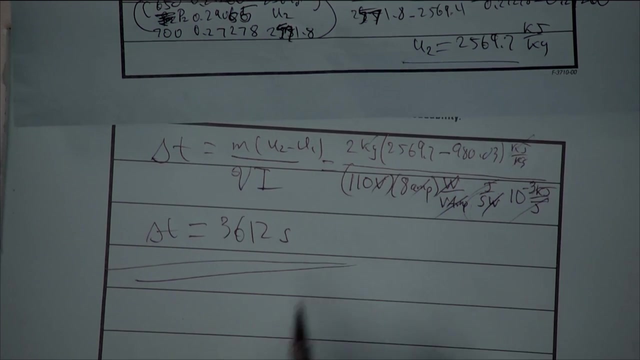 So the only units I have left are seconds, which are in the denominator Of the denominator, meaning that they're in the numerator, And if we go through all this mathematics we end up with 3,612 seconds. So it takes what. 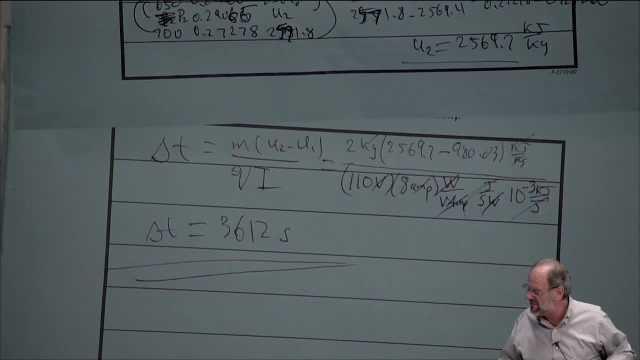 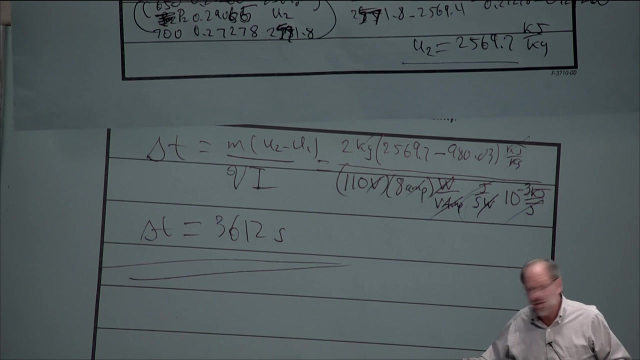 Just over an hour to provide the appropriate amount of electrical resistance work to turn a two-phase mixture into saturated vapor. And there you have that problem. So are there any questions? Any questions on this particular problem? Let me make another comment. It's very common in problems like this to not be given the mass. 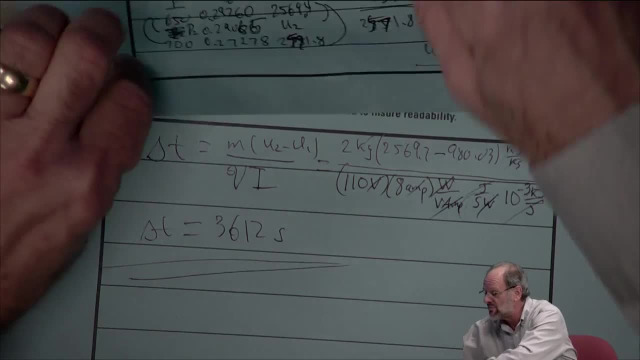 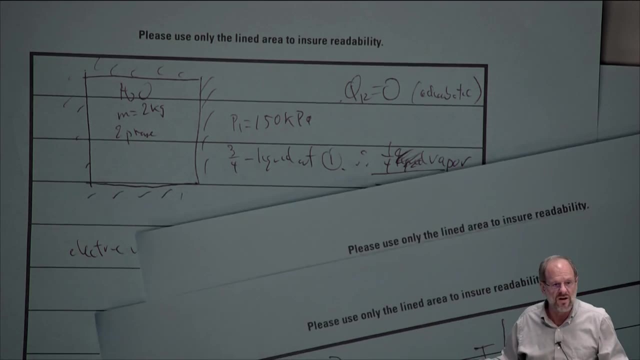 but to be given the volume instead. Like: what if we had this problem? and instead of being told that the mass was 2 kilograms, what if you're told that the total volume was, I don't know, a half of a cubic meter? 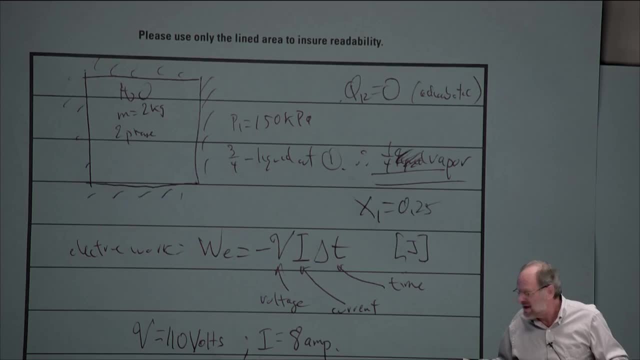 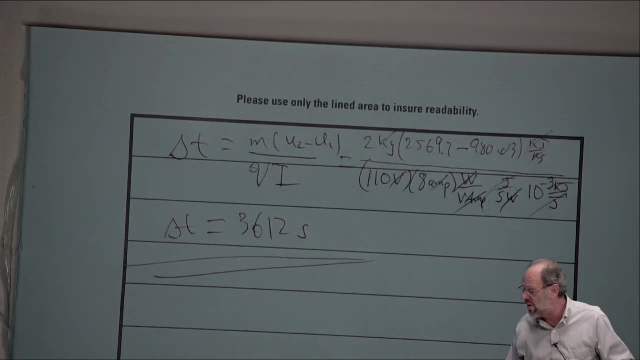 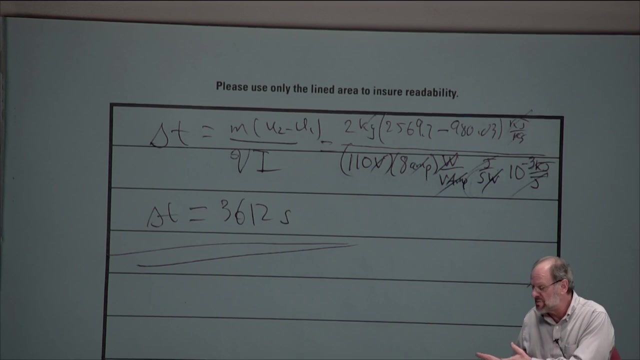 Would that change the problem in any meaningful way? Not really. So if you're given the total volume, yet you still know the initial pressure and the initial quality, can't you just use that pressure and quality to find the specific volume and then just divide the specific? 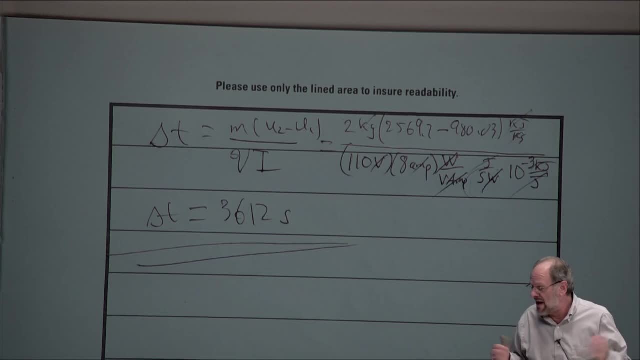 volume into the total volume to get the mass. So yeah, these problems sometimes are a little bit different than as I've shown them here, but similar right. So again very common to not be given the mass but to be given volume data, and then you would have to back. 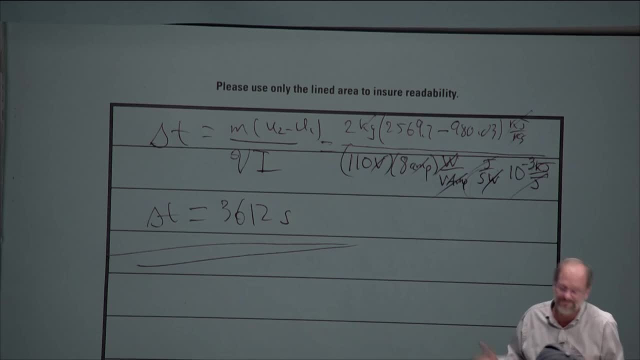 out of it the following way: So again, you would have to divide the mass, for you know solution to this particular problem. So again, just something for you to think about. So again, any questions Here. A joule per second is the same thing as a watt. 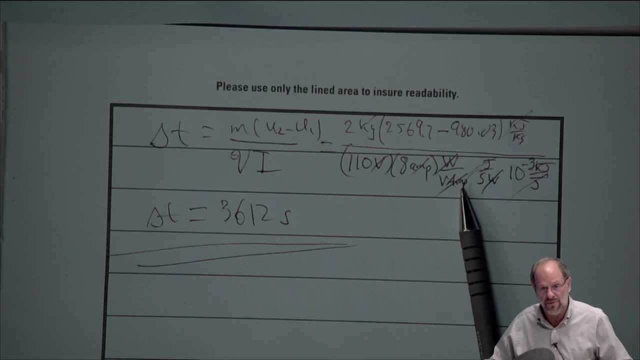 Yeah, So just by definition, a watt? well, a watt is a voltamp, but a watt is also a joule per second. So if we just note that a joule per second is the same as a watt, then you can see the all venous are going to cancel out. 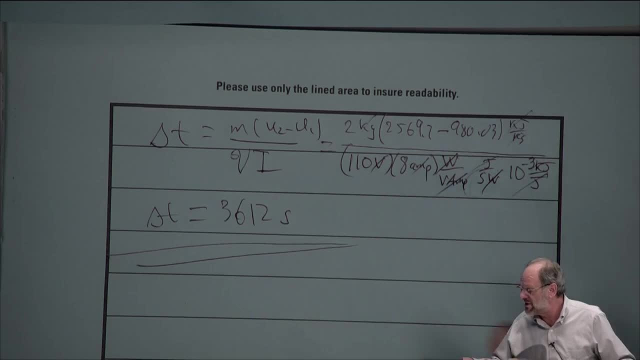 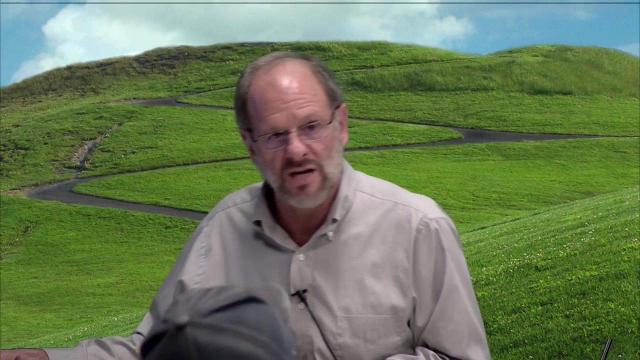 and we end up with a watt. So we end up with the time units that we need Again. look at these units. Make sure they make sense to you When you're solving a problem. always carry through the units in every problem and if the units come out right, 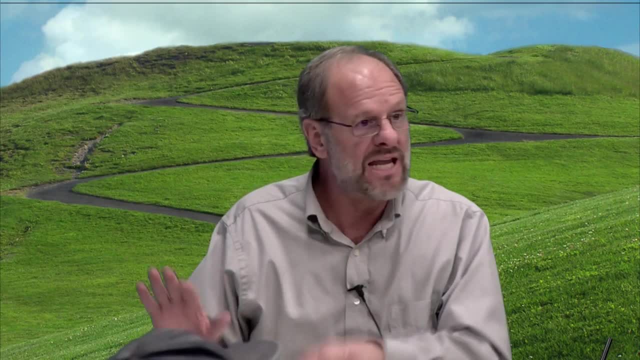 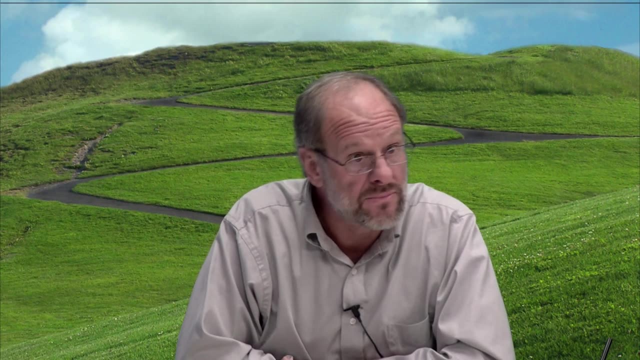 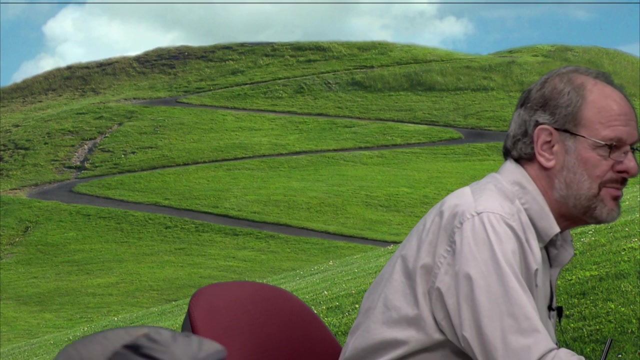 at the end there's a good chance. you did the problem correctly, All right, So again, any other questions? All right, So one more, all right. one more question first. Yeah, No, because in the booklet that I'm going to eventually give you. 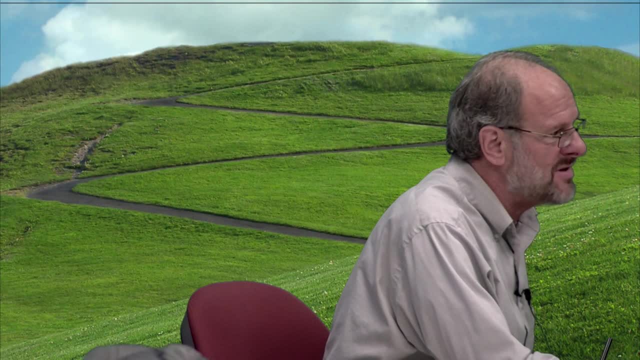 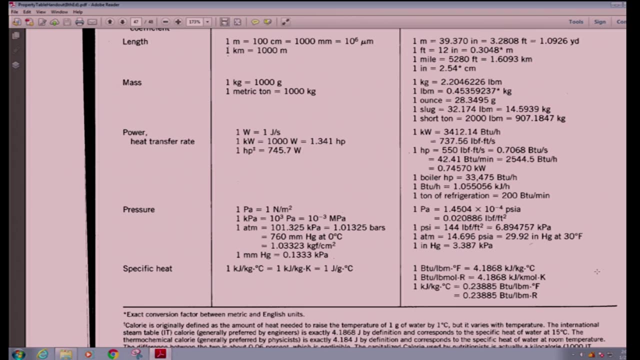 on all your whole- I'm sorry- on all your exams. you have this nice table of convergent factors. The whole inside back cover of your book are just all these convergent factors. So hopefully somewhere in here it'll tell you exactly what you need. 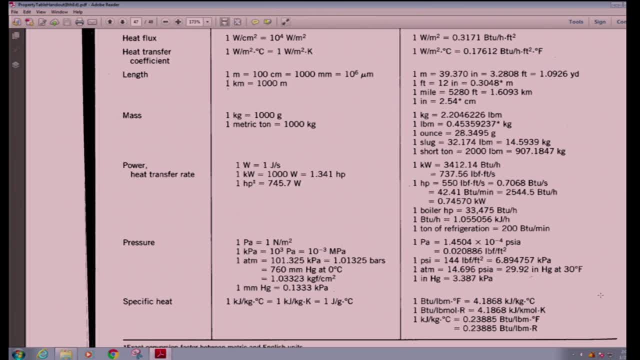 to know. as far as the conversions, If there's a conversion you need that is not in the table here, I will make sure you have it. I'll give it to you. on the. This is in our book, this page It's the inside back cover. 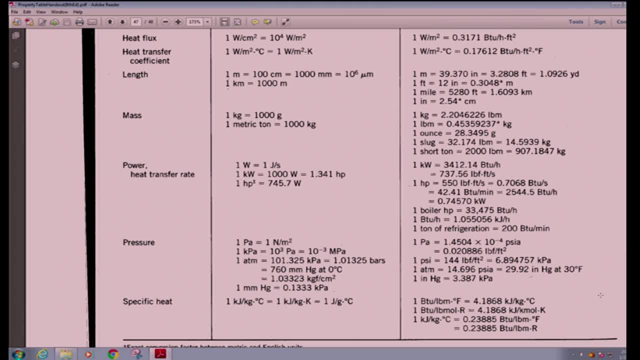 We have a hard cover, A hard cover copy of the book. It's in the inside. If you have the electronic version, it's somewhere in there. It's probably at the end, but I can't tell you exactly where it is. 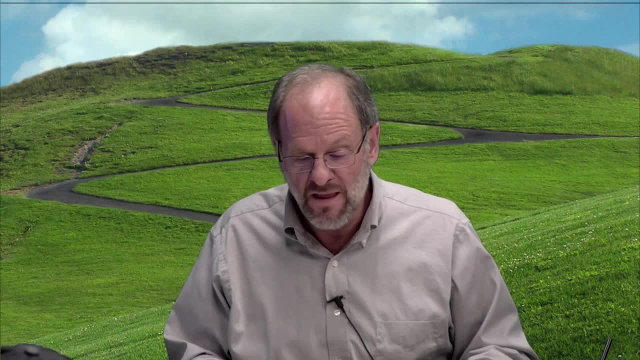 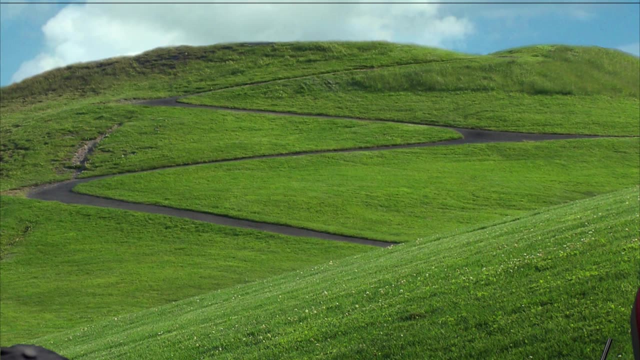 But it should be in there somewhere. Okay, Let's look at another example problem. I only have one minute, so there's no way I'm going to finish it, But I just want to at least get you thinking about what we're going. 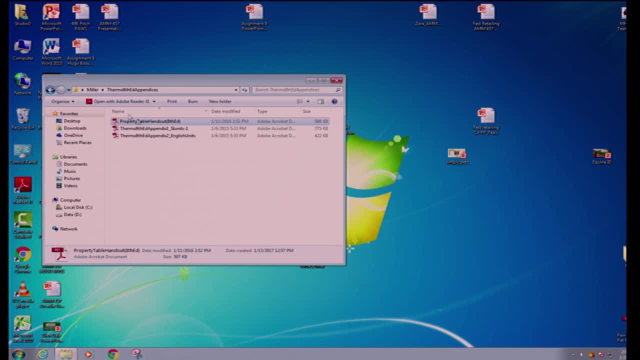 to start talking about next time, And this is actually Also from a previous edition of your book, but from the 6th edition, And let's see number 1,, 3,, 2, yeah, it's this one. 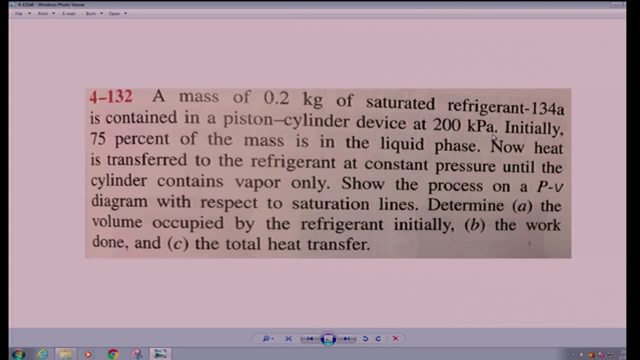 Okay, So this one is similar to the previous one. Let me just talk you through it, but next time I'll actually set it up. I just want to make sure that we can understand what this problem is. So, first of all, it should be noted that in this particular problem, we have a certain mass. 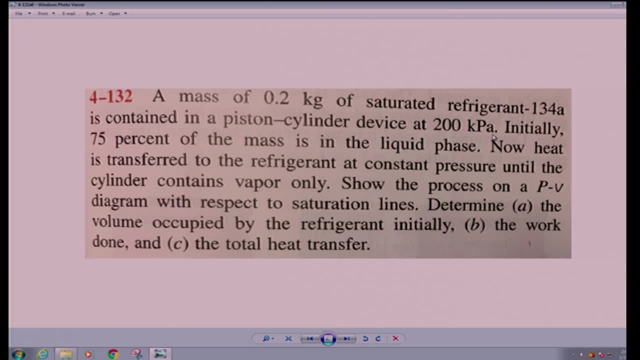 and it's in a piston-cylinder device at a certain pressure. So this is different, right? This is a piston-cylinder device, It's still a closed system, but it's not a constant volume system, So it's different than before. 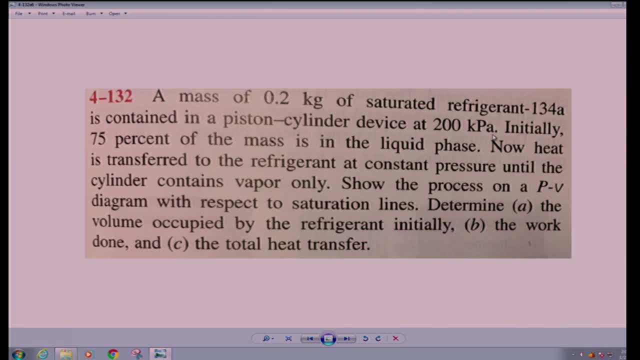 Piston-cylinder devices have the ability to change volume while maintaining a constant mass. So it says that we have .2 kilograms of this saturated refrigerant at a certain pressure. It says that initially, 75% of the mass is in the liquid phase. 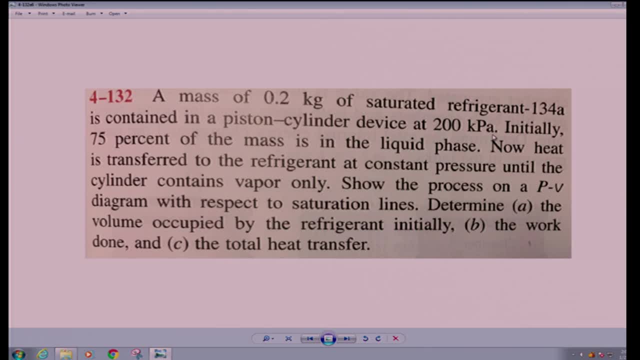 So the author did the same thing that he did in the previous one. In the previous example problem he should have just said the quality is 25%, but instead it gives you the mass fraction in the liquid phase. It says heat is now transferred at constant pressure. 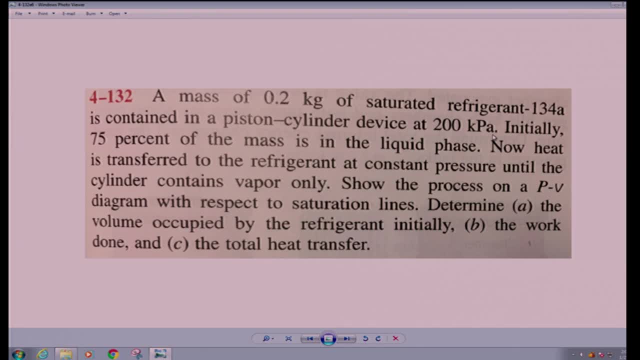 So really you can think of this as a frictionless vertical piston-cylinder device where the weight of that piston is always constant, So therefore it's maintaining a constant downward force through a constant area, so it's a constant pressure. 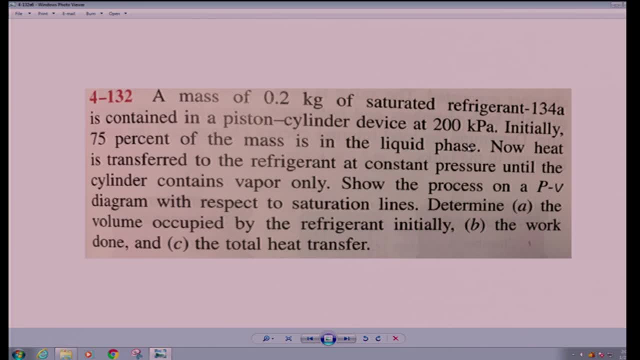 So the author could have just said that this is a frictionless, vertical piston-cylinder cylinder device. Instead, he chose to simply say it was a piston-cylinder device, but tell you that heat is transferred to constant pressure. It means exactly the same thing. 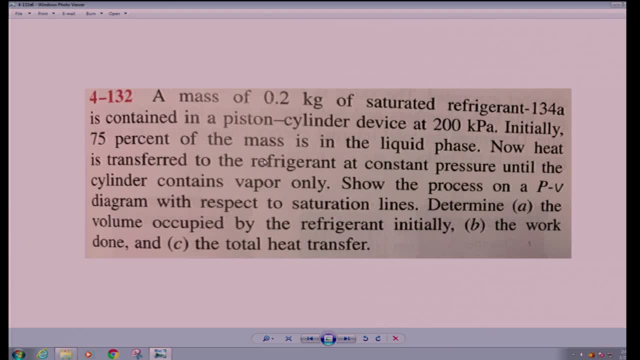 It's a constant pressure process And it's not well insulated, right? This has heat being added to it, So this is another difference. But it says that heat is added until the cylinder contains only a vapor. So that's kind of the same as the previous problem as well, right? 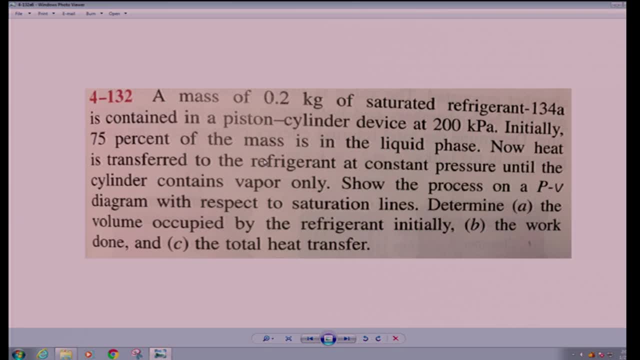 You start with a two-phase mixture with a 25% quality but unlike the previous problem, where you're adding work at constant volume in order to vaporize all the liquid, here you're adding heat at constant pressure in order to vaporize all the liquid. 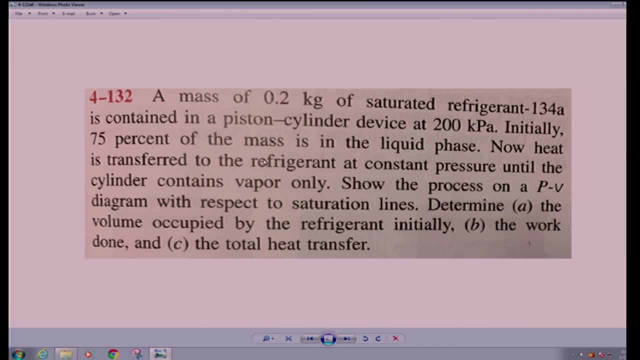 When you finally get to that point of the saturated vapor, the problem is done. You're asked to find the volume that the refrigerant occupies and the work done. Frankly, you don't even have to be asked to find the volume. The work is boundary work. 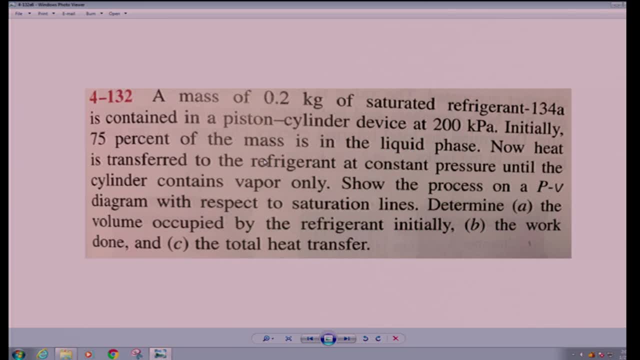 How do you find boundary work at constant pressure? but by finding the volume. Well, you have to find the volume, You have to find the pressure times, the change in the volume. So you need the volume. The author is kind of talking through this problem. 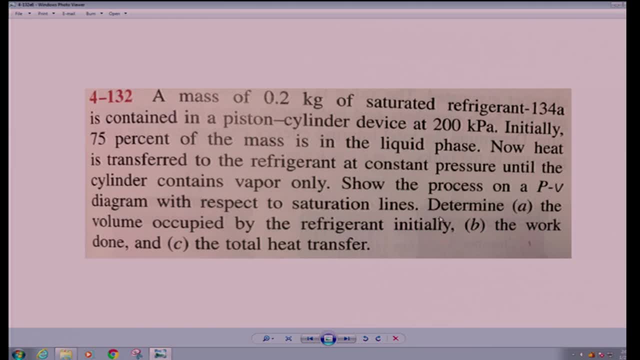 which is also kind of common. Nonetheless, you find the volume, You can find the work after you go through the process and then you can find the total heat transfer. So this problem is going to be very similar to the previous one, but not identical. 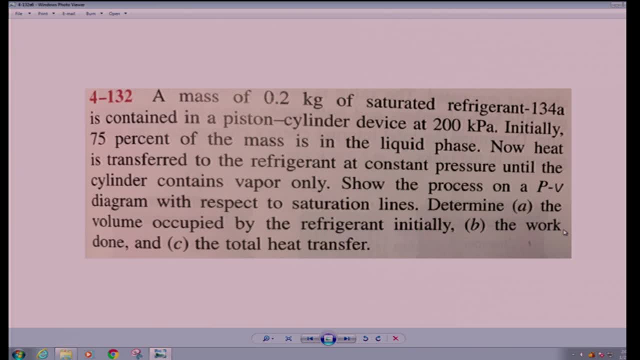 So that's all the time I have for today. I'll just leave this up here in case anybody wants to keep writing it down. You're welcome to think about the problem. The heat transfer, by the way, is 30.9 kilojoules. 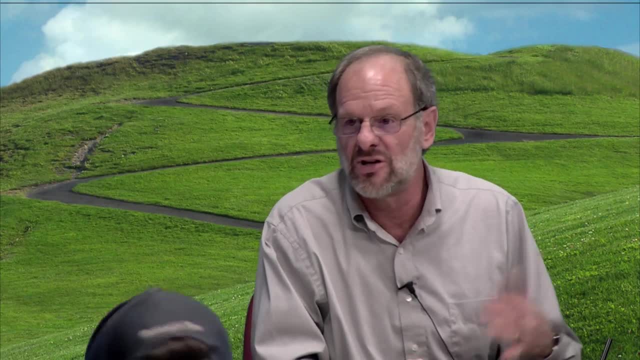 So if anybody wants to try to find the final answer, you can do so, But I'll go through this completely on Friday. All right, so that's all for today.